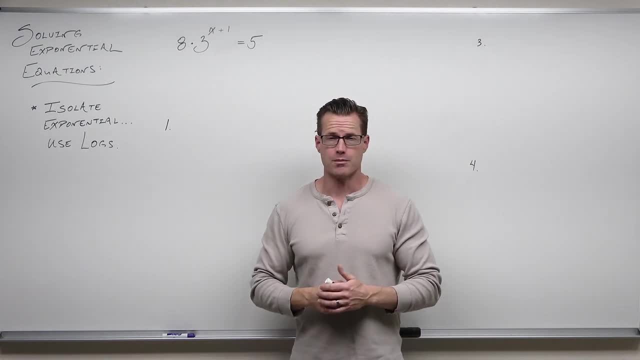 if you have an exponential equation, there's no way to find a common base like three and five. There's no way to change a five into a three or three and five into some lower base to set our exponents equal. So here's the idea. In solving any equation you need the inverse operation, or 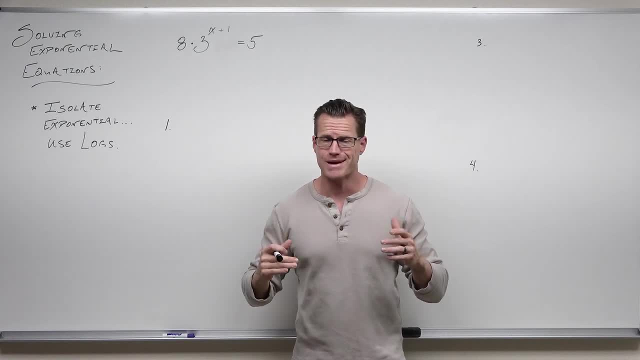 inverse function Because exponentials have an inverse and it's called a logarithm. it's going to take a logarithm to solve these exponentials. There are a few ways, like four ways, that I can show you how to do this. They're all equivalent. What that means is that your solution might look a little bit different. 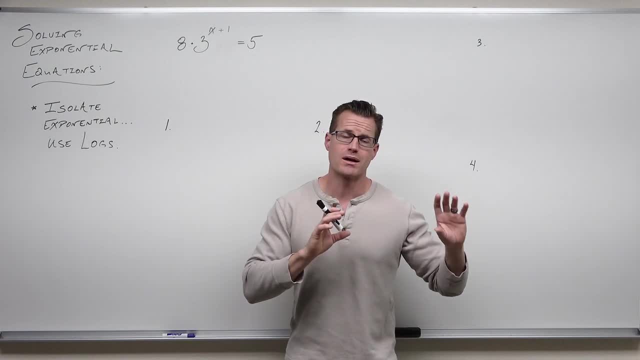 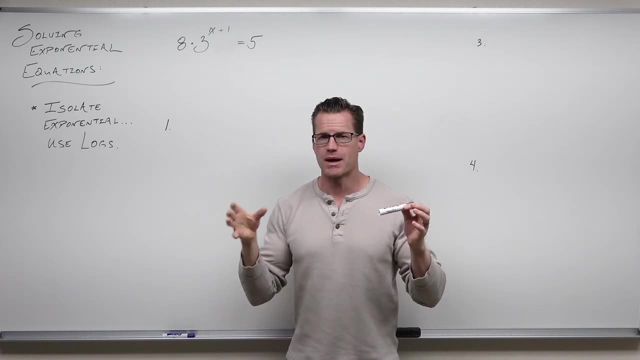 than like a textbook or someone else's considering the choice you make on how to solve this. When we get to not having just one exponential, we have two exponentials. that really pairs down what we can do and leads us into well, you have to take a logarithm on both sides And we're going. 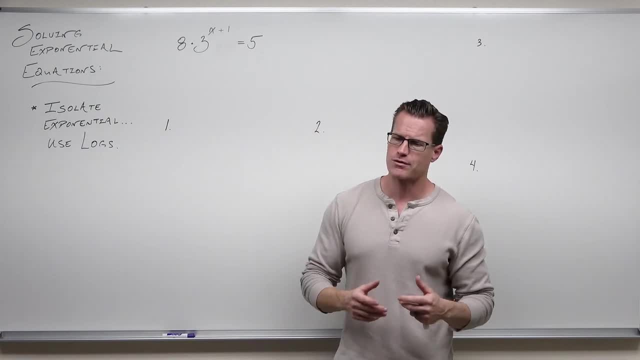 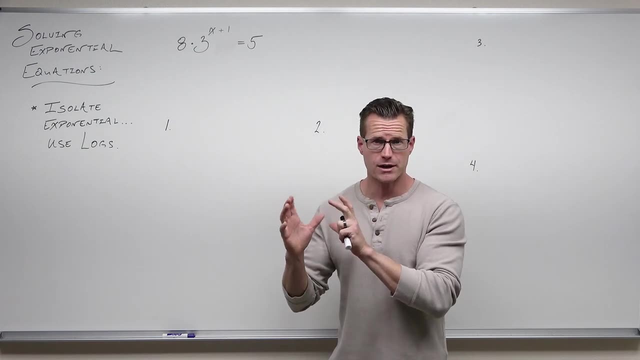 to see that, So we're going to jump right into it. Here's the idea on how you solve every exponential equation in general: If you can, one exponential on one side and a constant on the other. If you can't, that means that you'll have. 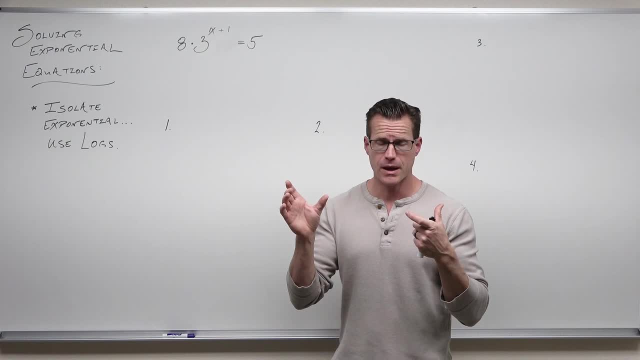 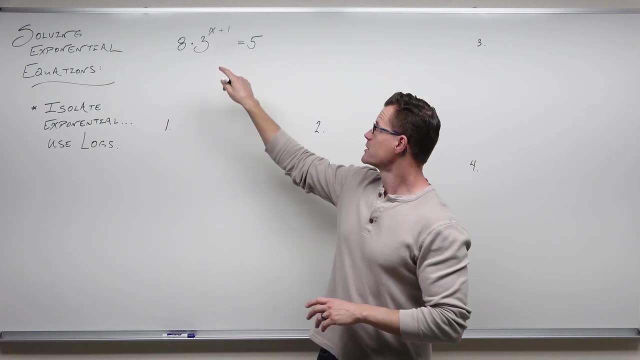 two exponentials. Pick one on one side and one on the other. Now, in either case, if you do not have common bases, you are going to have to use a logarithm, So we're going to do that right here. So this is what's called not isolated, When you have something added, subtracted or multiplied. 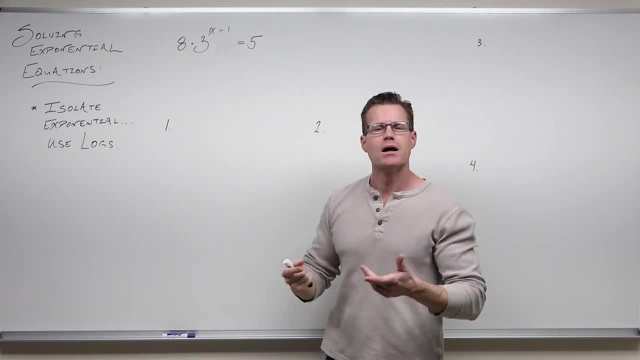 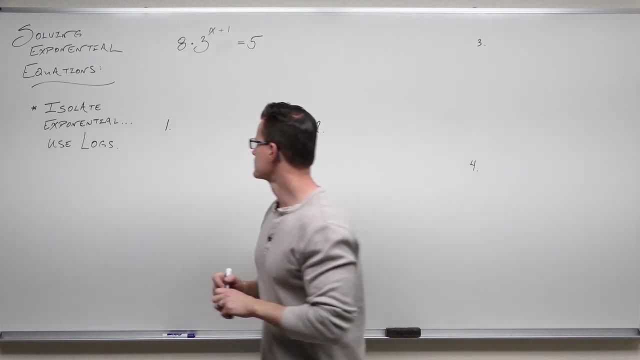 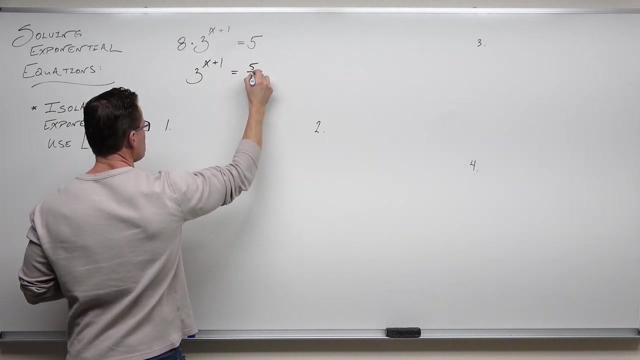 by your exponential, and that's on one side and a constant on the other. you have to remove the coefficient, or add or subtract to remove the constant. In this case we're going to divide both sides By eight. This is called isolated. as far as exponential is concerned, we're not really worried about the. 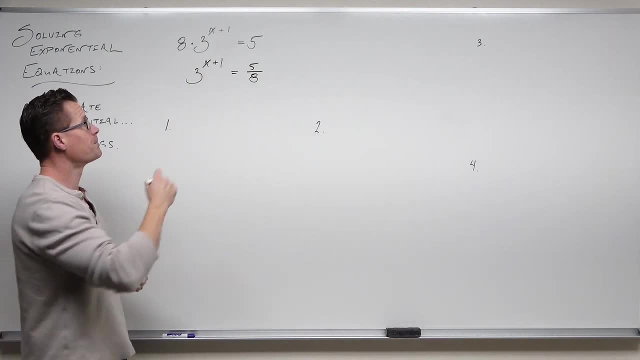 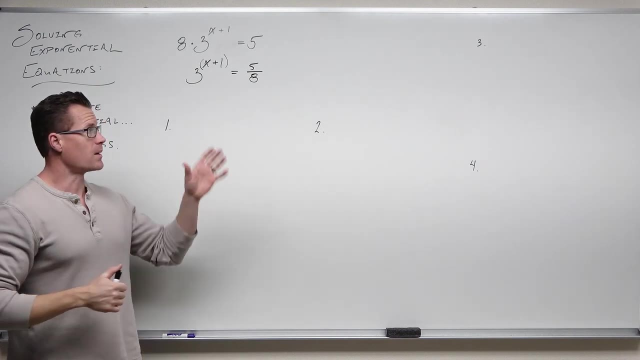 x plus one, because that is in the exponent and it would help if we put some parentheses around that to show this is the exponent. Now, here's what's going to have to happen. We're going to have to choose, on a basic exponential equation, One of four ways to solve this. We can either go directly. 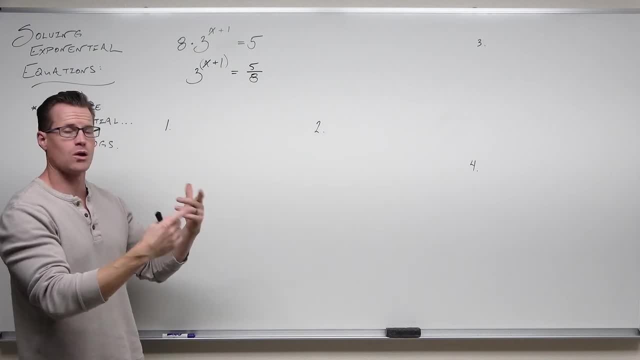 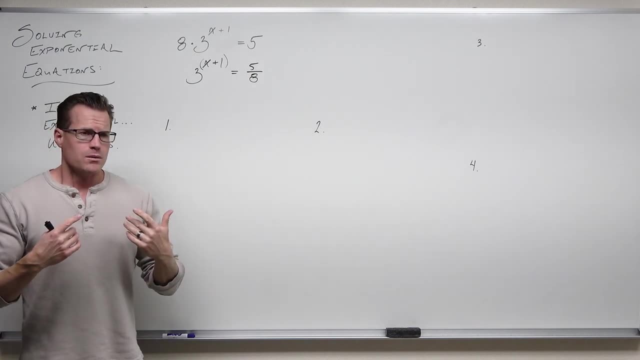 to a logarithm using logarithmic notation, or we can use a log on both sides in one of three different bases. I'm going to show you all of those things right now. So here's your options. I'm going to say this a couple more times, but please remember, if you have two exponentials. 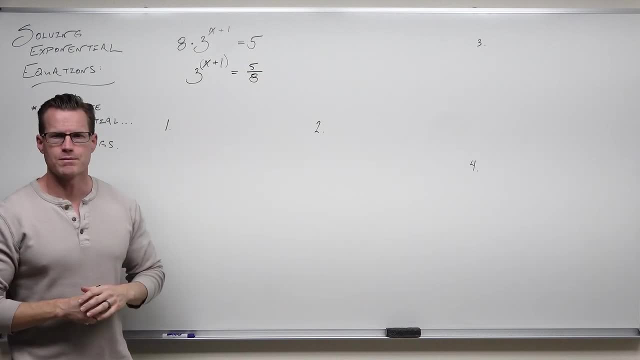 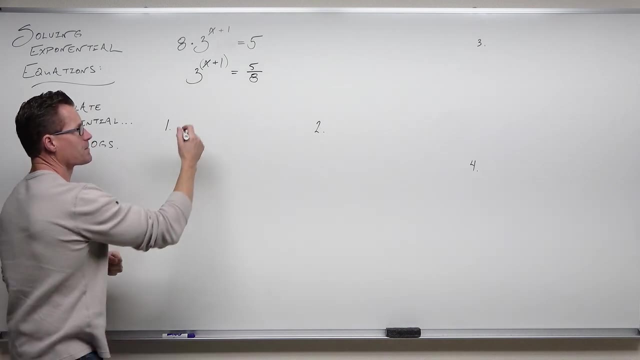 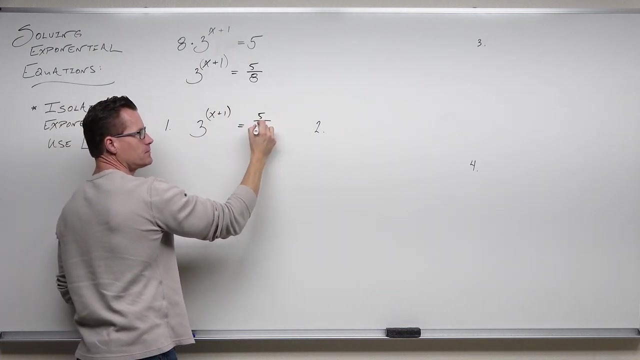 like legit exponentials of variables. this first way does not work. You cannot go directly to one logarithm if you have two exponentials. So here's the idea Number one way we can do this is, if you have one exponential, and we have that here- one exponential equal to a constant- we can solve that. 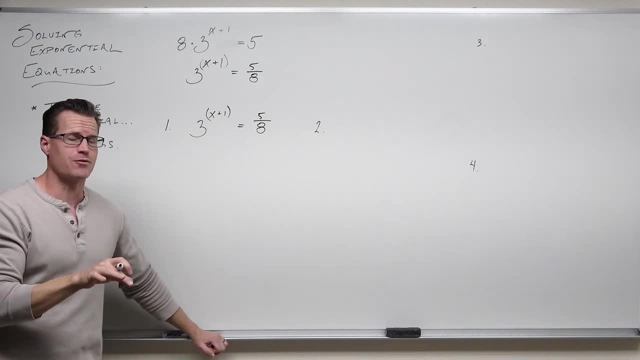 logarithm by going directly to logarithmic notation. We've actually seen that before, So we just identify: well, what is our base? Well, base is three. What's our exponent? Our exponent is x plus one, and what they're equal to is five-eighths. A logarithm will rewrite that for us. It will solve. 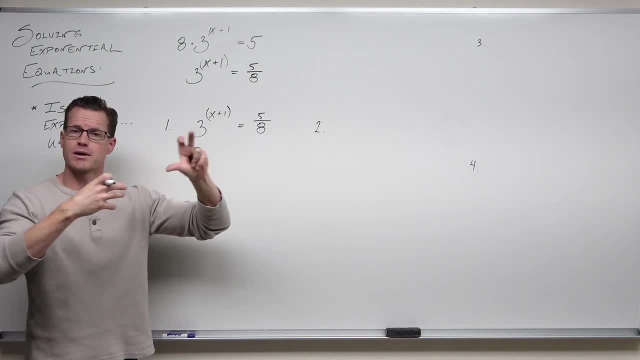 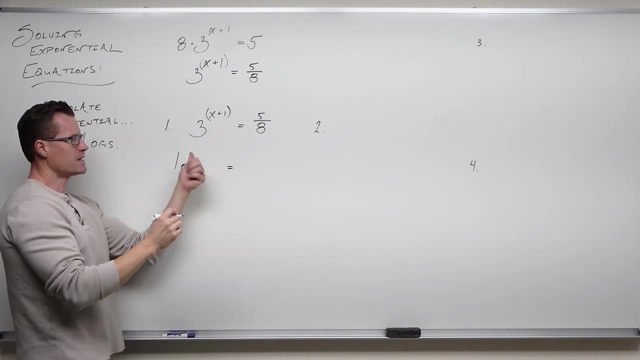 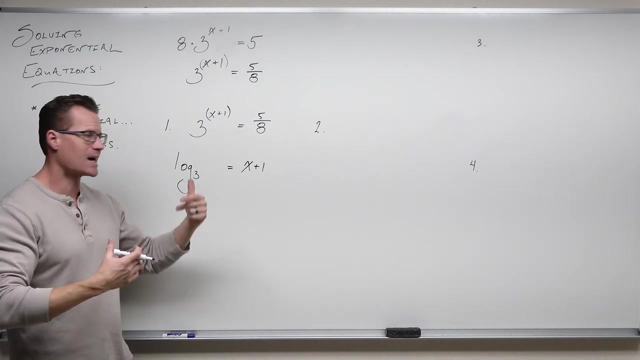 for your exponent. So logarithms take the base and the exponent and separate it on different sides of your equation. So it takes your base of three, your entire exponent of x plus one. Can you see why we put that in parentheses? So we don't lose that, So we don't actually add or subtract one right now. 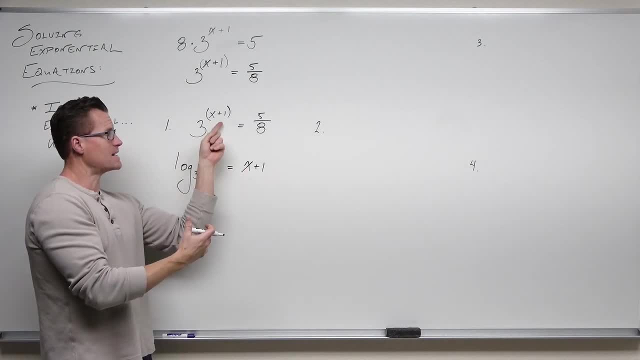 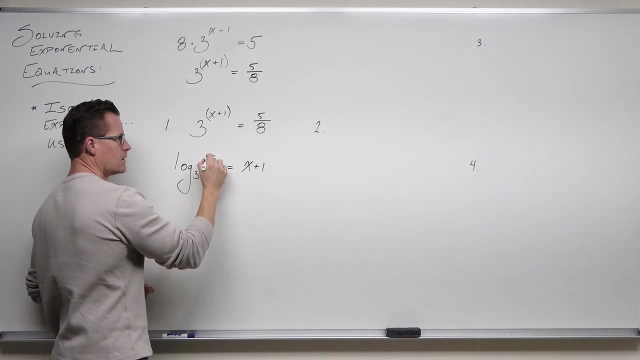 We have x plus one on one side. Yeah, we're going to subtract one, but it's not from the five-eighths, It's from a logarithm, And then five-eighths is the inside of our logarithm, And we're going to put that in parentheses, not because it's strictly necessary. 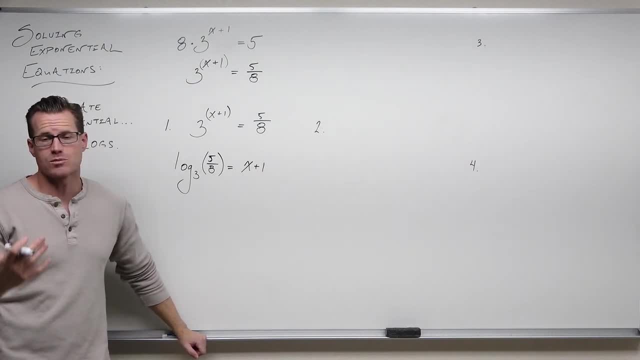 but because when we subtract one, we're going to get a logarithm Here in just a moment. we don't want to accidentally subtract it from the argument of a logarithm. That's exactly what we're going to do. We have, hey look, a logarithm will solve. 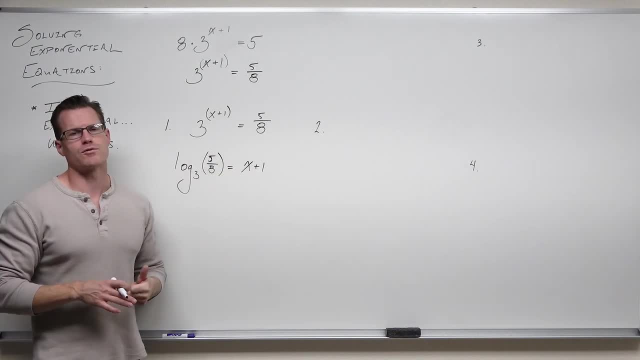 for your exponent. Because your exponent contains your variable, it's solving for your variable. practically, This is the easiest and most straightforward way to solve an exponential equation. if there's just one exponential, is writing this directly as a logarithm. Now, if we subtract one, 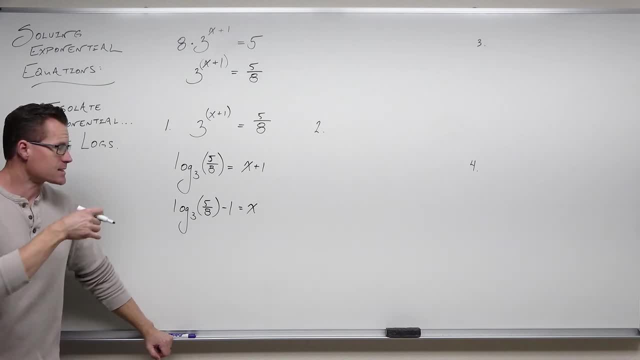 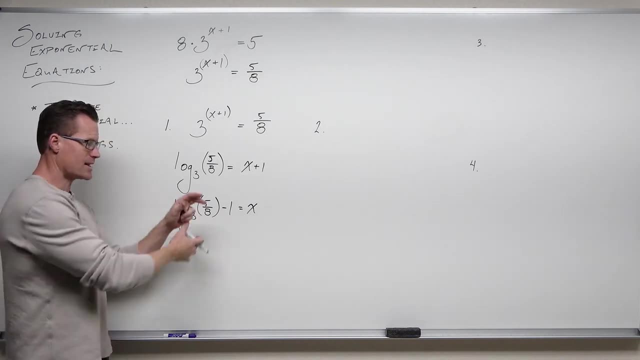 we're done. That's as basic as this gets. That's as simple as we can write this solution And it is a solution. This is what's called an exact solution. It is not an approximation. It has everything in there, if you will. If we wanted an approximation, you'd have to put that. 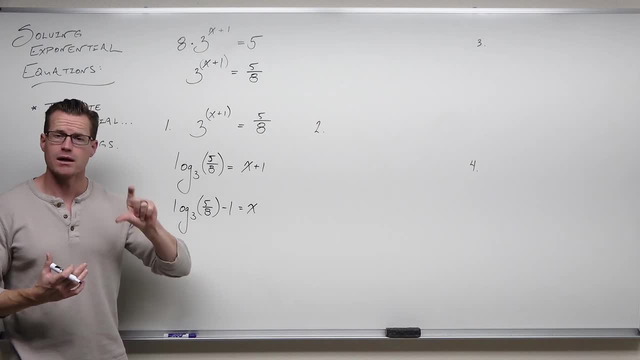 in your calculator. Now, some of you can't, because you cannot do anything beside a base of 10 or a base of e, like a common log or a natural log respectively. So what could you do If you had to approximate this? 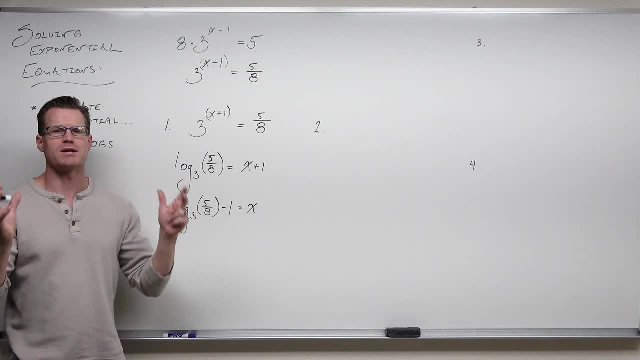 we would use what's called the change of base formula. We talked about that. It says: pick whatever base you want- Well, usually a base of 10 or a base of e, And you could write this as a common log of 5 eighths. 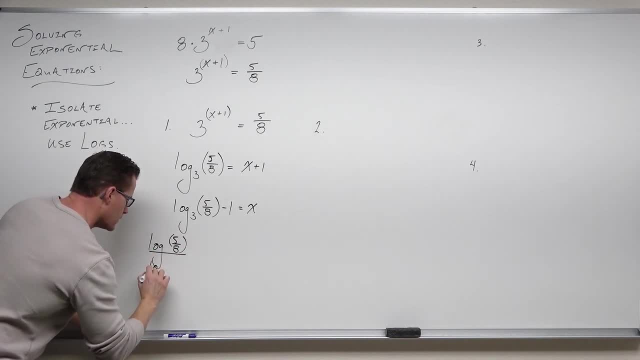 over a common log of 3.. Remember, this goes on the numerator, the base goes on the denominator and you pick whatever base you want. In this case you pick a base of 10 because that's on your calculator And the minus 1 comes after that ratio. 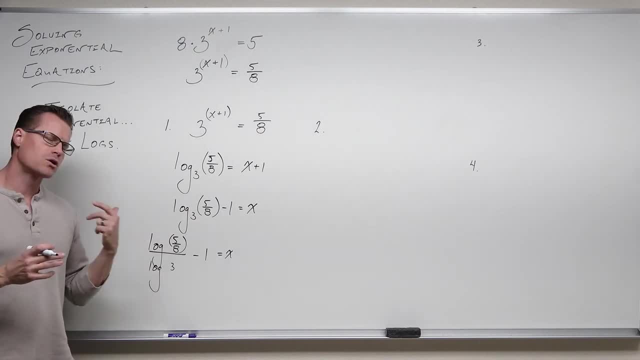 So you plug this in or evaluate Log of 5 eighths. Now could you write that as log of 5 minus log of 8? You could do that. Is it beneficial? It depends, I mean, sometimes maybe. 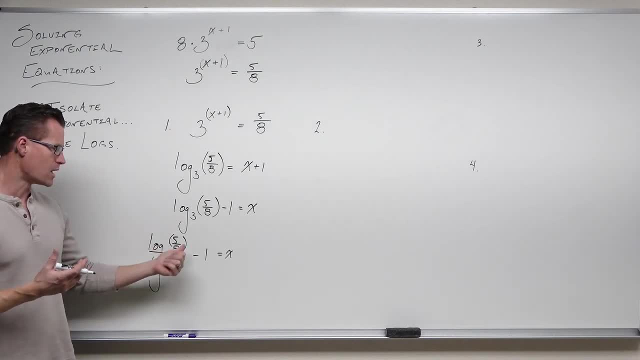 but here if we're just trying to approximate, probably not Just plug in a fraction, Then divide by log of 3.. Get that, whatever that approximation is, and then subtract 1.. You could have also chosen ln. So if we take ln and use that, 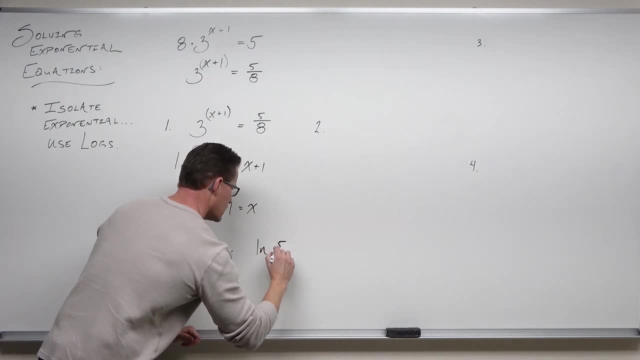 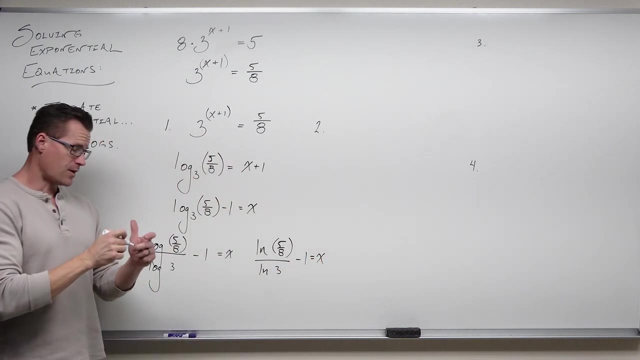 as our new base, we'd get ln of 5 eighths over ln of 3,, all minus 1, and that would equal x. These are the three appropriate solutions that we can get out of this. Is it okay to have any one of those? 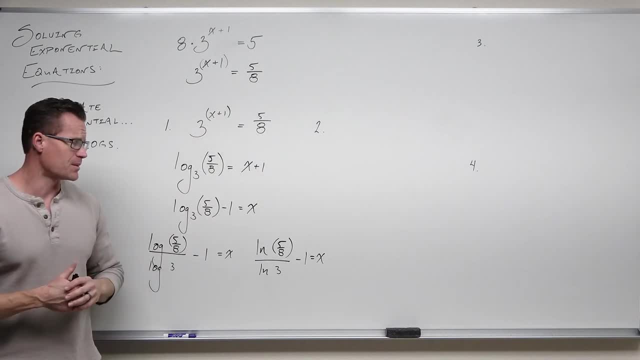 Yeah, absolutely. We're going to see that in the other three examples that we do. So this is the most straightforward way to solve this: Isolate your exponential and then go directly to logarithm. You know, take the logarithm. however, 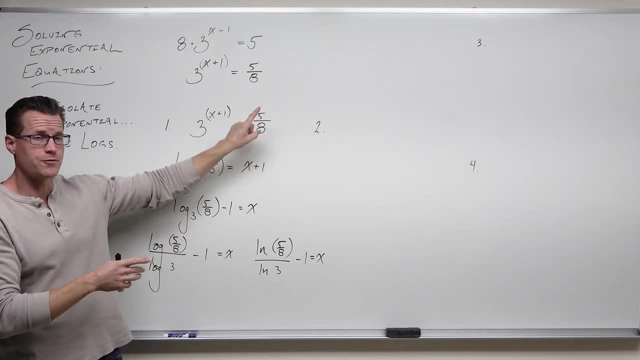 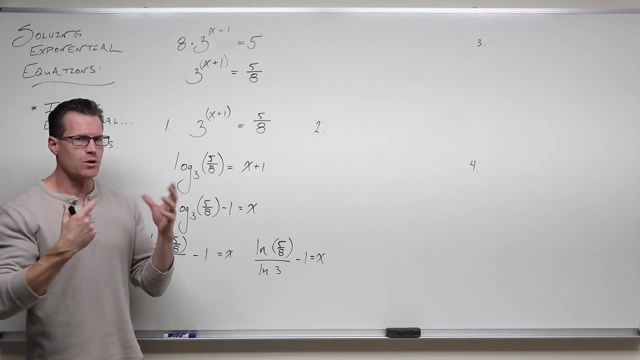 this does not always work. If you have another exponential with a variable, this technique won't work because you can't go to one logarithm if you have two different bases. That would be a problem If you don't have two different bases. 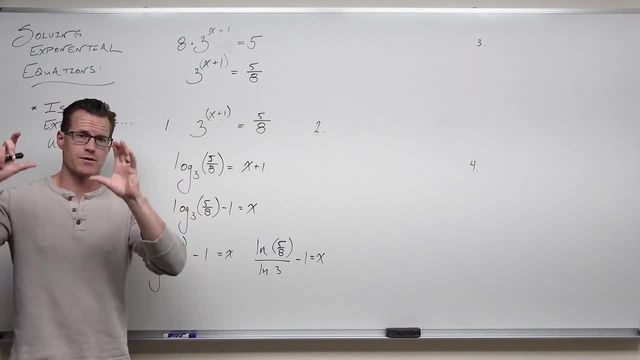 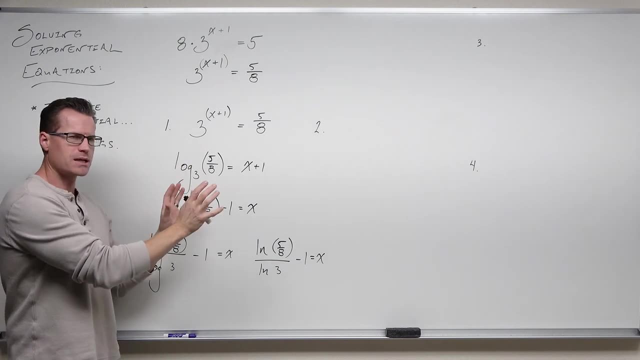 you have the same base, then we wouldn't even be doing this. We'd have the special case of: hey, I have common bases, Let's set the exponents equal. So that wouldn't be relevant. So let's go ahead and let's learn another technique. 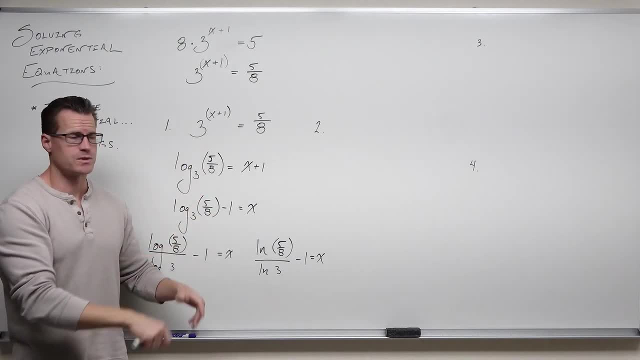 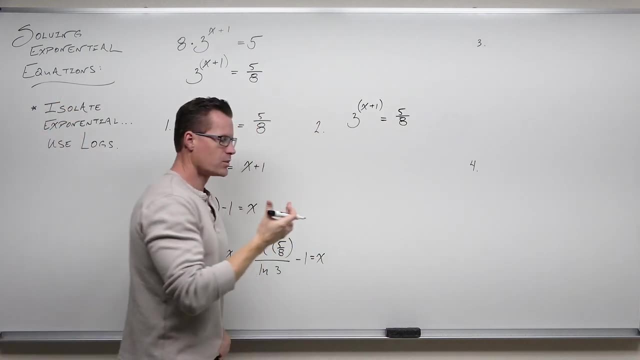 that says, well, what would happen if we don't have just one exponential? These are going to, they're all going to work, But two of them are preferable, So let's go to the next one. So what if we had three to the x plus one? 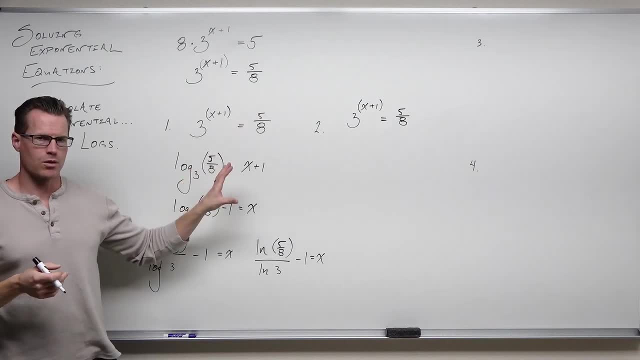 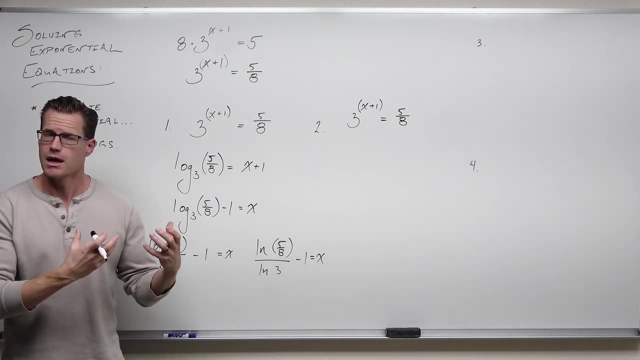 equals five eighths again, and we don't want to go directly to logarithm and notation In exponential equations. you can do almost anything you want, as long as you do it to both sides. We can take a logarithm of both sides. 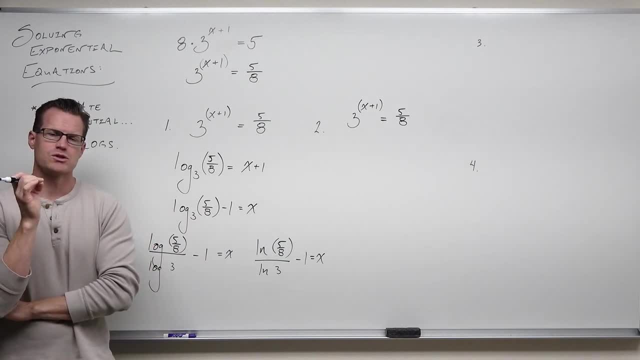 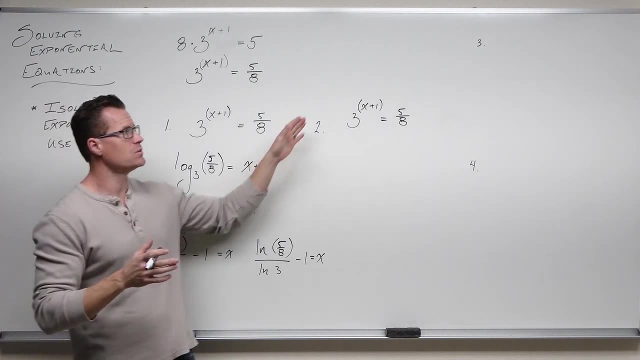 Now why in the world do we want to do that? Well, if an exponential's inverse is a logarithm, a logarithm will undo that exponential. So let's take a logarithm. Now, the next two choices you have to solve these are: you choose. 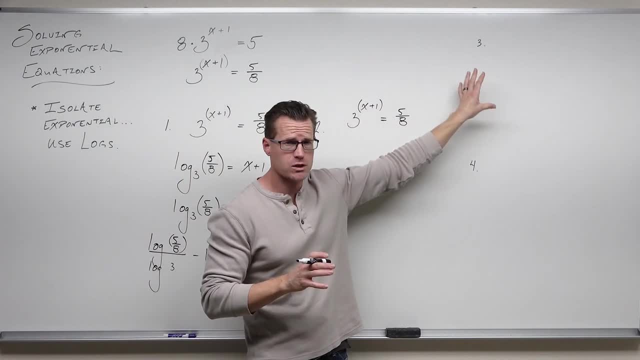 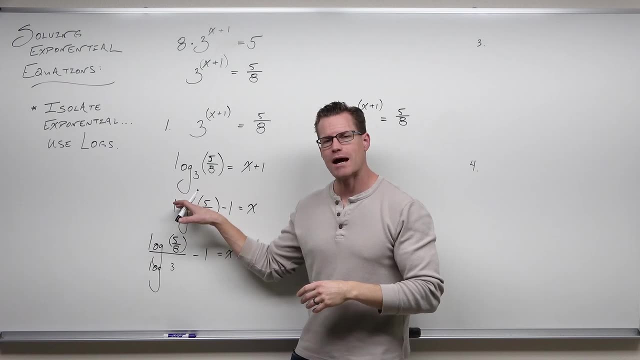 either a common log or a natural log. Most people use a natural log. A common log is a base of 10 and natural log is a base of E. Now, why we want to do that is so that we don't have to go and do change. 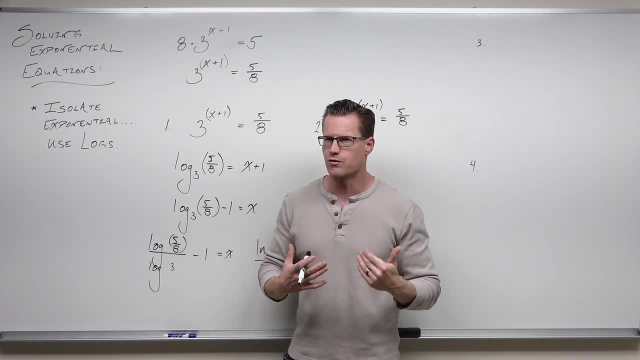 a base. anyway It already be in a base. that's very usable for us, for most people and their calculators. So we choose a common log or a natural log to do that. The last example is: what if you were really smart and you took a logarithm? 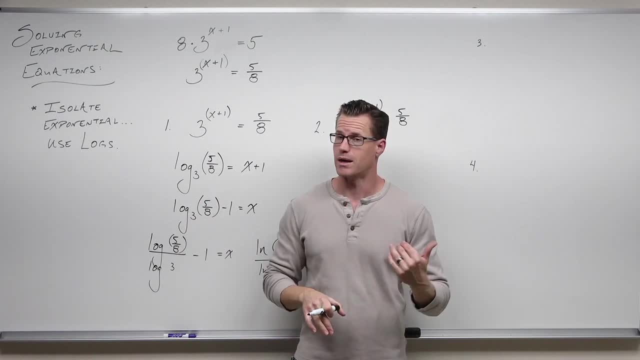 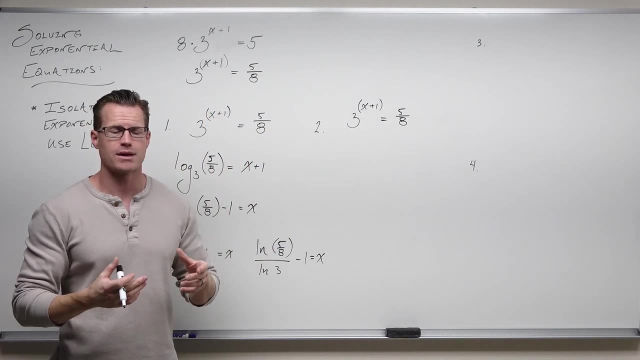 both sides with a base that inherently matches here. Well, that would be nice too, So we know what everyone's long do at both sides. Let's take a log of both sides. Let's choose a base 10, so that that way we can evaluate our calculator when we get. 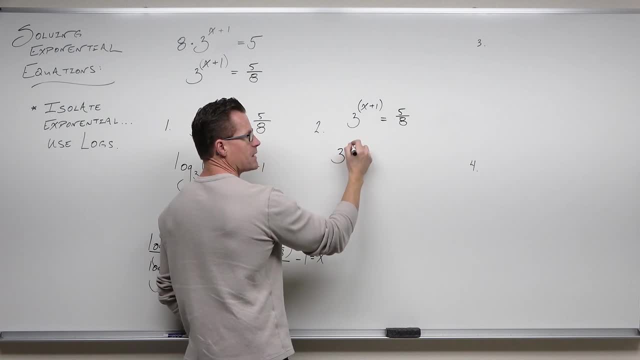 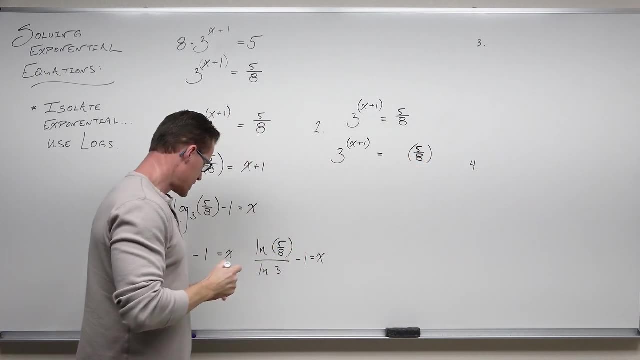 to the end, very nicely. So we would take our three X plus one and our five eights and we would take a logarithm on both sides. Whatever base you want, right, But we're picking a base of 10 because that's on your calculator. 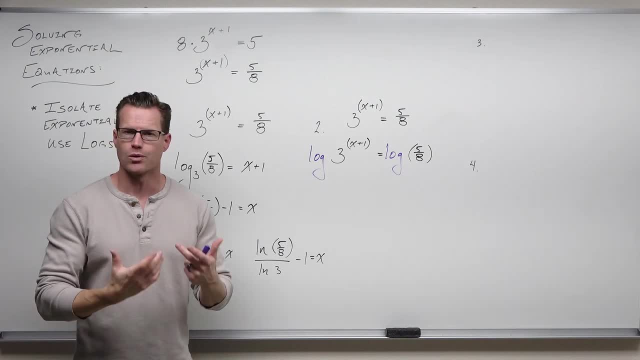 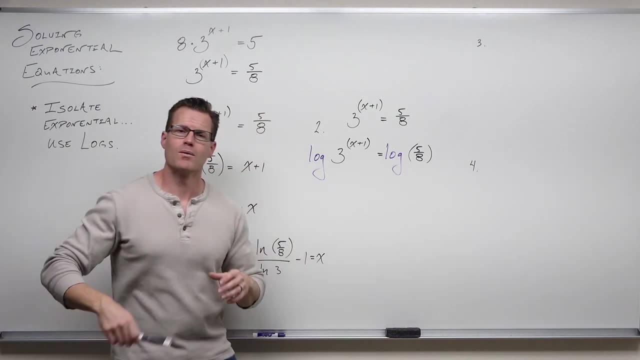 Now why in the world this works on the right hand side, you still have a constant logarithm of five. eights is still a constant on the left hand side, though. why a logarithm allows us to solve an exponential is because it allows us all. this is a beautiful thing. 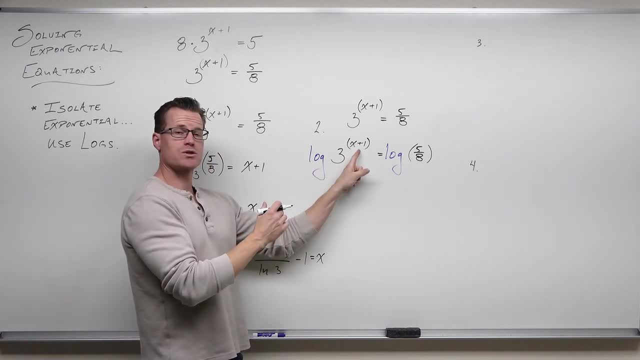 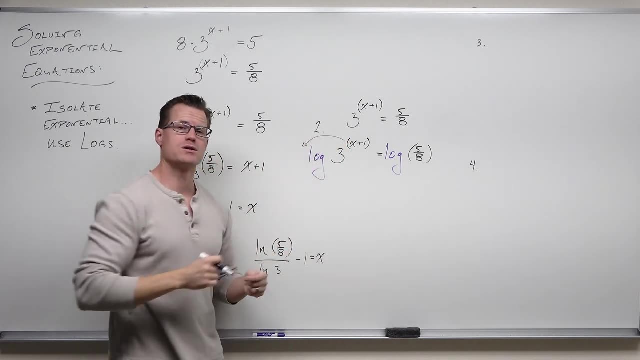 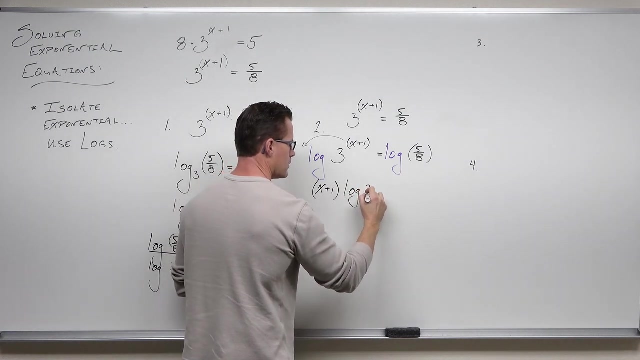 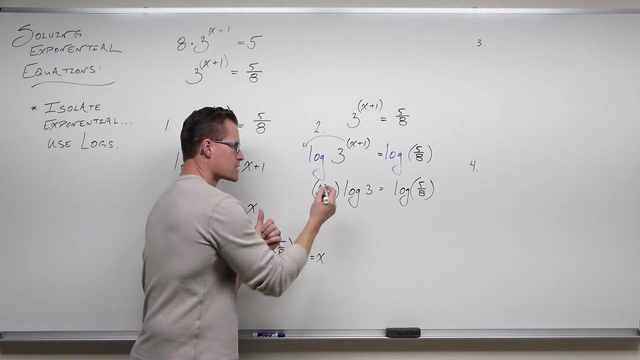 You see it, log base 10 of three to the X plus one. The X plus one is now an exponent on the inside of your logarithm by the power property. You can move that to the front of your logarithm. So we would get X plus one times log of three. 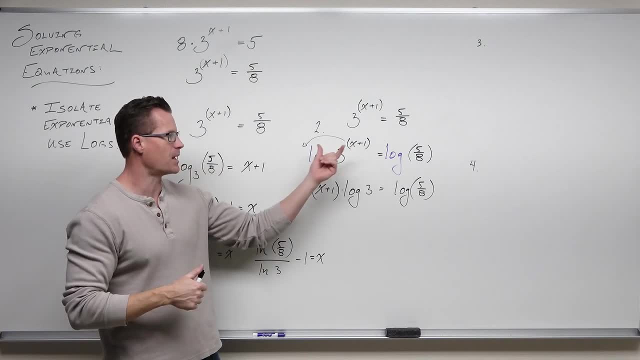 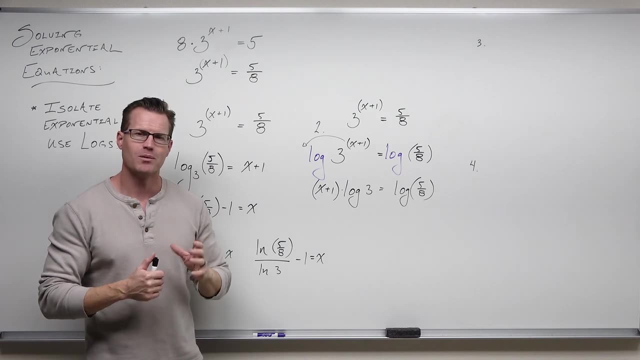 equals log of five eights. They're still based on logarithms, but by the power property we can move that exponent to the front as a coefficient. Now why is that useful? Well, because that's now just something I can solve for. 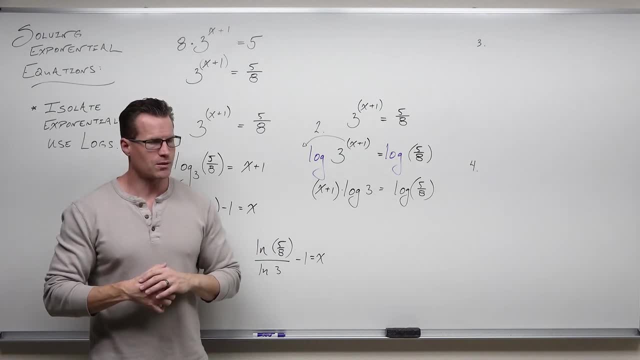 I can solve for that X really nicely. There's a couple of things I I really really want to point out to you that if you don't pay attention to anything else, this is super important. This is where almost every mistake comes from. 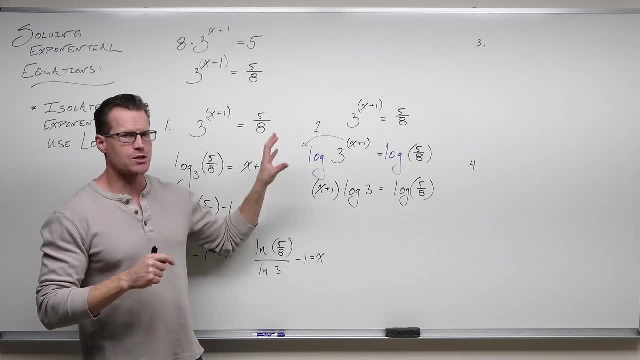 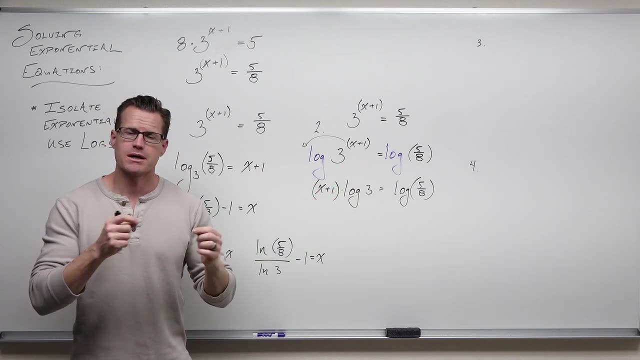 I'm moving on number one. You absolutely have to have this exponent in parentheses When you move it to the front. it's a must. Why? Because most of the time you're going to have to distribute that And, if I allow you to write that with F X: 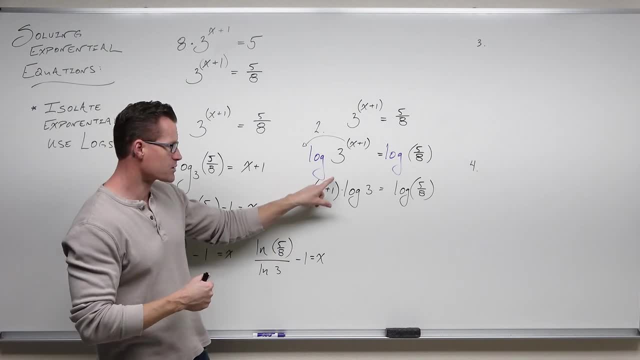 without the parentheses. some people aren't going to see it, Some people are going to. if I don't have those parentheses, they're going to go. Oh, I just subtract log of three and I'm done. No, you're not. 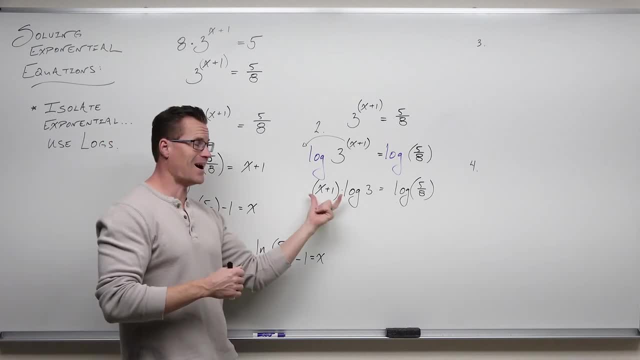 You make a very, very important choice. And the second thing I want to bring up, So number one, you got to have parentheses. It's a really big deal. It shows what you're actually doing. It shows you're multiplying the exponent times, the logarithm. 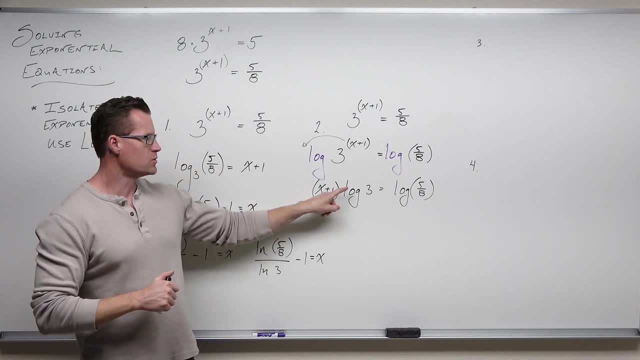 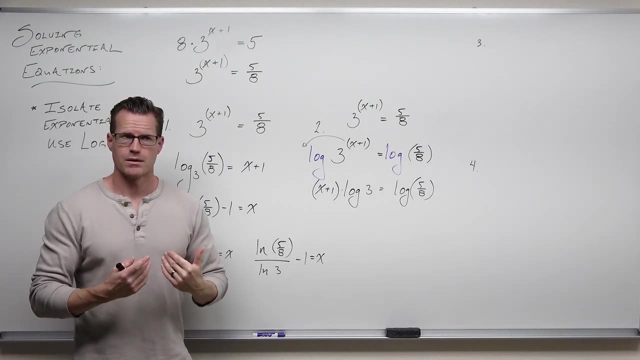 Secondly, you make an important choice here. The important choice is: you choose whether to distribute or not. Here's when to distribute. Firstly, if you don't understand what I'm about to say, I do it all the time. You can't really mess it up. 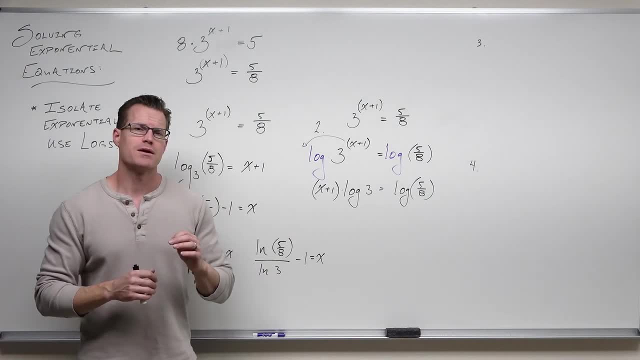 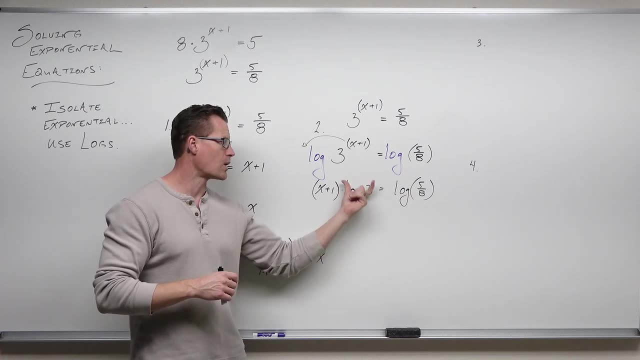 do it all the time, distribute all the time and you can solve for X. Not all that bad. But if you don't, if you, if you do understand this, if you have no other X's anywhere in your equation, you don't have to distribute this. 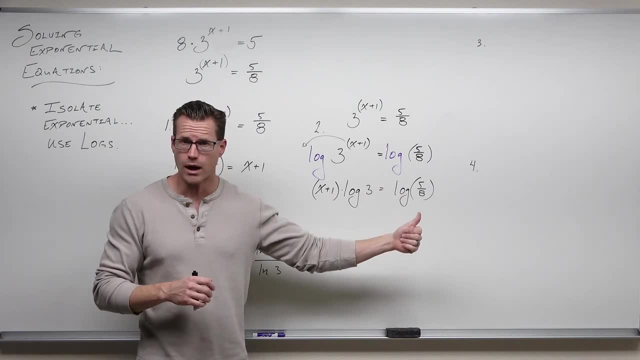 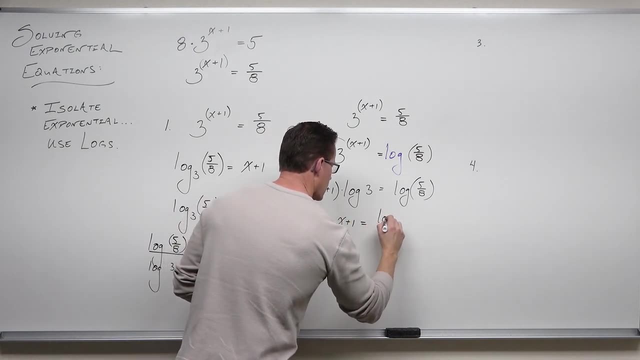 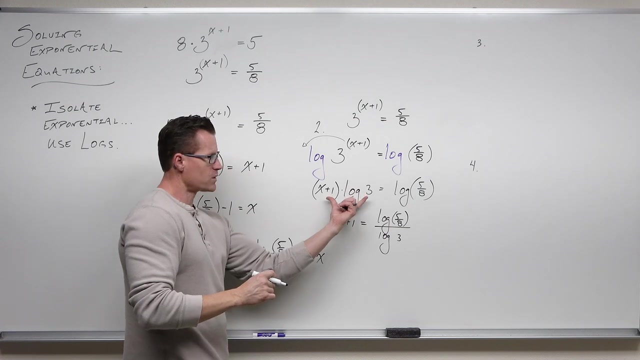 You can divide by log of three and then subtract one. That would be fun. You could do that. So dividing both sides by log of three, we have this. wait a minute, Oh, it's really, really familiar. It's the same thing. 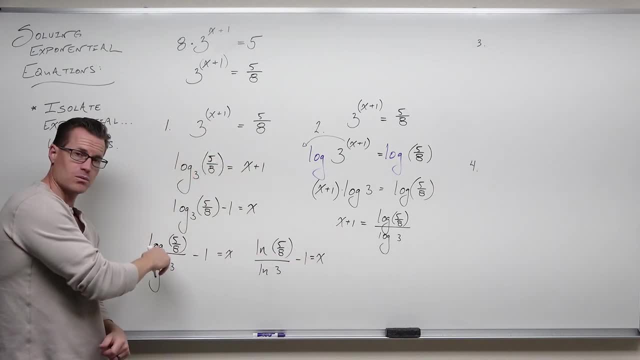 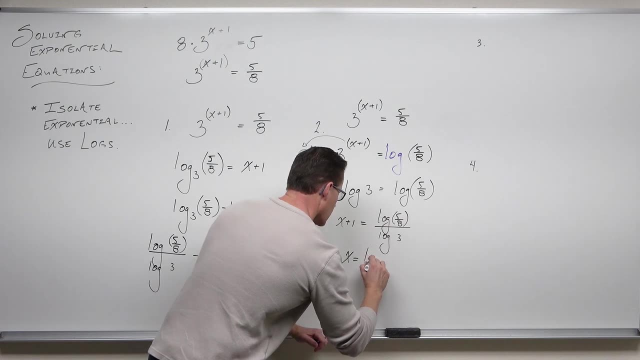 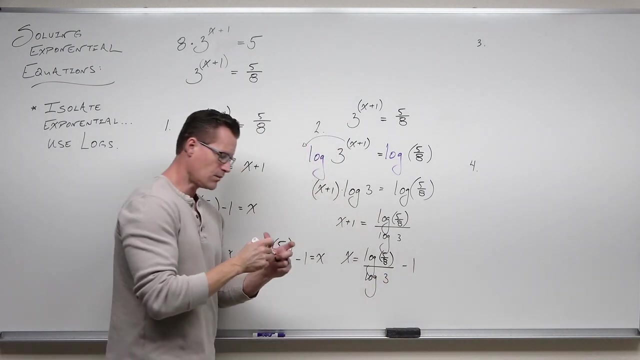 And if we subtract one, we would get exactly exactly this right here. We would get exactly log of five eighths over log of three minus one. That is perfectly fine. Now I said also: well, wait a minute, Uh. 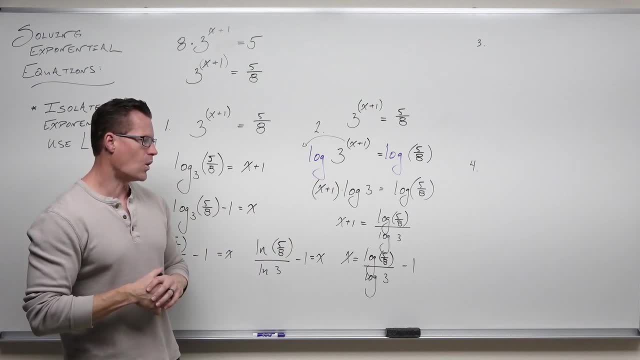 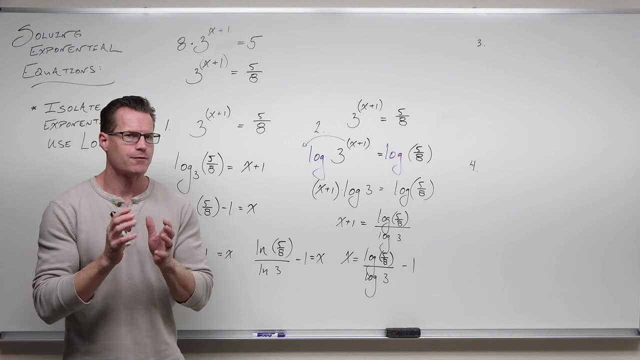 could you distribute? you could distribute and it's not all that big of a deal. but I want to show it to you to make sure that you see that. So you see that our answers can look different. When do you have to distribute? 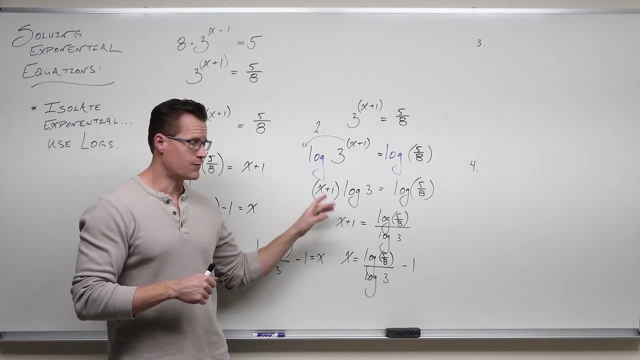 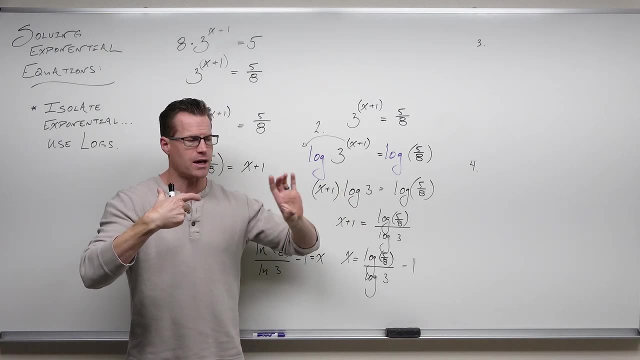 Again, you have to distribute. If you have more than one X, if you have any other X is floating anywhere around here. you've got to distribute. combine your X terms on one side, your non X terms and other factor in X and divide. 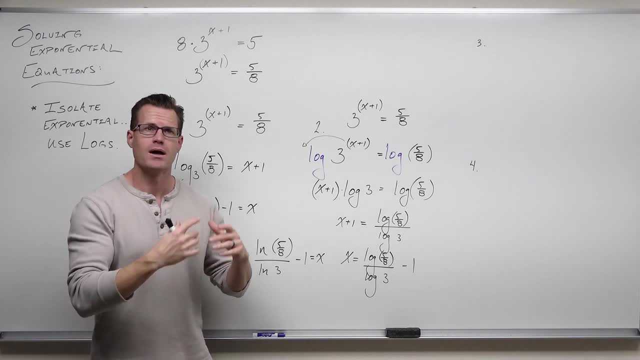 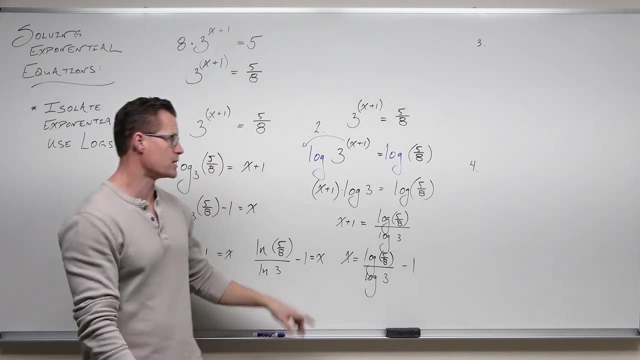 We've seen this as the fourth time that we will have seen this in this class, this idea of- Oh yeah, I have multiple things I'm trying to solve for- distribute, collect them, factor, divide. That's the idea. I'm going to show that to you. 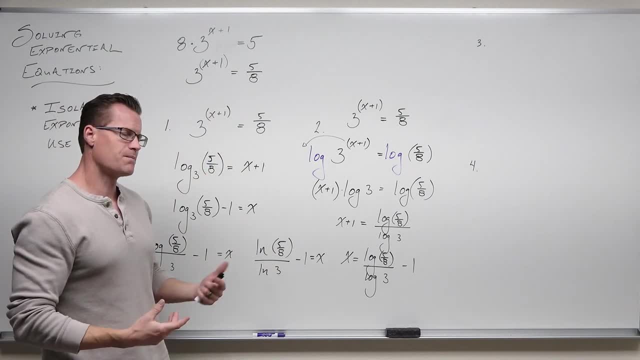 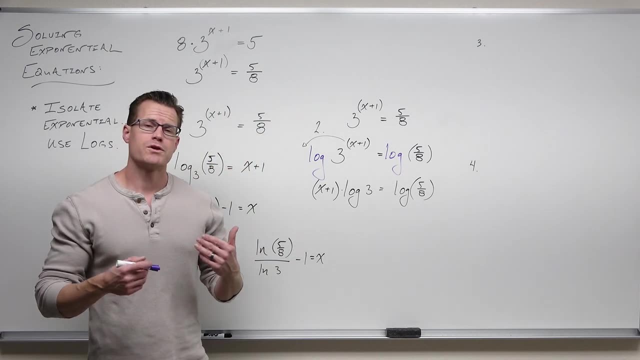 Kind of preface what we're going to do after we finish these, these four techniques on the next examples. So this is cool. We've already seen it, It's exactly the same thing. Now what if we chose to distribute something you will have to do in some of the 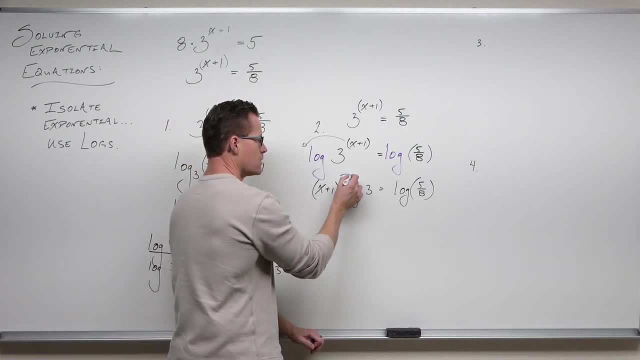 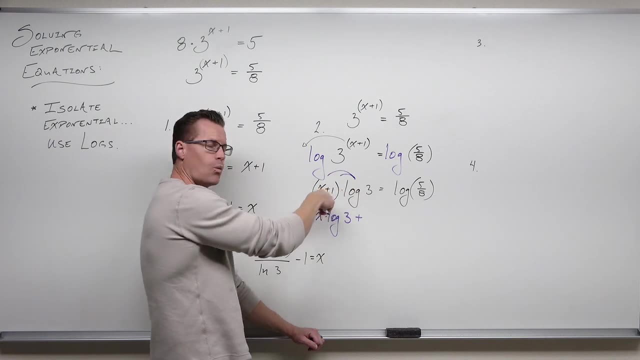 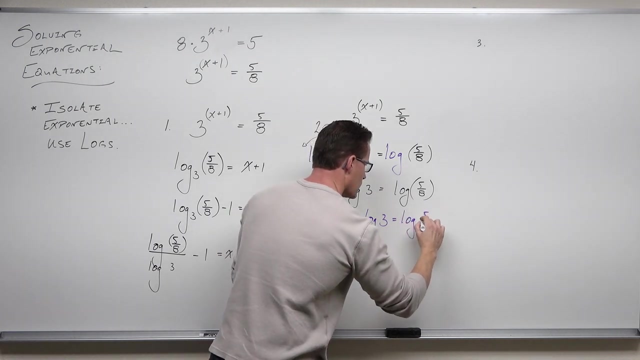 examples moving forward. if we choose to distribute, we get X times log of three plus one times log of three, which just log of three. As always, I'm trying to train you on where we're going to get to in a little while. 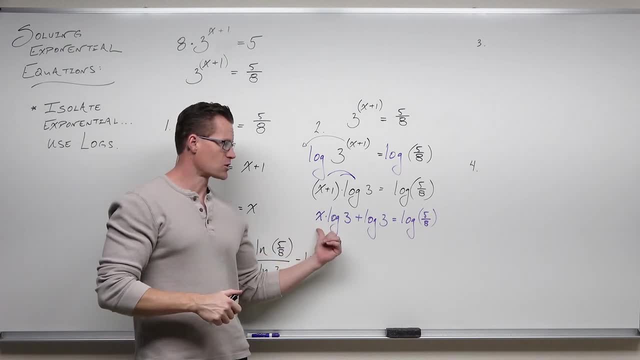 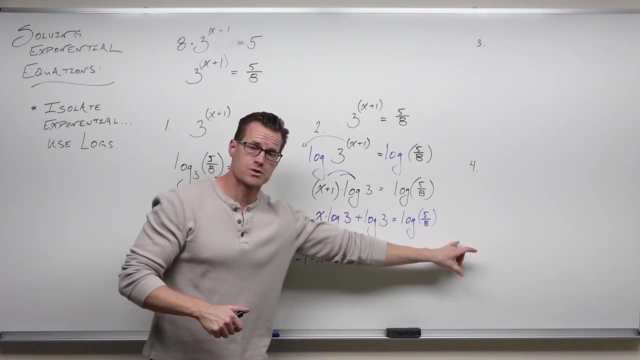 In a little while. What's going to happen is you'll distribute. You had an extra here and X term here. maybe somewhere else you will combine. you or your move your extremes to one side, your non extremes The other than your factor in divide. 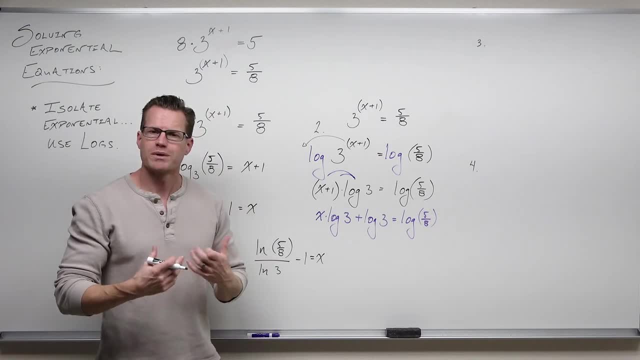 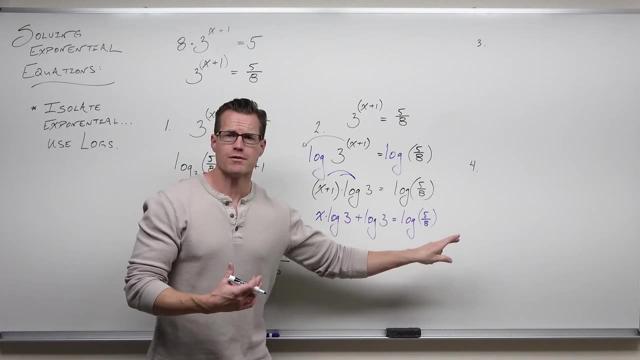 That's what we're going to get to in just a little while. here We're kind of doing the same thing. We're getting our X terms on one side. That's this one. that's already there. This is not an extra. That means you've got to get rid of it so that you can divide between them. 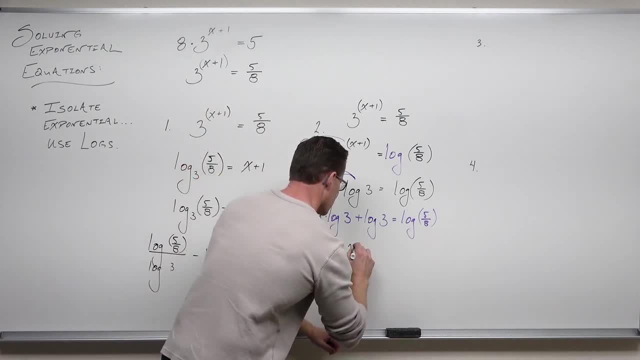 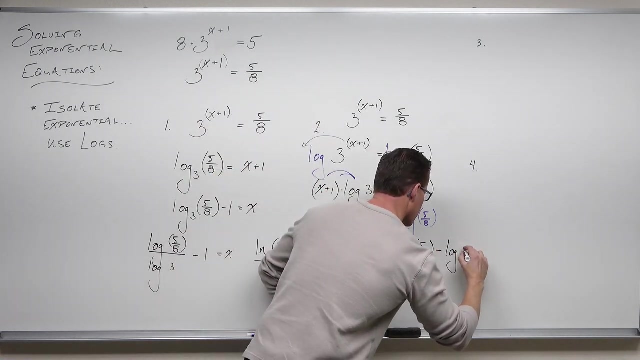 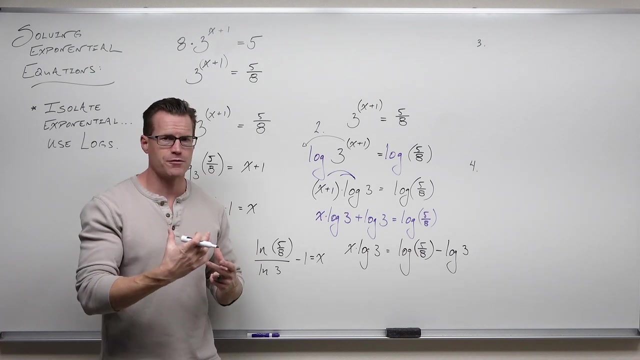 appropriately, We're going to subtract log of 3.. I'm still keeping that 5 eighths in parentheses, so I don't accidentally subtract. And lastly, because we have one x term, because that's connected by some coefficient. this really is a coefficient. 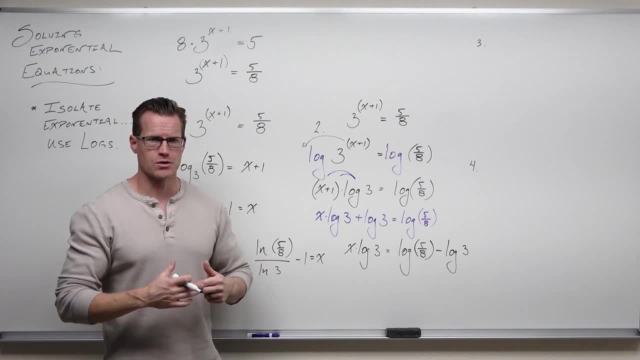 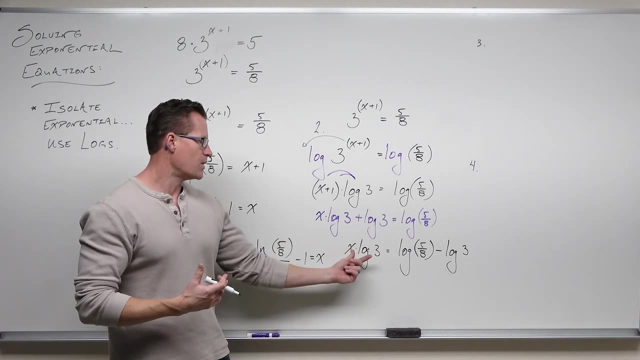 log of 3 is just a constant. It's saying 10 to what power gives you 3? It's an exponent of 10 to that exponent gives you 3.. It'll be some sort of decimal there, but this represents a number We can divide by that. So if we divide both sides, 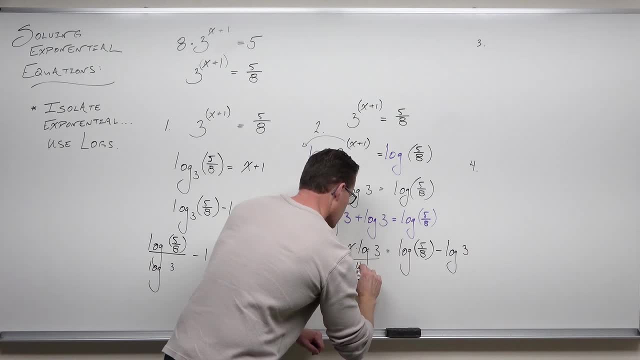 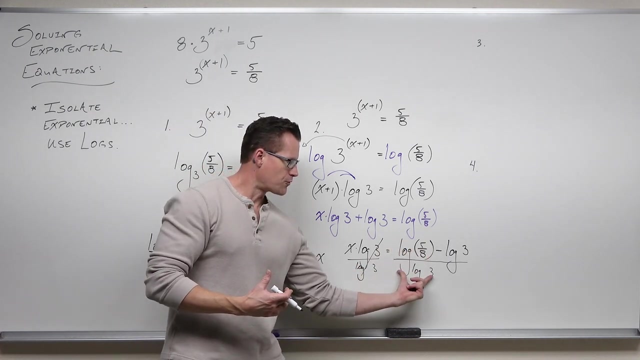 by log of 3, here's what we would get. Remember that when you're dividing, you can separate one fraction minus another fraction. but take a look at what you would get. This first fraction would be log of 5, eighths over log of 3. 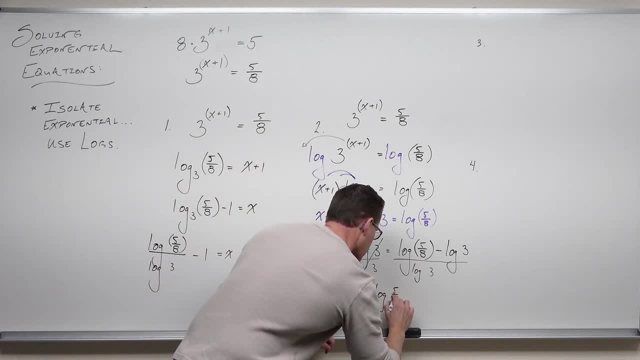 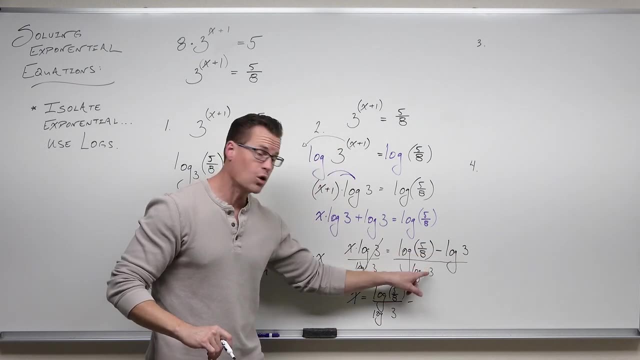 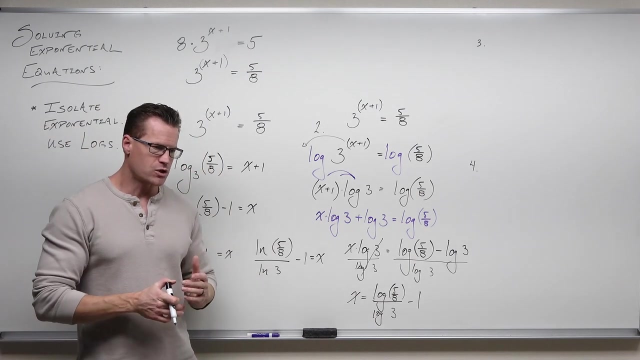 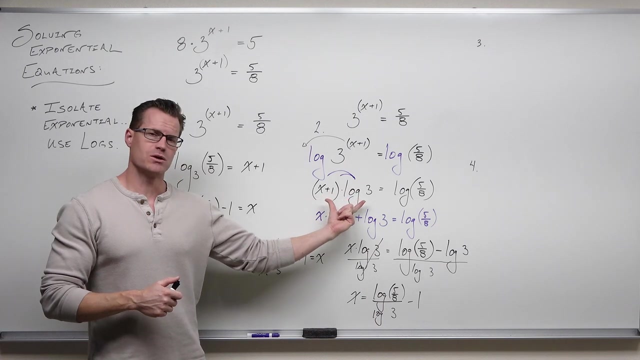 minus log of 3 over log of 3, which is 1.. And that's precisely the same thing that we get right here. So which way is better? Well, that's a personal choice. I said, suppose, Me, I like to divide right here when I don't have to distribute. But if I'm 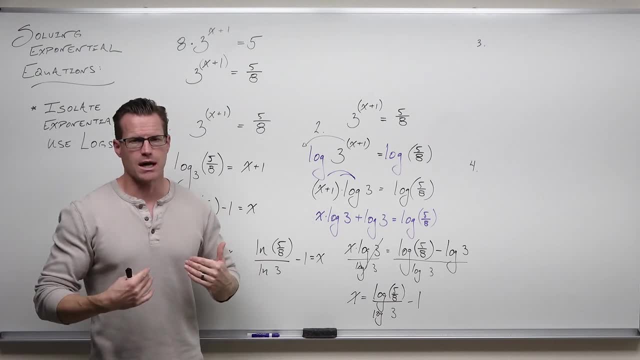 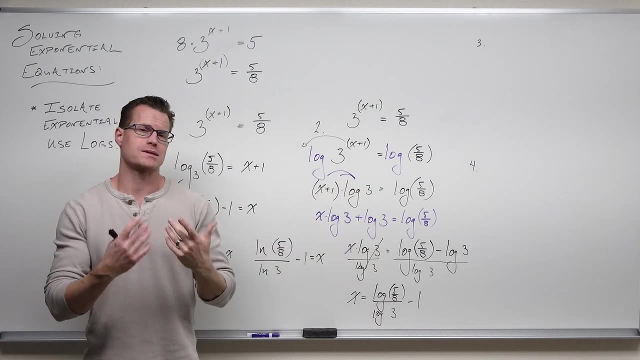 not confident on knowing what I need to distribute. I'll distribute every time. There are times when this will not work. You cannot just divide it. If you have x's anywhere else, you have to distribute. I hope that sunk in for you. Let's move on. 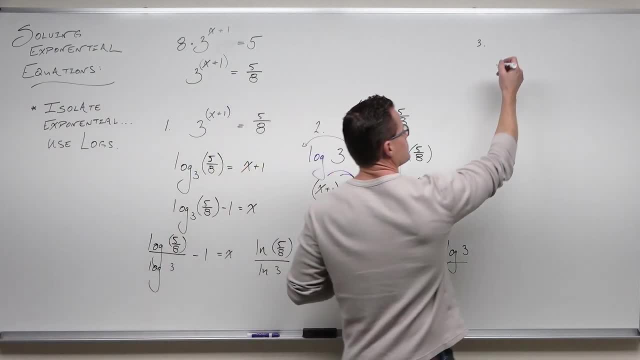 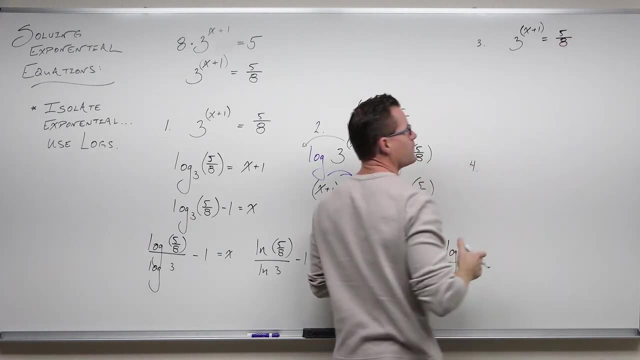 to the next way. So I'm going to start over with 3 to the x plus 1 equals 5 eighths. So I'm going to start over with 3 to the x plus 1 equals 5 eighths. I'm going to start. 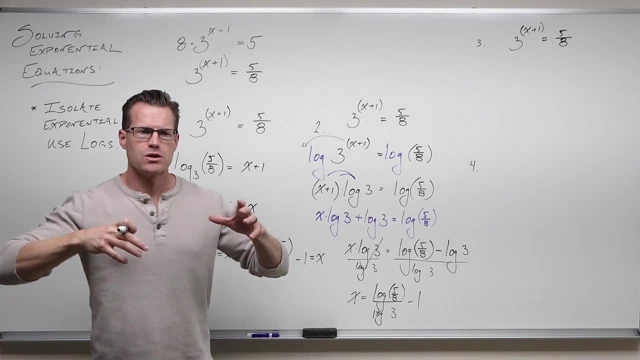 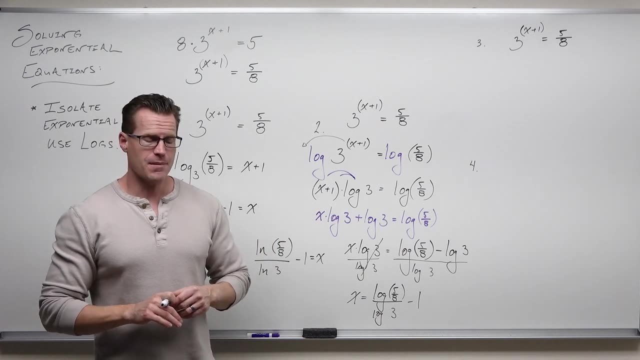 over with 3 to the x plus 1 equals 5 eighths. I'm going to take a log on both sides again, but I'm going to do a natural log. This is usually a very preferred way for people because it's ln, not a lot of writing. one less than a log. one less letter every time, And also. 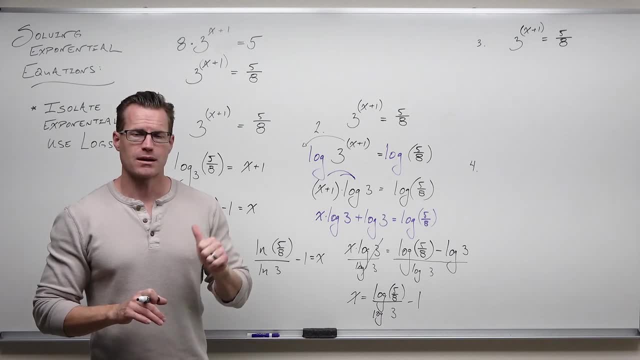 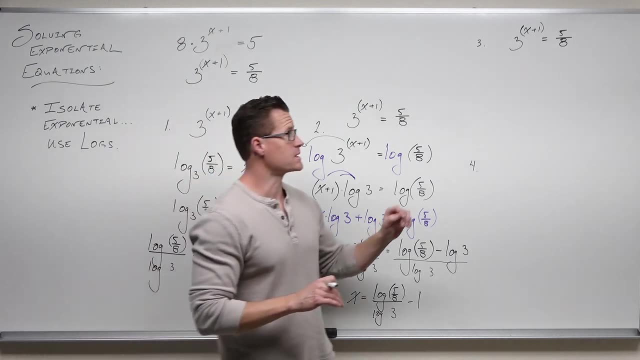 that if you ever have a base of e, a natural log automatically composes with that. Now I want you to think about that for a second. Could you use a logarithm that automatically composes an inverse with an exponential? What base would that be? And that's our fourth. 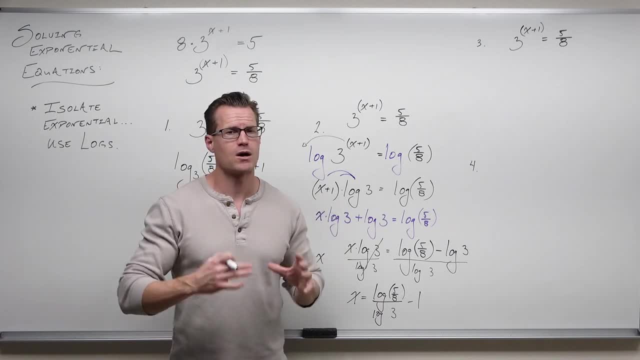 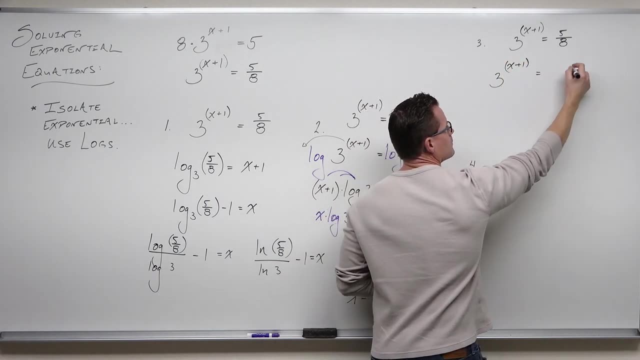 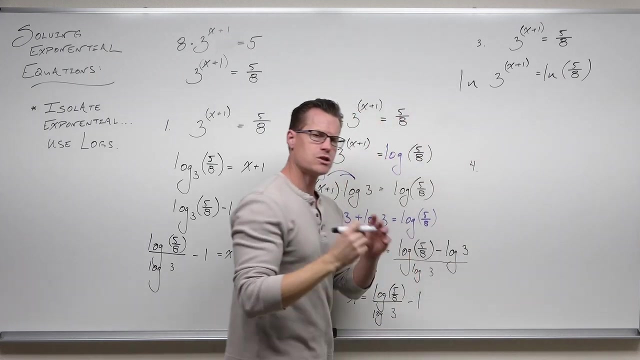 technique. So here we're going to choose a natural logarithm. It's a very common thing to do. So we're going to choose a natural logarithm. It's a very common thing to do And we would get on both sides: log base e, log base e. Once you do one side, you have to do the. 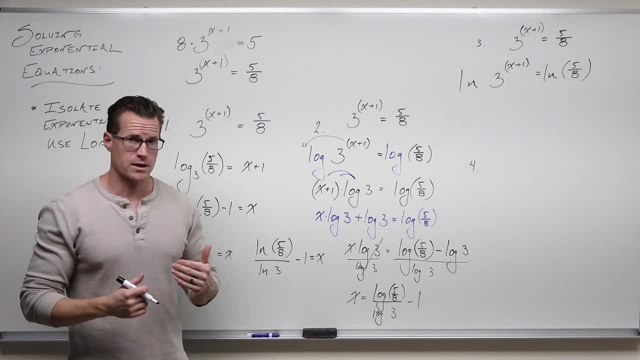 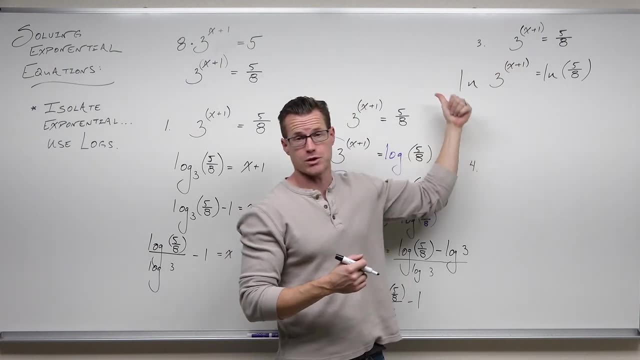 other, It's going to model exactly like this, So I'm not going to spend a whole lot of time doing this. What this lets us do is, if you have a logarithm on some exponential, it lets you move that exponent to the front as a coefficient, but you got to keep it in parentheses, So that's x plus. 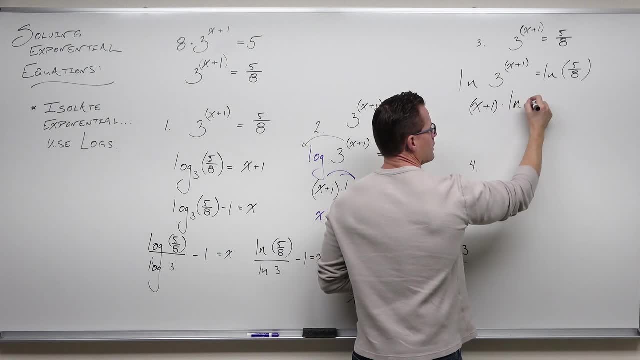 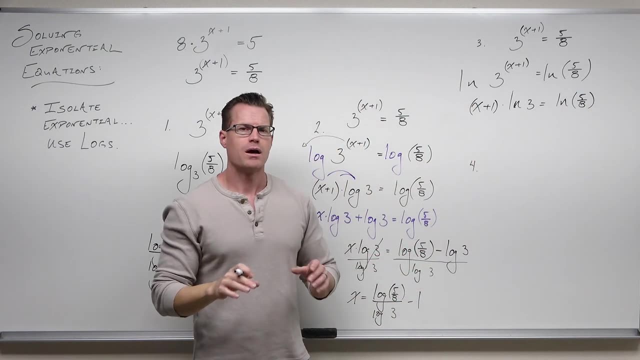 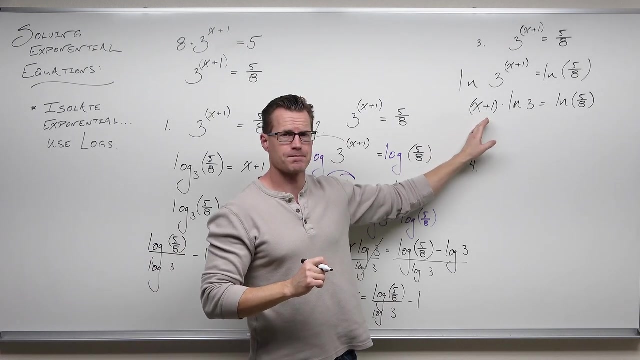 one ln. three, ln. five, eighths. Think in your head right now. Do I absolutely have to distribute this? Do I have to absolutely have it in parentheses? Yes, Do I absolutely have to distribute this? Not if there's no other x's, but if there are, then yes. So this is a choice. 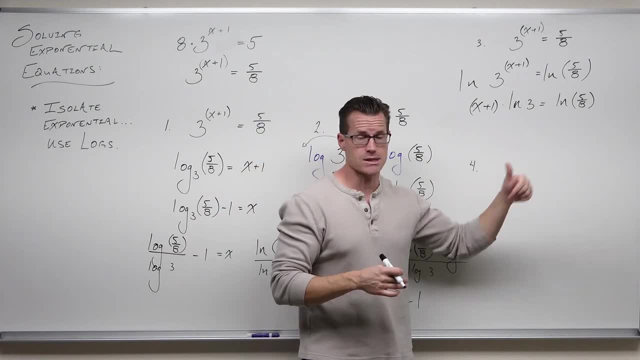 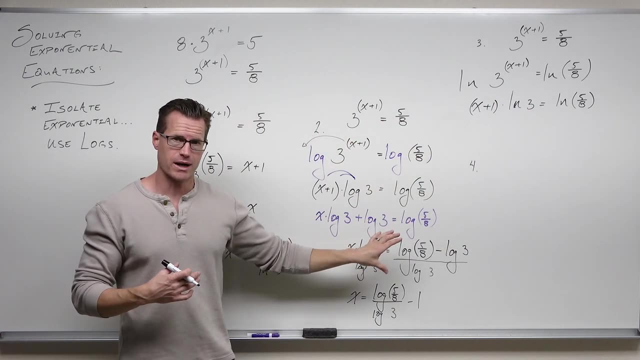 you make right now- This is the only time you get a choice- is when you don't have the other x's. You can choose to divide right now, which I'm going to do, or distribute Subtract and then divide, which is modeled right here. If you just change this to an ln. 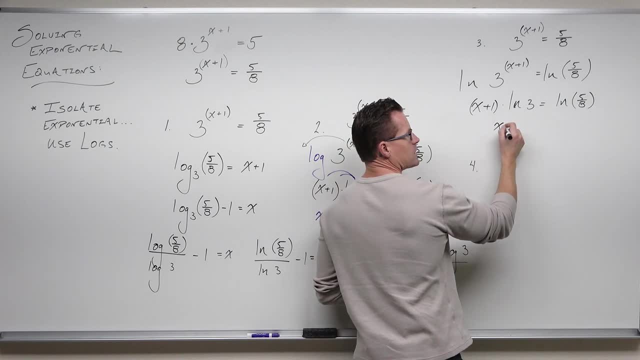 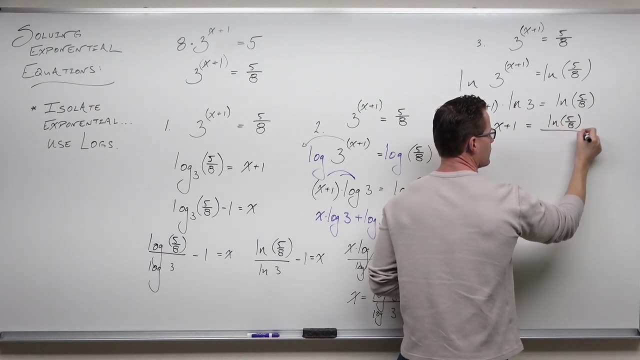 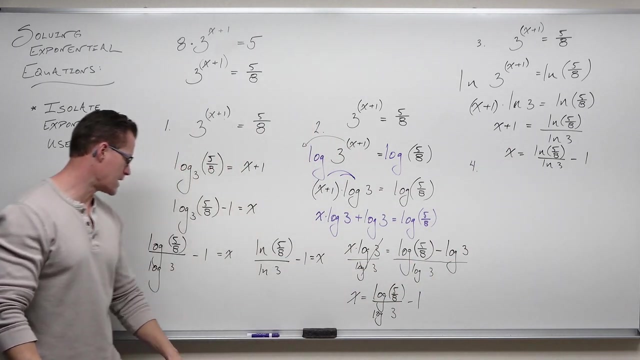 you get exactly the same thing. So we're going to do x plus one. I'll divide both sides by ln three. I'll subtract one. Now, how in the world do we know that this and this are the same as this over here, or this right? 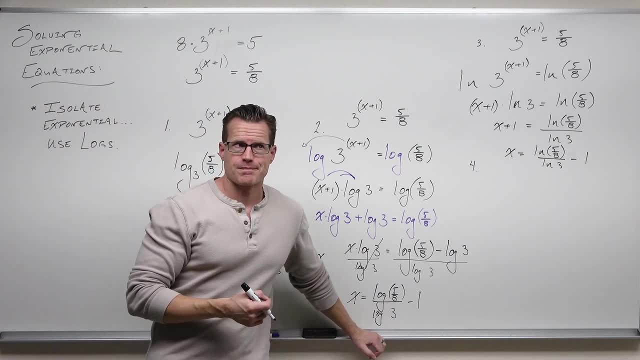 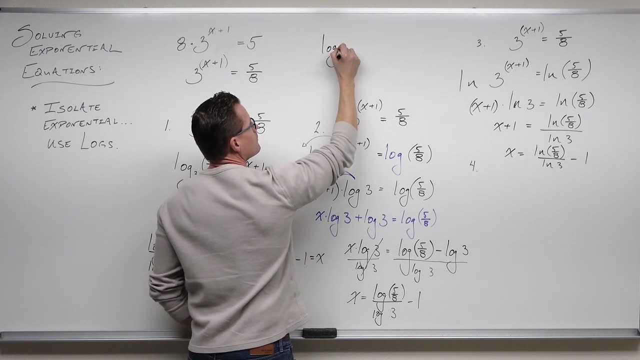 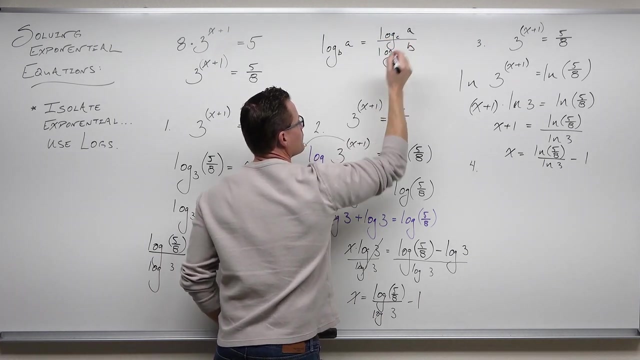 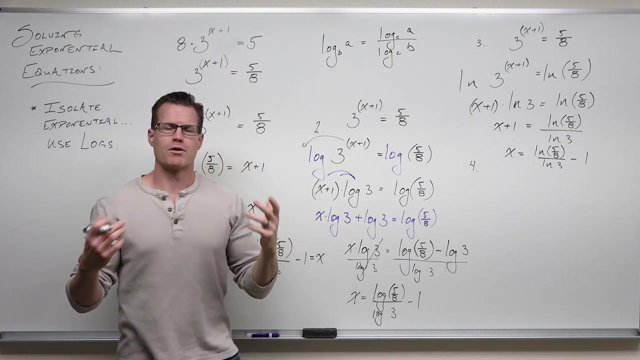 here. Well, we can still do the change of base, but only in reverse. Think about this for a second. If the change of base says that I can pick whatever base I want, just take the argument to the numerator base, to the denominator, pick whatever other base you want. 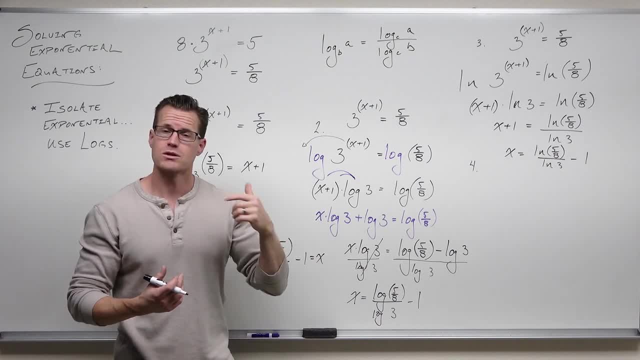 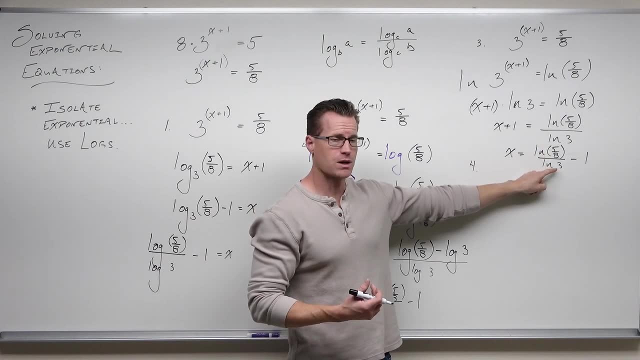 And you create this ratio: Can we go backwards? Well, as long as we have the same base, the answer is yeah. So if we have log base e of five eighths and log base e of three, this is your new argument and this is your. 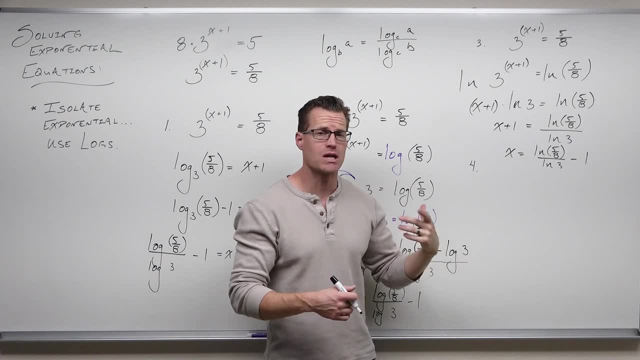 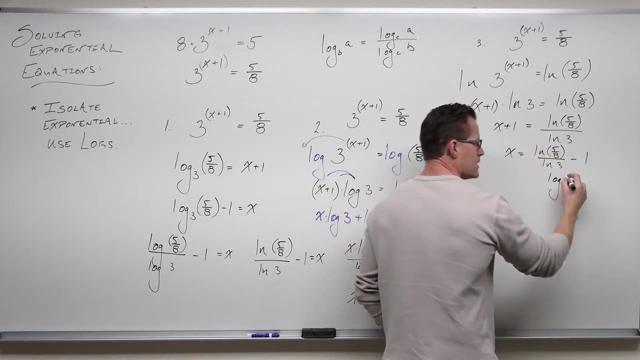 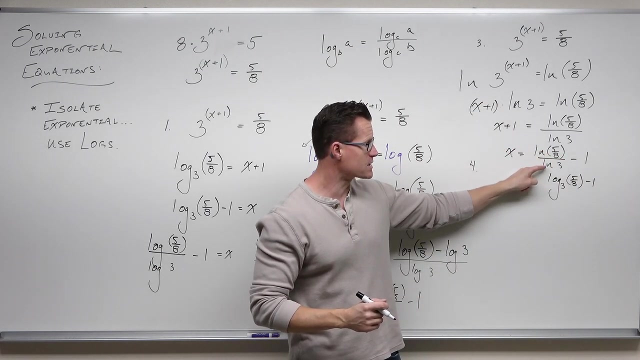 new base of some other logarithm, provided. these are the same base which they are, So you could totally write this as log base. three of five eighths minus one. You're just doing change of base in reverse. These have the same. 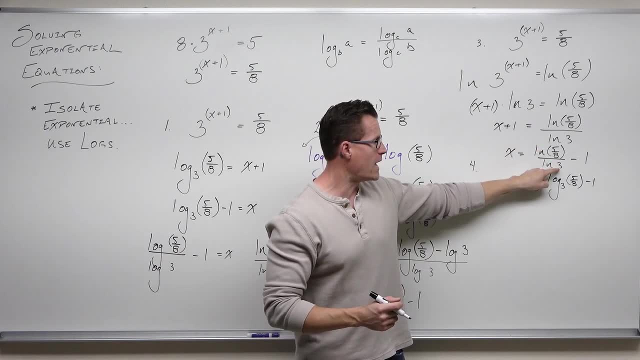 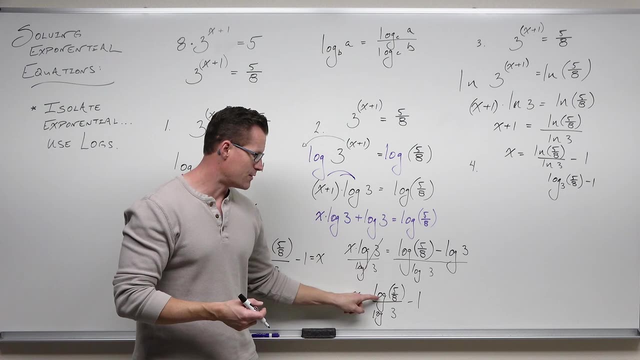 base. Therefore I can combine them to one logarithm, with that as the new base, that as a new argument. Same thing would happen here You have log base 10.. Hey, those are the same base. New logarithm would have a log of. this would be the argument. This would be the base, exactly like. 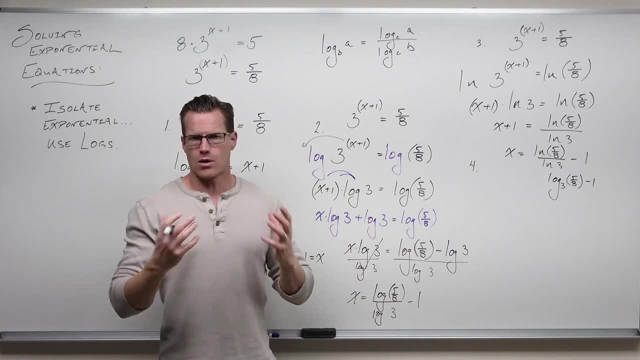 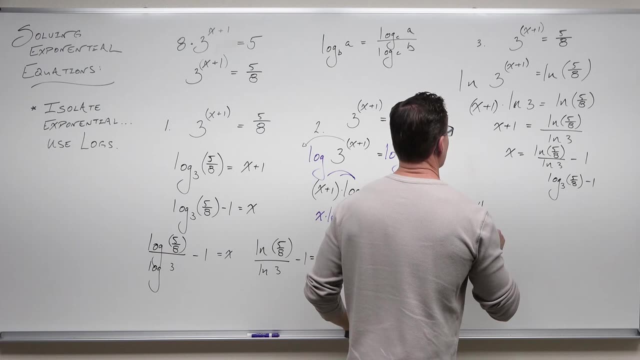 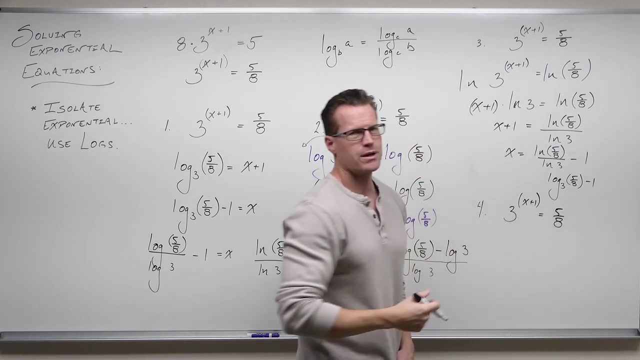 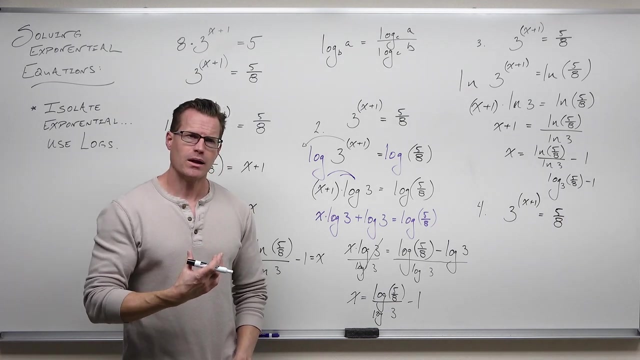 that one. So they're all equivalent. They just look a little bit different. They're all valid. Pick it whatever you want. Now the last one. We already know we can do a logarithm on both sides of an equation, provided we actually do it to both sides, And we also know that, like an ln. 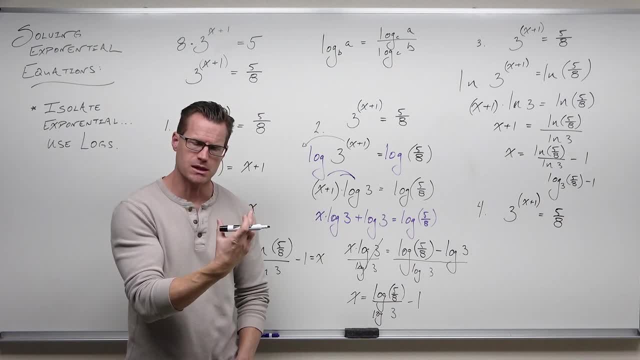 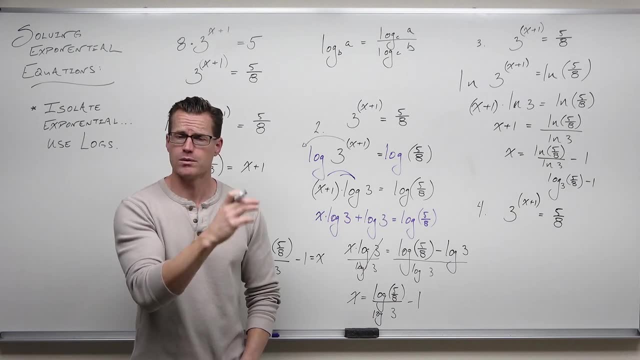 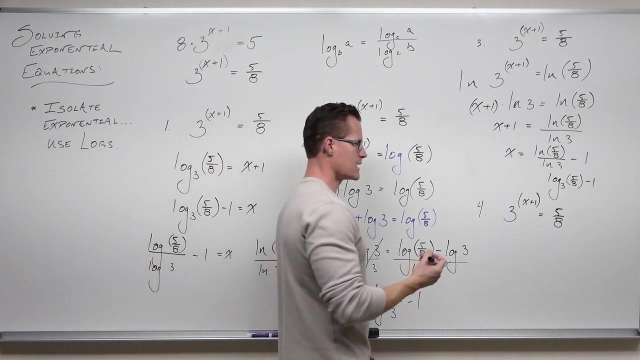 composed with an exponential base e, or a common log composed of an exponential base 10, simplify it, Because if naturally compose an exponential onto its inverse, which is a logarithm, then that's great. Well, can we make that happen here? What if we took this and said: you know what? 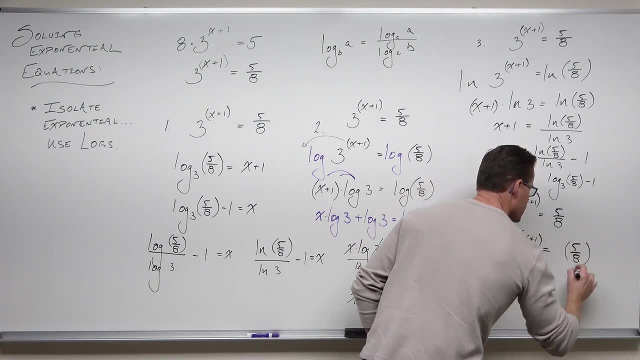 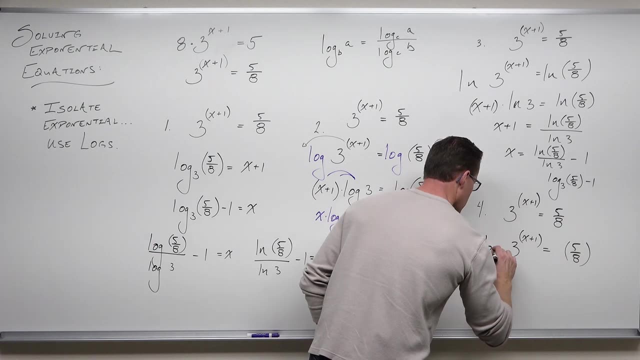 We know about logarithms and exponentials being inverses. What if I took a very specific logarithm? What if I took a log base three? Now, why would I want to do a log base three? Notice, you have to do it on both sides, But if you do, 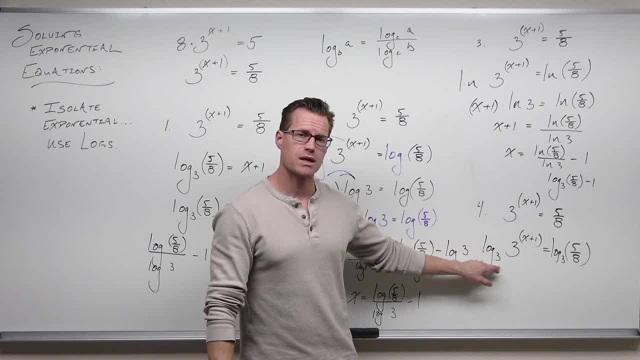 log base three of three to the way. wait a minute. that's a logarithm base three, an exponential base three. You compose a function on its inverse. They will cancel out. They will give you the exponent. You could move the exponent. 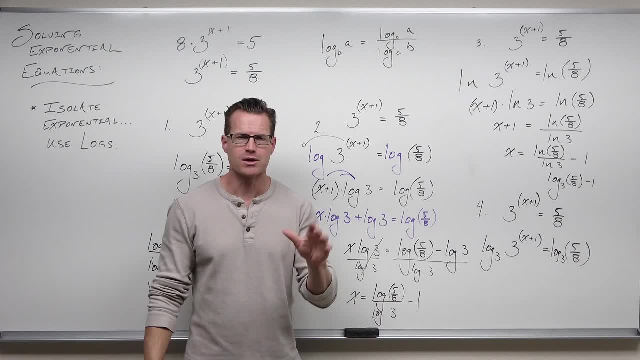 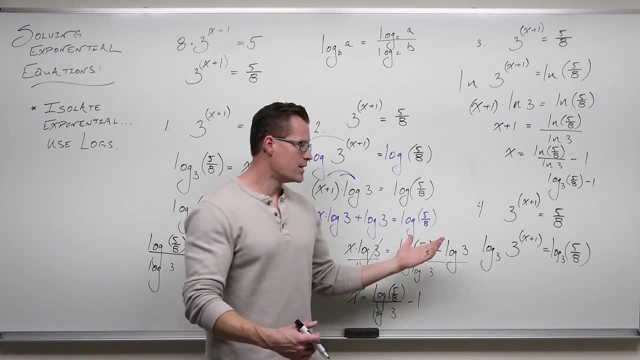 to the front And you'd get a one there And you go: oh yeah, I remember that property, Do you remember it? Log base three of three to whatever power you have is the power that you have. That's what we're doing right here. This: no matter what you do, you're going to get just x plus one. 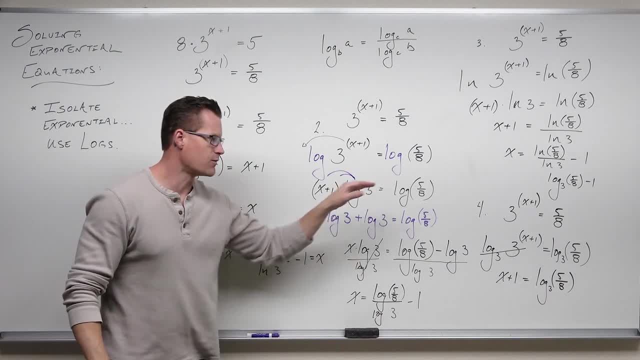 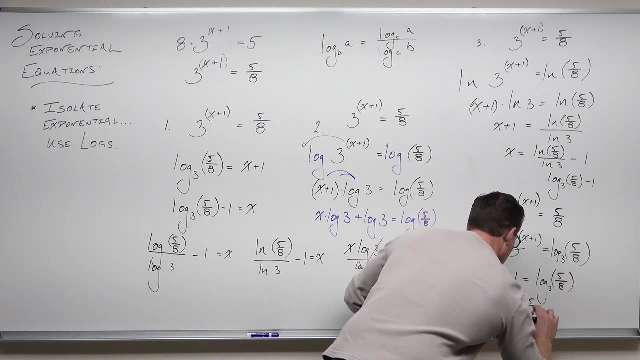 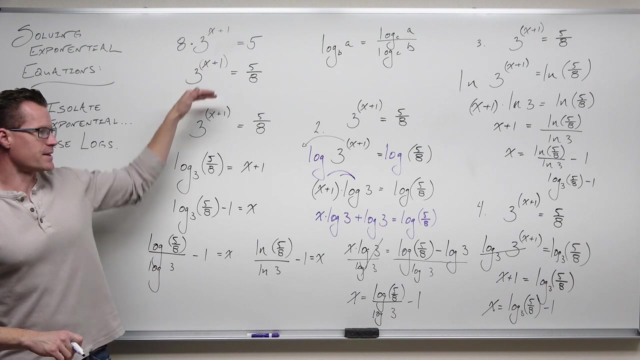 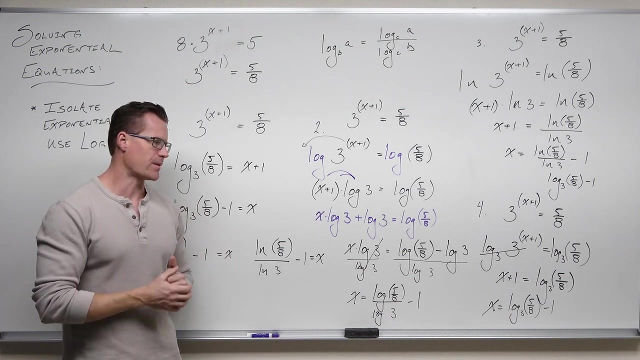 So if we subtract one, we get the same thing we've got every other time. This really is the same as writing this as a as logarithmic notation. It's just showing a little bit of more work. Either way you go, it's going to come out the same. Preferentially you'd probably. 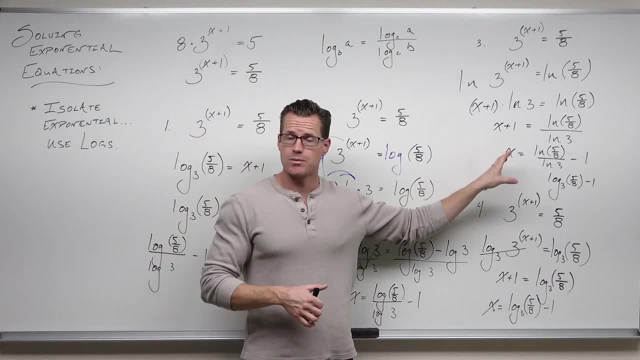 pick a common log or a natural log, So if we subtract one, we get the same thing we've got every time, Because that would be very easy to evaluate in your calculator. This one, you'd have to change your base, would you? You'd say, hey, I want a log base ten or a log base e, And write this as: 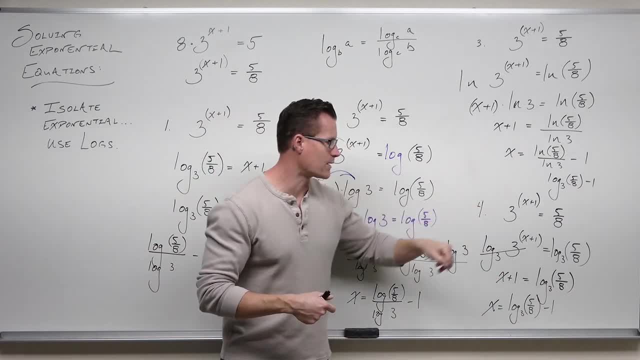 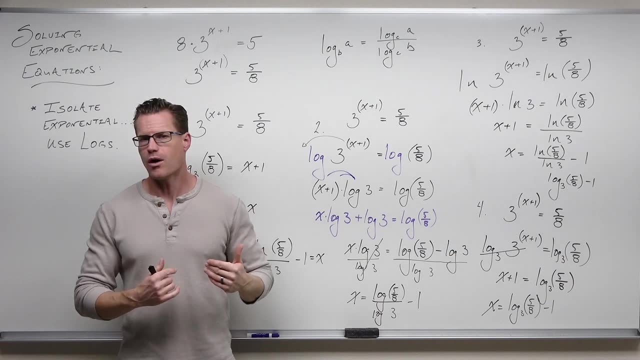 ln five-eighths over ln three. Exactly what we had right there, minus one. So I hope I've made that make sense. These are the four options that you have to solve a basic exponential. Now we're going to move on And this one's going to fall off the map, And so really is this one, Because 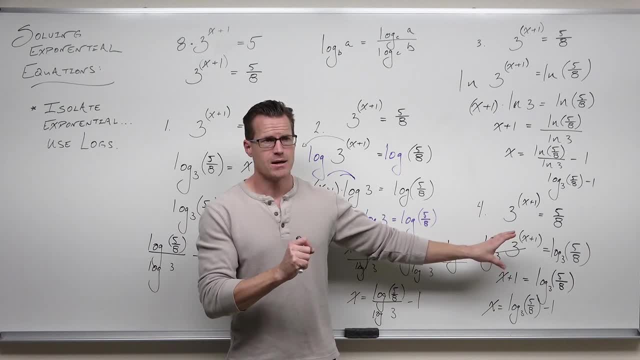 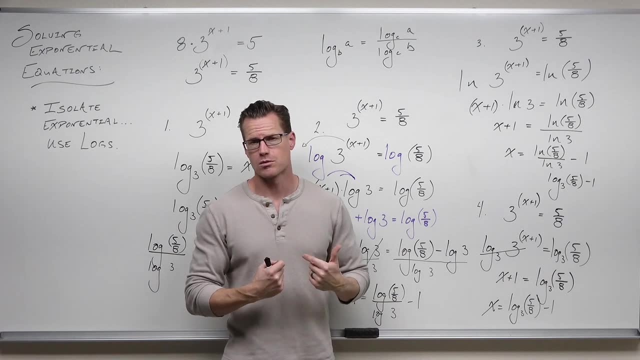 both of those deal with a very specific base. What if I have two bases? Well then, it would benefit us for one exponential but not the other, And so we typically pick a natural logarithm to do this, Or a common log in some cases, But most of the time just a natural log. So we're going to come back. 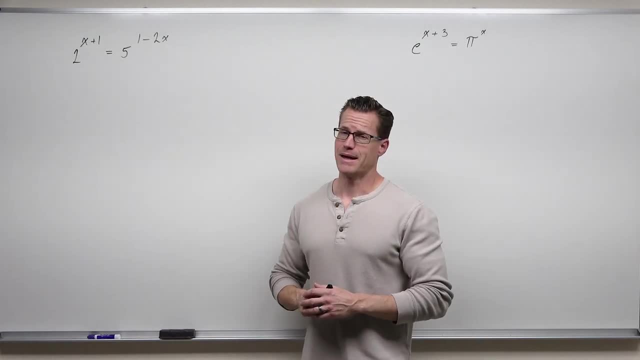 with a couple more examples and show that. All right, Now I'm not giving you a whole bunch of examples in this video, I'm really giving you only five, And one of them like four different ways. But these next two are going to illustrate a lot of different examples, kind of in one A lot. 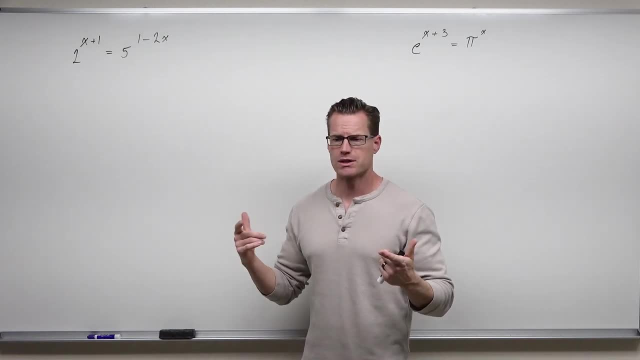 of different examples. look like one of these two, And the reason why I'm only giving you a couple is really there's not much else that doesn't fit into one of these categories. There are some substitutions, And I'm going to give you the next two examples, But if you're going to solve some, 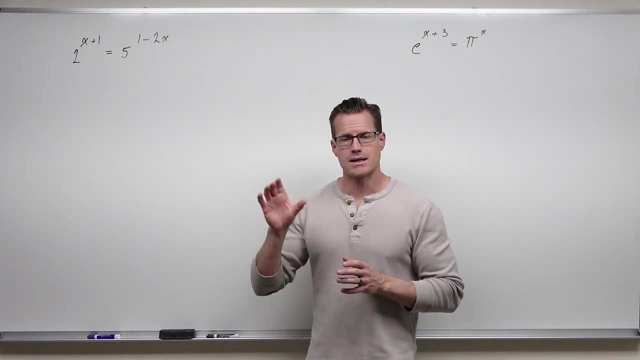 exponential equations there's typically those you can isolate on one side And then do what I just showed you in the previous example, Those which have two exponentials but have a common base, which I showed you in previous videos, Or those which have two exponentials that don't have a 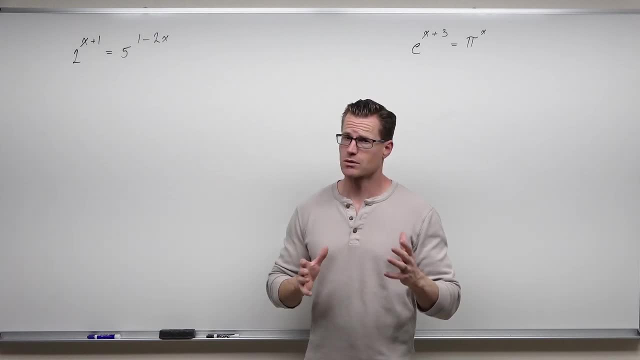 common base. That's what we're dealing with here. So we have two exponentials. They certainly don't work. You can't write a five as a two. You can't write a five and a two as some other base. So 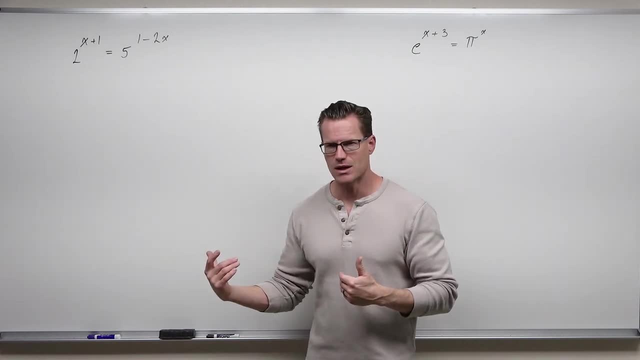 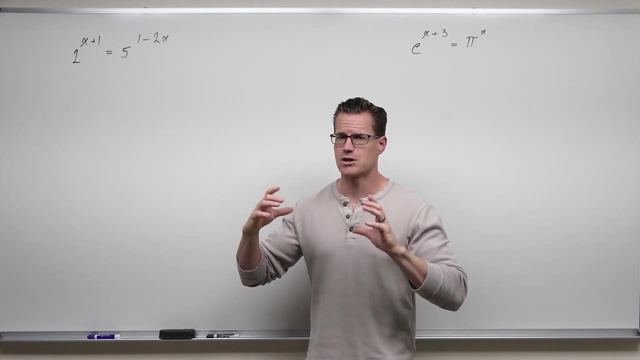 that's off the table. Also, we have an inability to isolate an exponential here, Like we have two of them, So we can't get one of them on one side and a constant on the other side, Which is why the first technique I taught you in the last example is not going to work here. You can't write this. 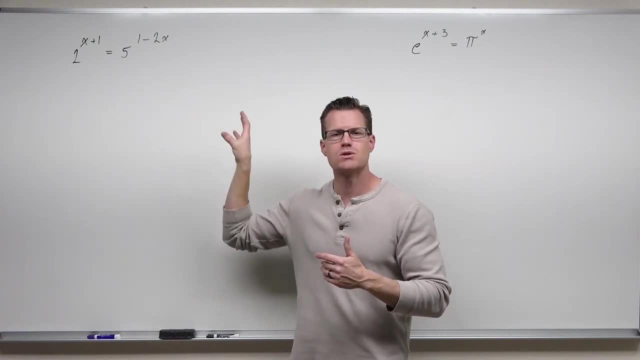 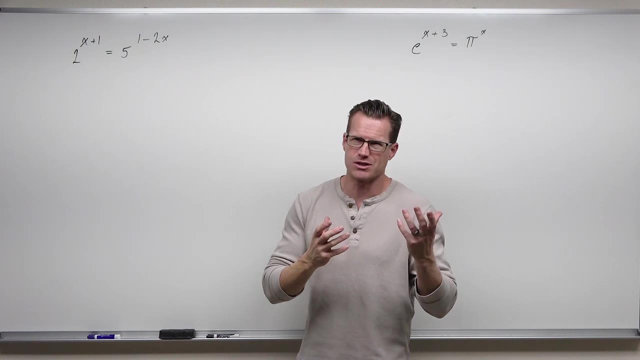 as one logarithm with one base, with two different bases. That's not going to work. So we're on to the next example. Could we choose to do like a log base two on both sides? Yes, you could, But what's going to happen is you'll end up doing a change of base later if you want to approximate. 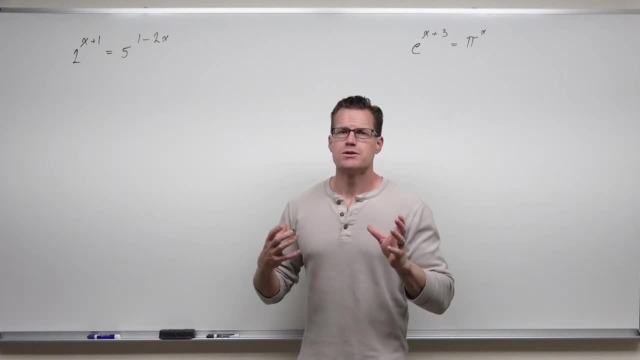 it. So I'm going to give you one of do one of two things. Choose to do a common log on both sides or a natural log. I'm always going to do a natural log because I prefer it Also when we. 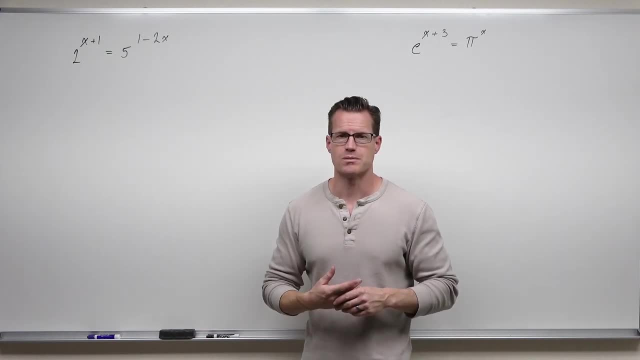 see in the next example, natural log is really nice when we match a base with a base. Now you have done that here, but we deal with some other issues if we end up doing that. So not hard issues, but issues. Maybe I'll show that to you in just a bit. So let's take a look at it So. 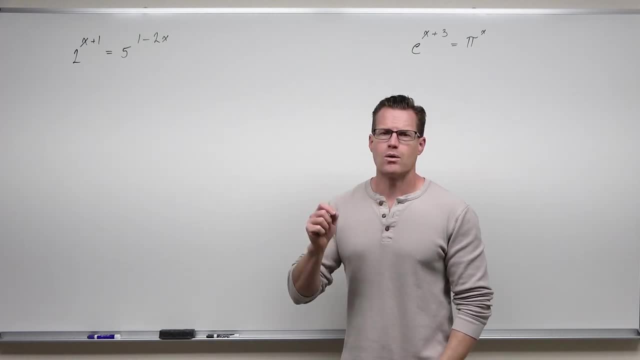 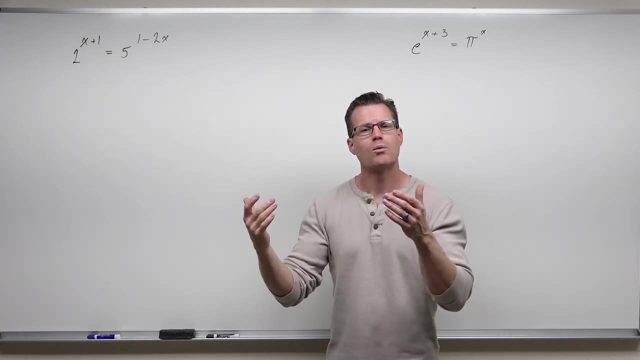 it's got two exponentials. We don't have a common base, We can't isolate one. The only way to solve exponentials like this without common bases are to use a logarithm, And we're going to apply a logarithm on both sides. We're going to pick a natural log, So an ln on both sides of this. 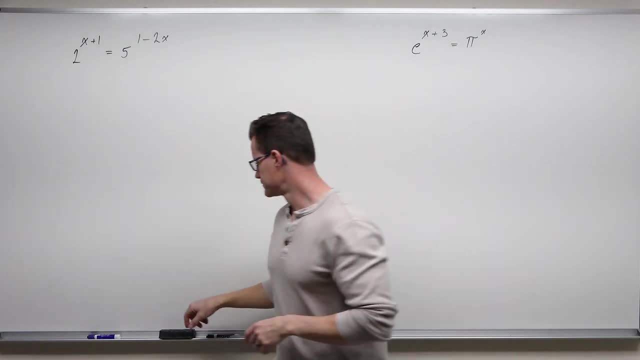 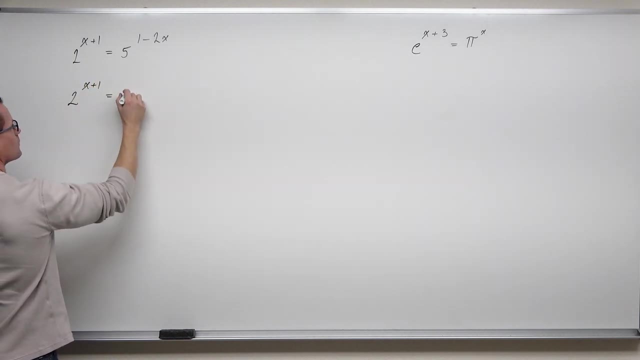 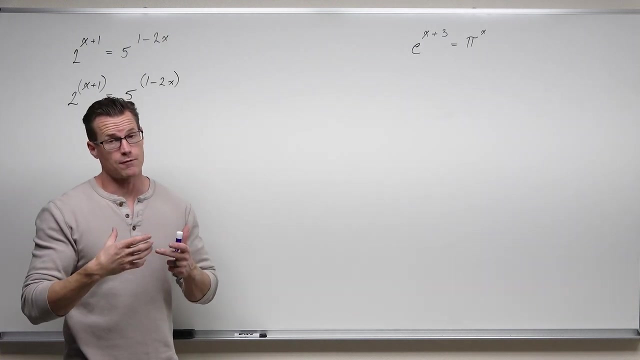 equation. What's going to allow us to do is move our exponent to the front. So right, here is also where I always write parentheses around that exponent. Why? Because I know I'm going to move it, And if I have them now, I'll be able to move it later. and not forget. 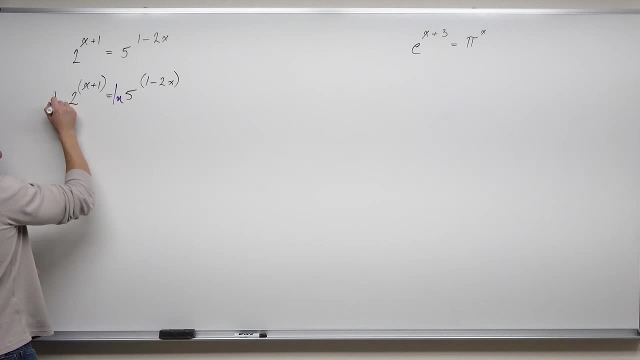 them. So I'm going to do a natural log. It's got to be on both sides. You don't have an option here. Once you do the one side, you have to do the other. But once we've done that, we change an. 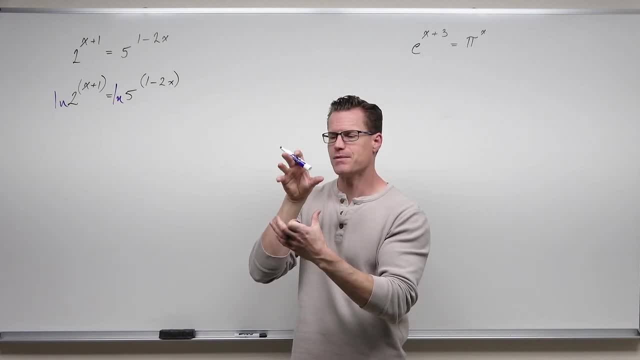 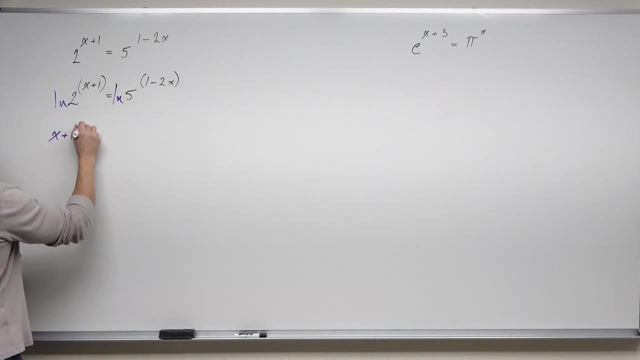 expression, kind of into a logarithm. It allows us to move by the power property, these exponents as coefficients, as products, next to a logarithm. I've done a mistake on purpose. I want you to see it. I see this a lot when I'm grading tests and things like that. I see students who do this and 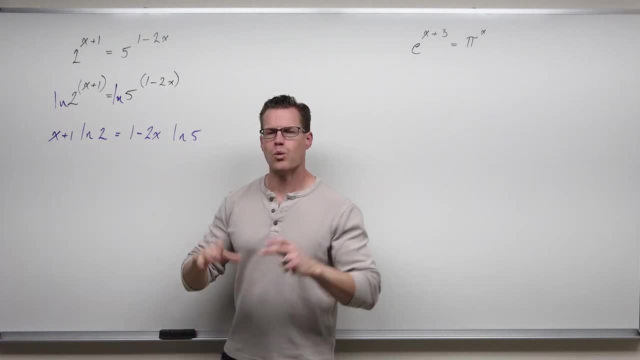 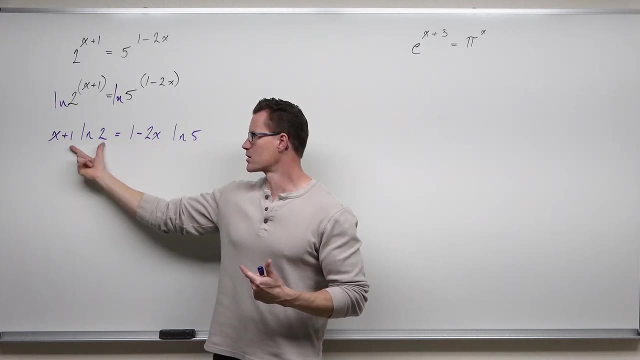 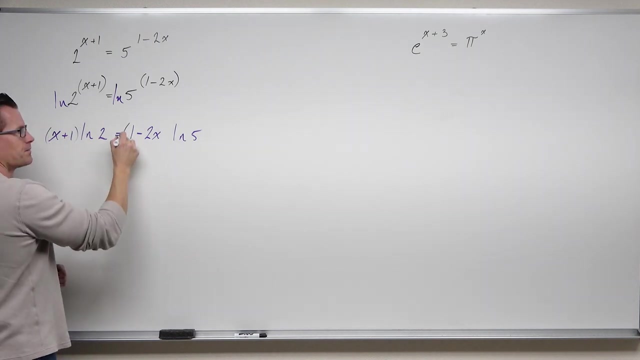 understand the property, They really get it, But then they fail to do one little thing and it leads to a problem. You see how, if I do this, this looks like a term and this looks like a term and it's not. There's a product here. This is the case, if I write it correctly, where you must distribute. 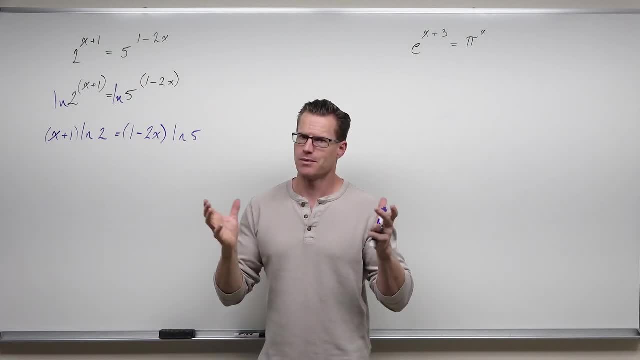 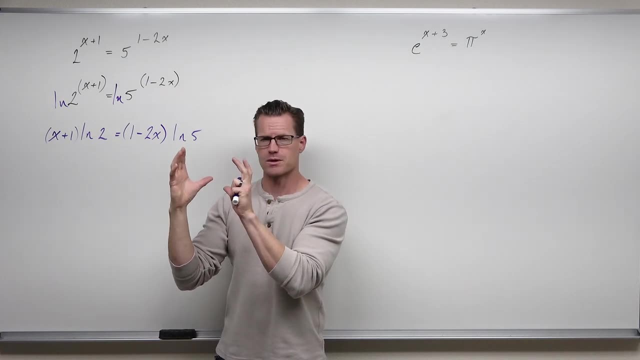 I hope that you can juxtapose this with the previous example where I said: oh, you might have to, you might not, But look, if you have x's in any other place beside this one, right here, beside one parentheses, one parabele expression. if you have them anywhere else, you must distribute. 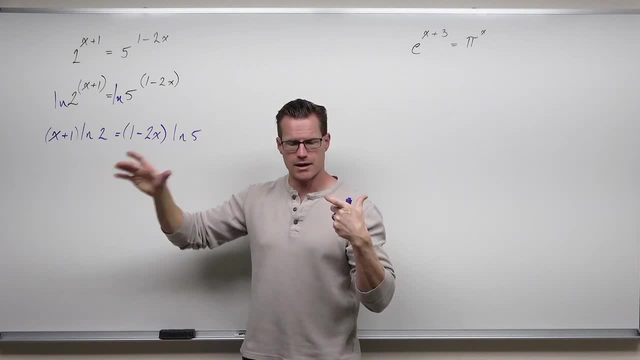 Get your x terms on one parabele expression. If you have them anywhere else, you must distribute. Get your x terms on one side, your non-x terms on the other side, factor this side and then divide. So that's our necessary process for solving these. There's really not another way to go about. 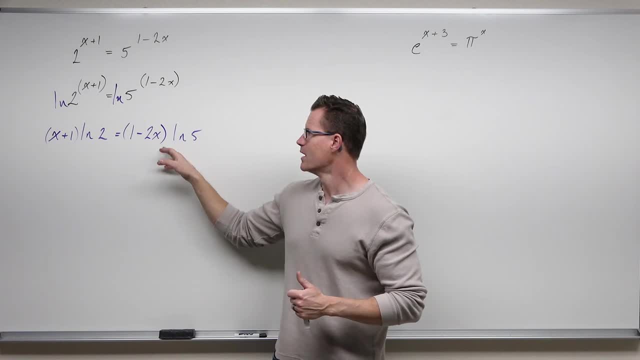 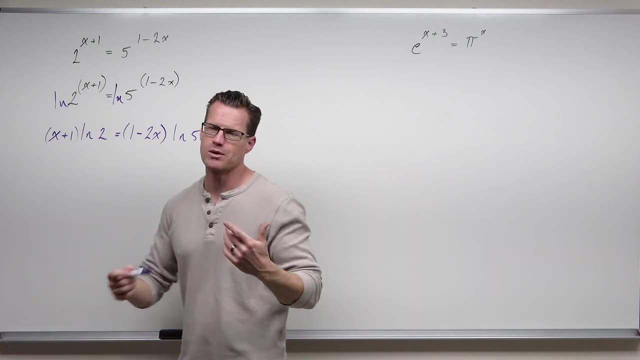 doing it because x's are in multiple places. If we just start dividing here, we're going to make this side even worse. So distribute everything right now. That's why we put the parentheses and that's why we're noticing multiple x's, so we can make that judgment call. 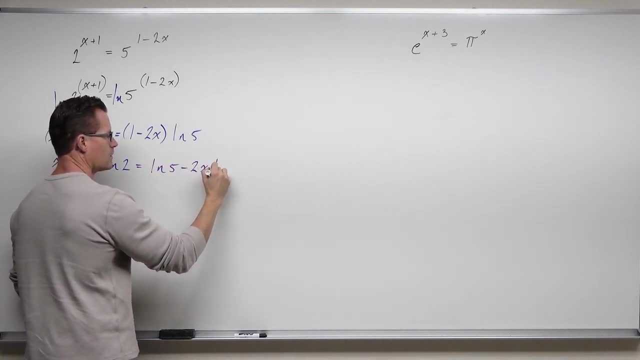 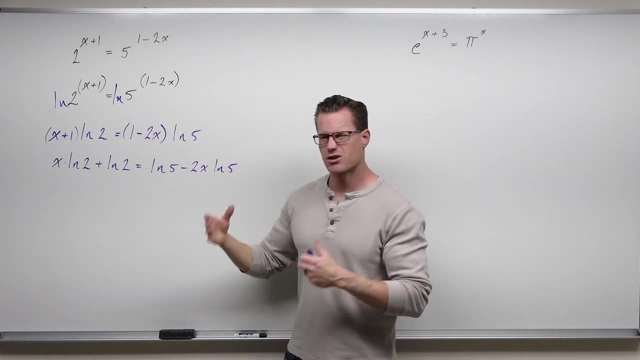 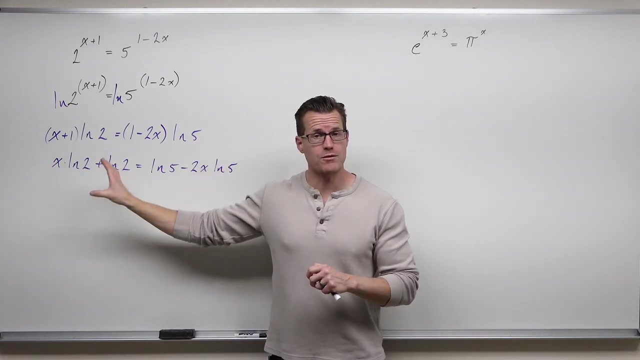 So we've distributed. We know that we can distribute ln 2. We can distribute ln 5. We're kind of doing backwards distribution, but it doesn't really matter. And now we're noticing that, hey look, there's one, two terms with x's. We need to group those so that we can factor. 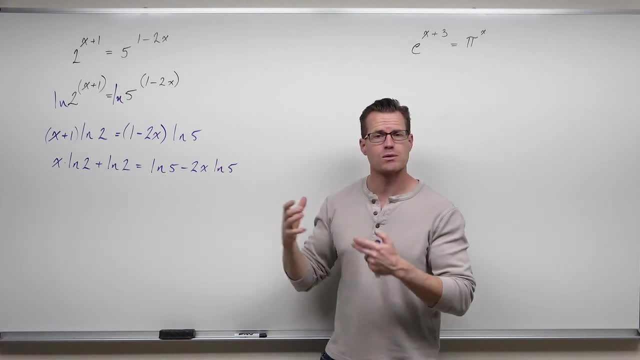 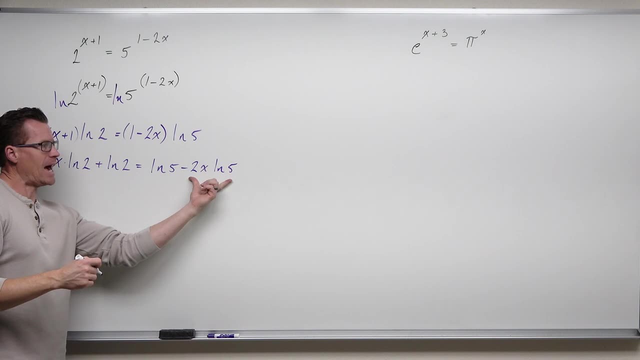 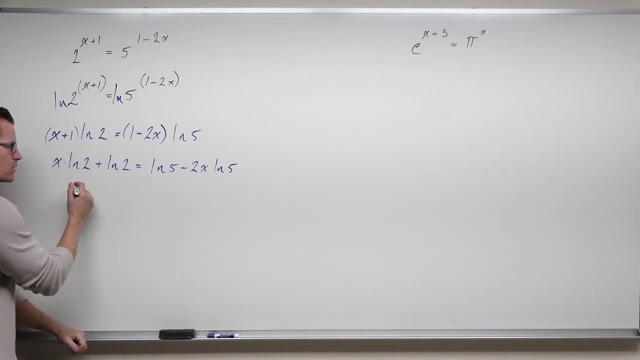 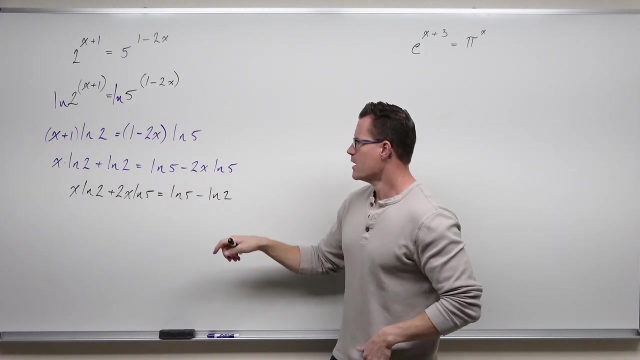 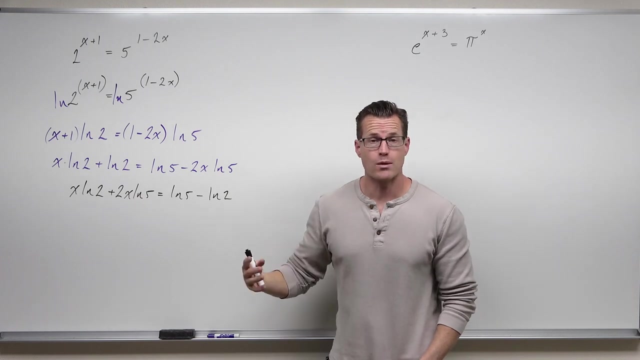 add two x's, ln 5, and subtract ln 2.. We're going to watch our signs, be real careful. It's really easy to make sign errors when we're moving terms around. So I've added two x's ln 5.. I've subtracted ln 2.. My other signs look pretty good. This is why we want to do it. 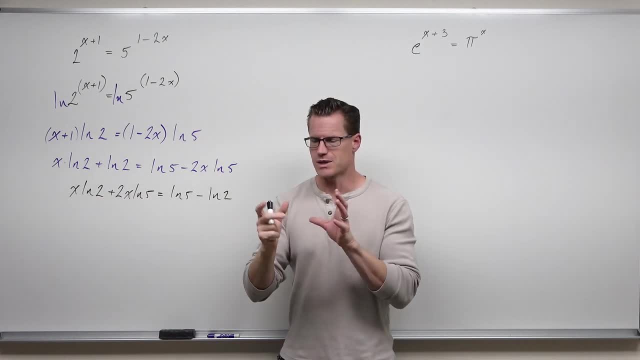 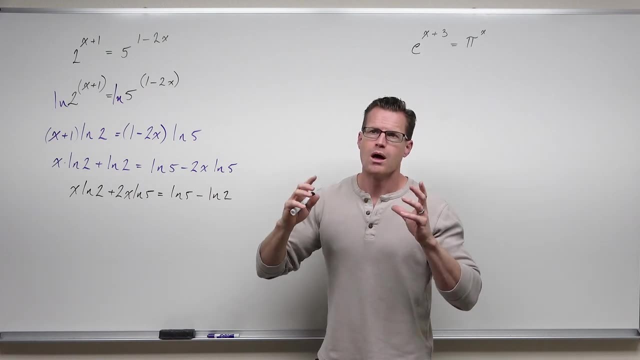 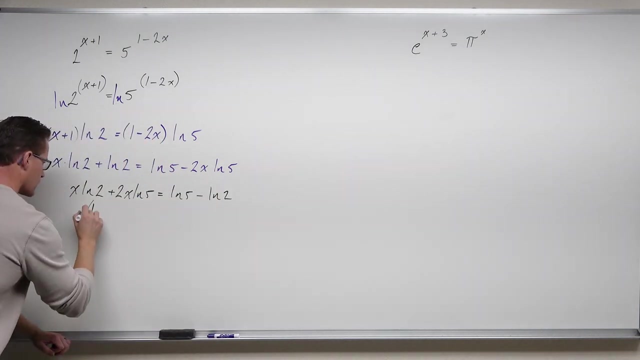 so that we can group our x terms, Grouping x terms: every term that has an x in it. we can factor that. x Terms that don't have x's don't need that, so are on the other side. So we don't have to worry about factoring something they don't have. So factor in x, we factor x, and 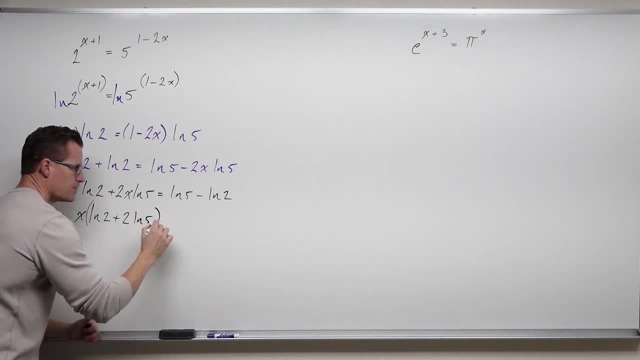 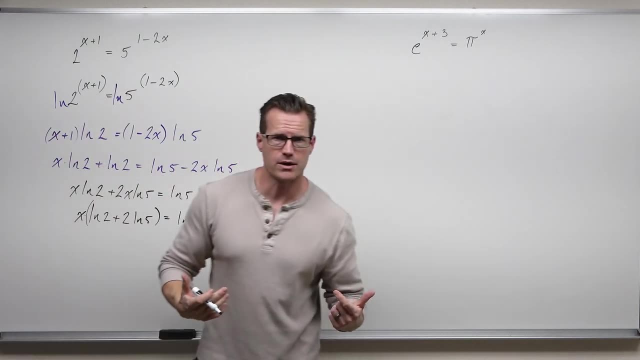 get ln 2.. We factor x and get 2, ln 5.. This is great. This is exactly what we want, because what it does now is it creates a product for us, And how we undo products is with division Before that. 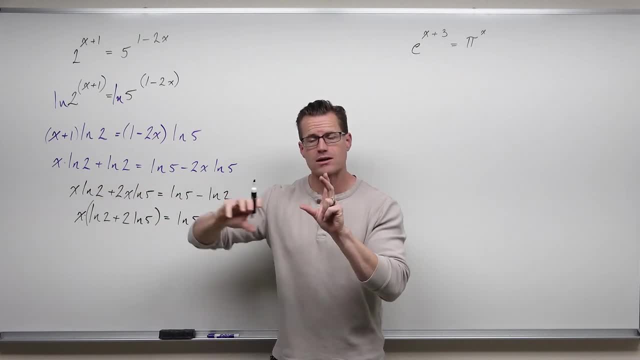 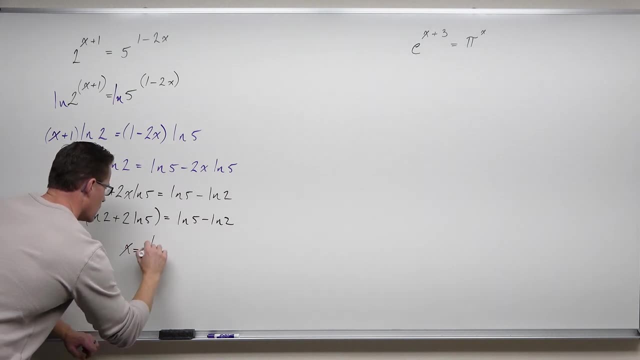 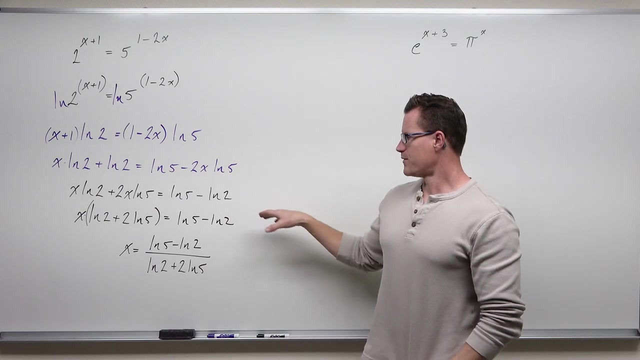 we had two x's and we couldn't really divide it. It wouldn't be relevant. But now that we have that factored version of it, we can divide both sides by whatever that expression is. So ln 5 minus ln 2, all divided by ln 2 plus 2 ln 5.. It's pretty wordy. That's lots of ln. 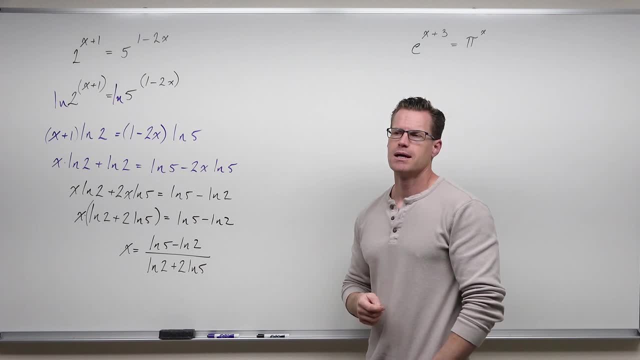 so this is probably going to make sense. Can you see it differently? Could you see it differently? Yeah, you really could. Now, this is perfectly appropriate. You can do this, This is approximatable, But I do want you to see that there is some simplification possible, For. 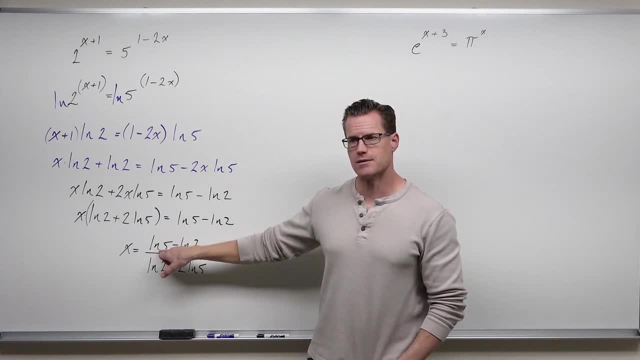 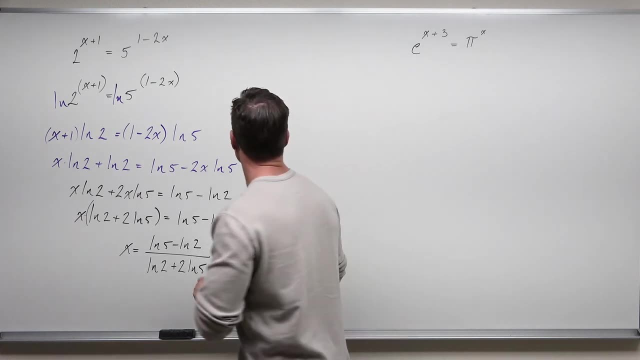 instance, can you combine two logarithms with the same basis if they are being subtracted? Yeah, of course You can create one logarithm, the same base, with a fraction or a quotient inside, So you actually have a plus sign in the back. So again, when we need to divide by a minus sign, 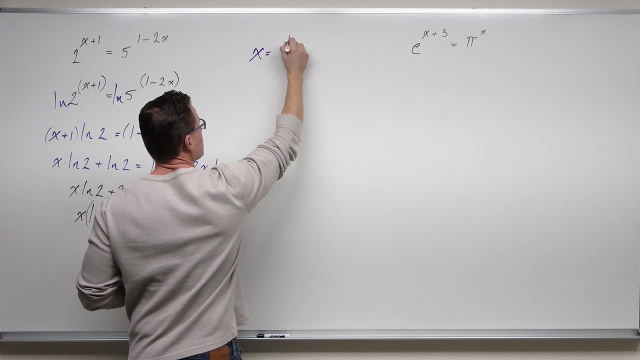 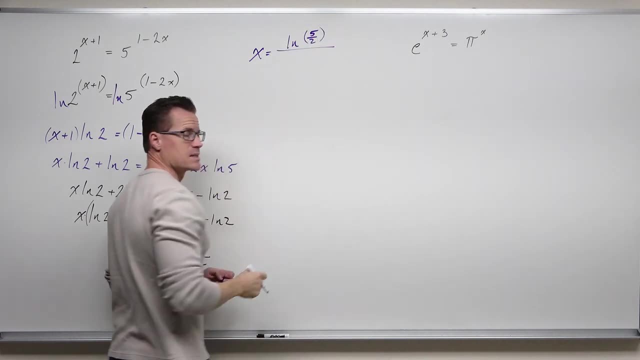 we can add a minus sign on top of the minus sign. We use the same approach here, So we can do that as well. Now let's go over here. How do we do that? By changing the lowercase, it, andGEI, So 5 over 2, inside of a logarithm. 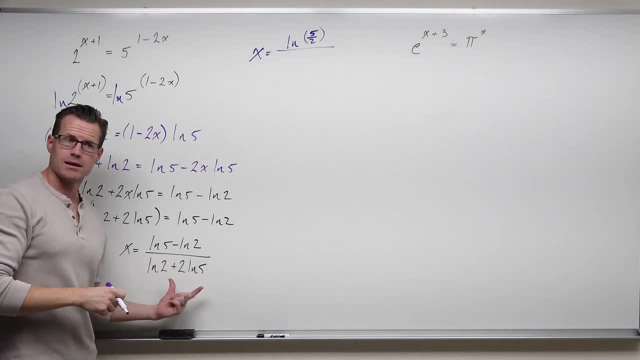 On your denominator. can you combine two logarithms being added if they have the same base? Yeah, you can, but you'd have to move a coefficient as an exponent. so wait a minute. This is ln 2 plus ln 5 squared, if you move that as an exponent. 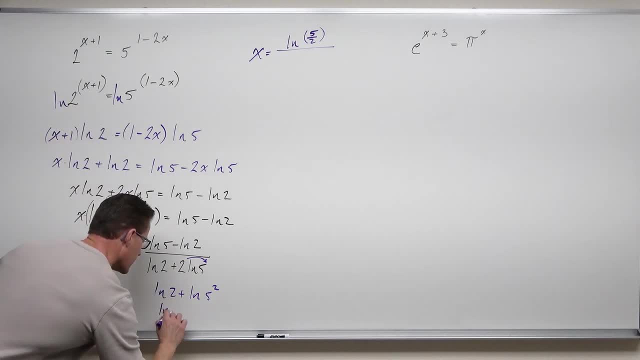 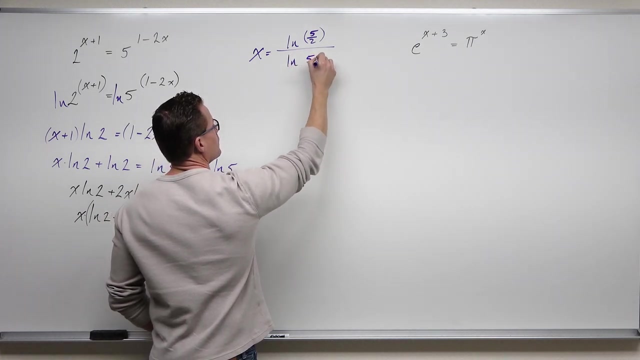 That's ln 2 plus ln of 25.. How do you combine two logarithms being added with the same base? Well, you multiply that plus creates a product inside one logarithm, so ln of 50. You can see that. you can certainly see that you can even have a 2.5 there, but you can. 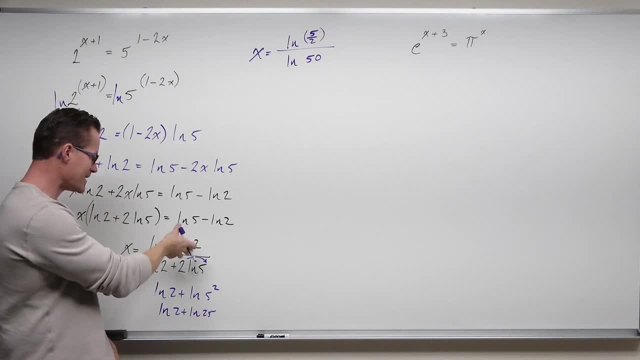 certainly see that in the back of the textbook, because they combine all this. Now, if you've got this and you look at that clearly, you're going to go. oh, that's a mistake. No, I made a mistake. 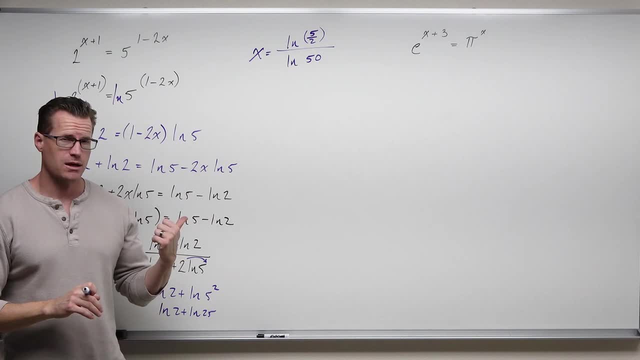 You haven't. They've just combined some things. In fact, we can do one more Now. I would leave it here because that's easiest to approximate on your calculator. It's going to basically be: you've got an ln button, that's great. 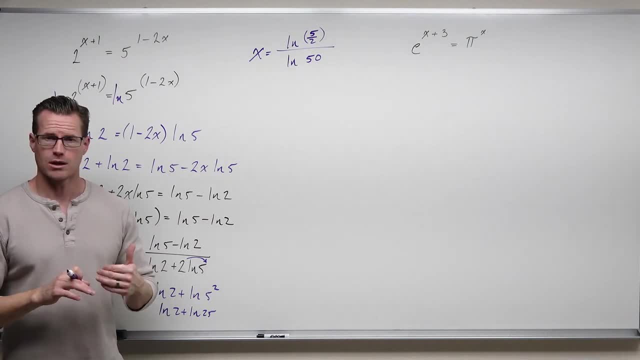 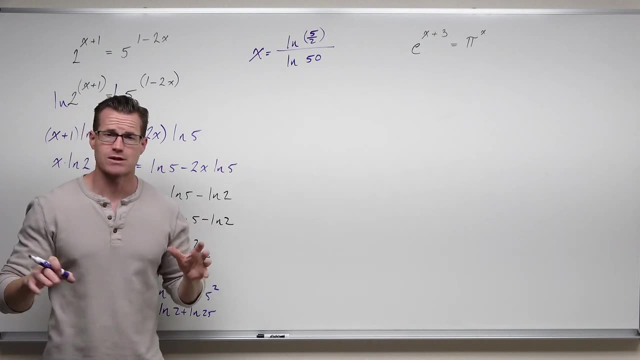 Notice something. I'm going to pause right here and just say this: Could you have done a common log and just put log everywhere and got the same thing with log and log? Yes, absolutely, and it does not make a difference. 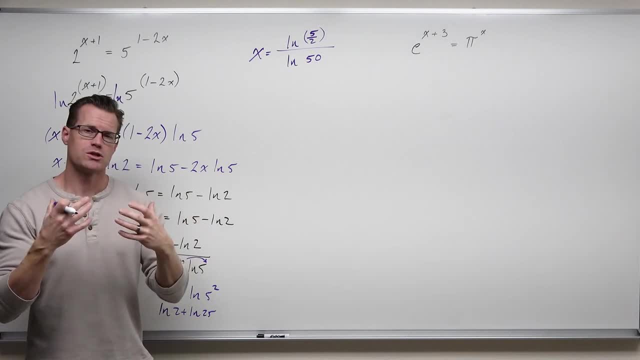 This is why I'm not showing it to you. I'm not going to repeat this. the same steps, with just that word log. That's fine. What you could do, though, here is, because you have the same logarithm, you're going to 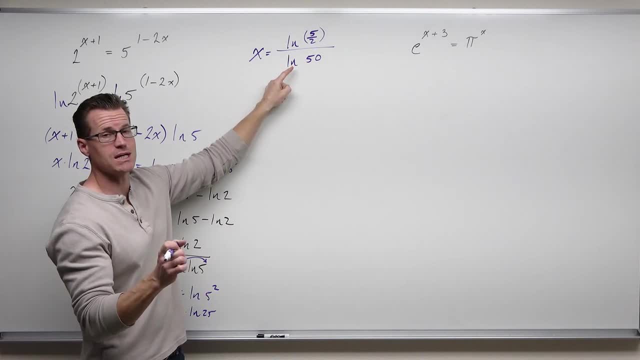 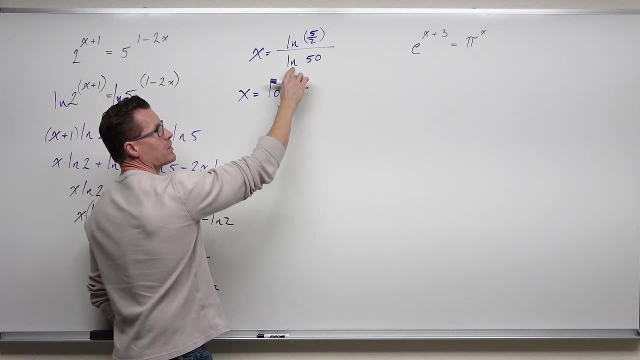 have a common log. That's fine. You have the same base in a fraction. I'm hoping you see it. Do you see that we can use change of base in reverse? We could really write this as a log with a base of 50, and a new argument of 5 halves. 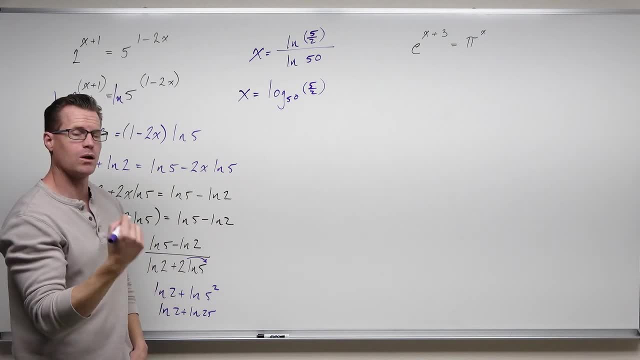 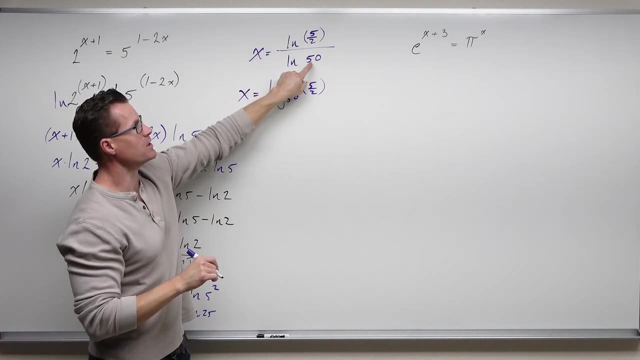 Now I don't know if that's better or worse, but that is one logarithm. Notice it's not ln anymore. You changed the base. You said these have the same base of e. I can combine this, make this my new base and my new argument and create one logarithm. 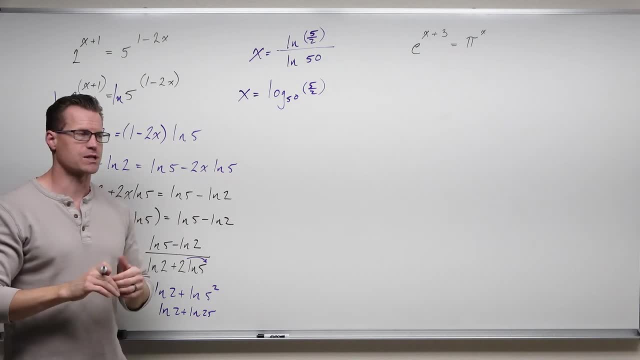 That's as concise as we can make it. There's nothing better that we can do with that, as far as I know. Now I did say there is another way to do this. You'll see that you have to do a change of base somewhere or you end up with something. 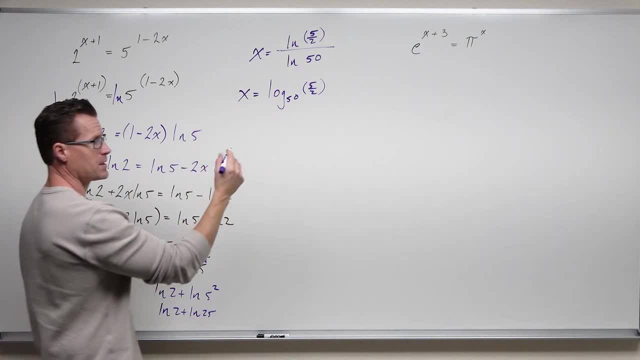 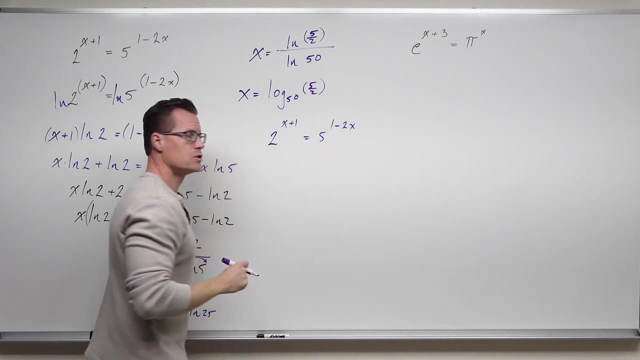 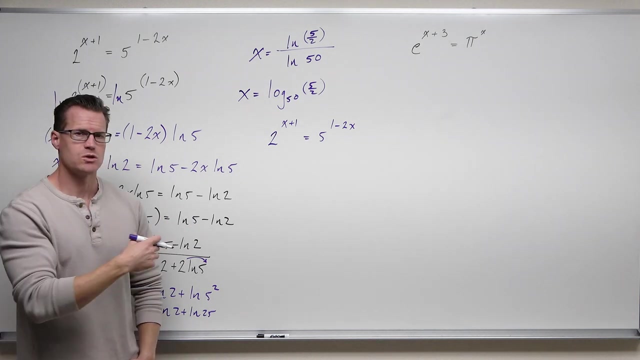 just like this. So approximate might not be the best, But from here could you choose a logarithm with a base of 2, and a base of 5, and get the same thing? Yes, you can, I don't care which base you choose. 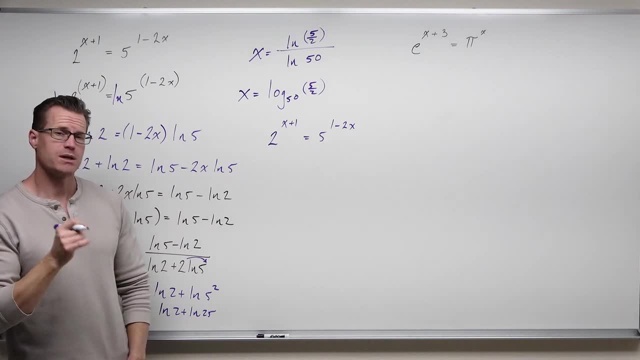 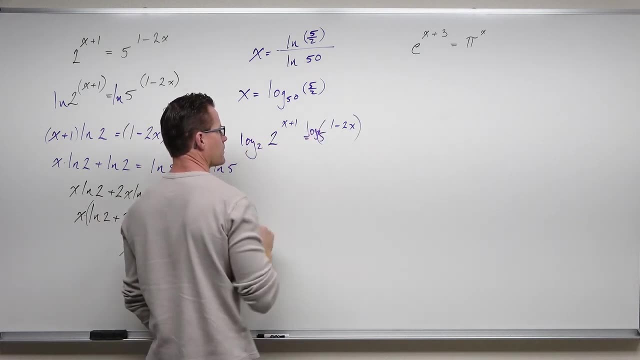 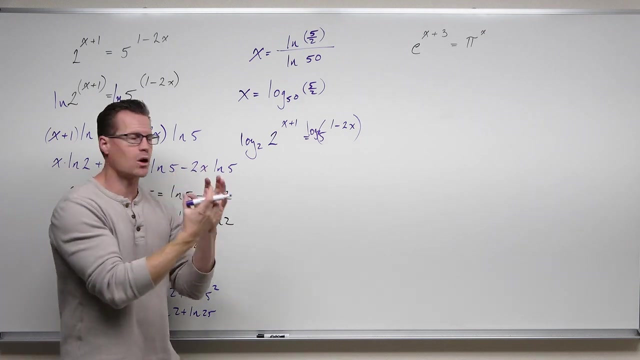 It's kind of a whatever you want to do in it. But if we did, let's take a log base 2 of both sides. So on this side, notice what happens. This is the important side for you to see. If you choose a log base 2, you inherently match a logarithm and an exponential and compose. 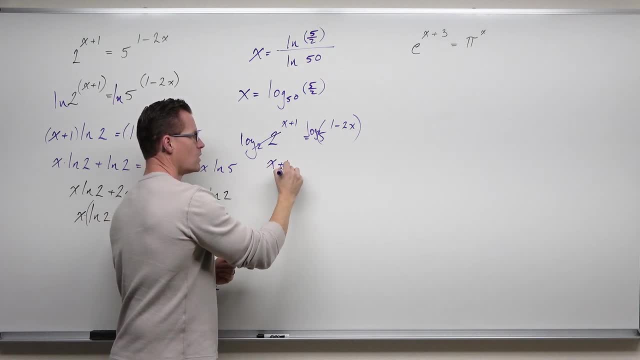 a function with its inverse, and you are going to get x plus 1.. On the right-hand side, though, you have log base 2 of 5 to the 1 minus 2. That's the same thing. That's the same thing. 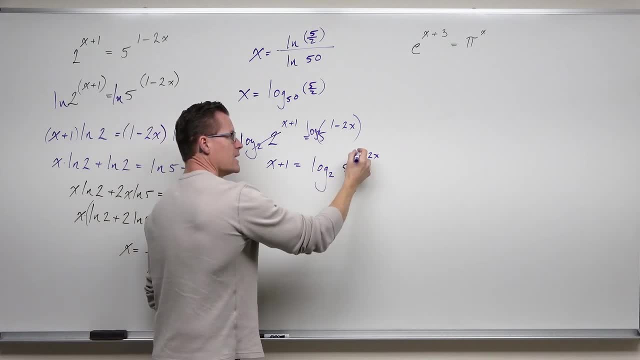 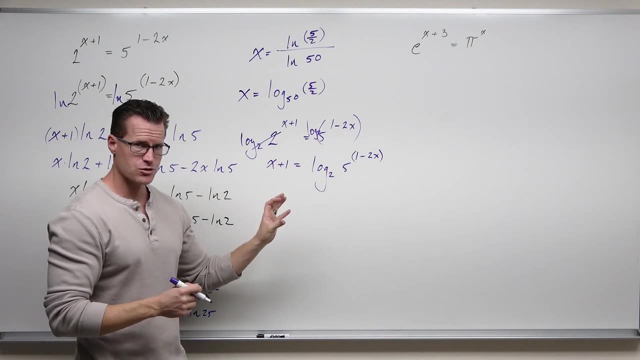 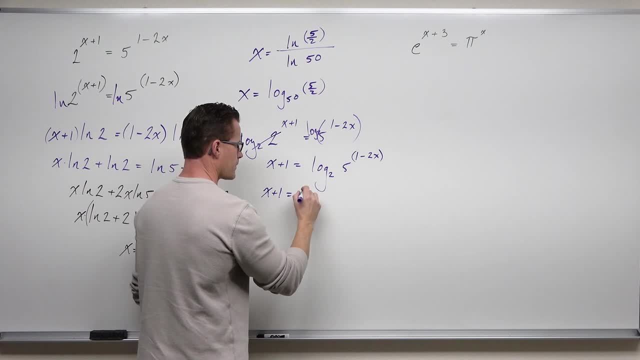 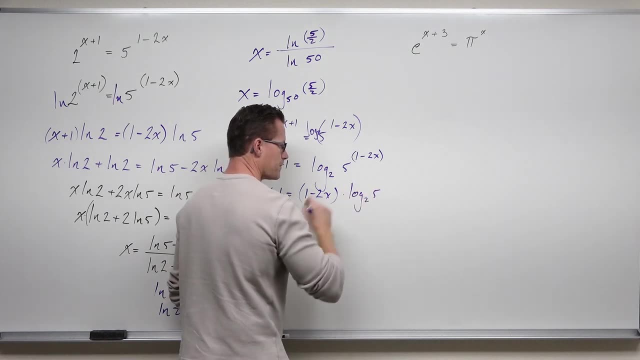 and dividing. I wouldn't say it's better or worse, It's just different. Now do you have to distribute? Well, I just said you did, But the reason is because you have an x here and x here. Actually, you must distribute this. 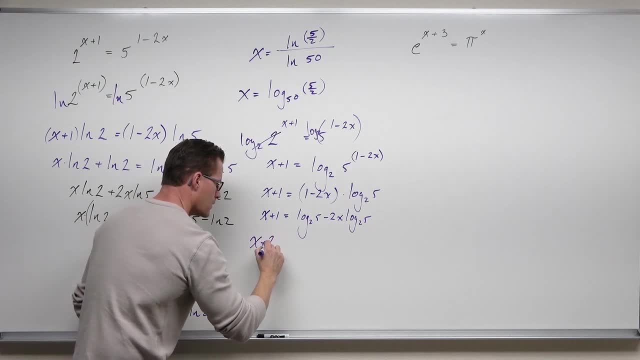 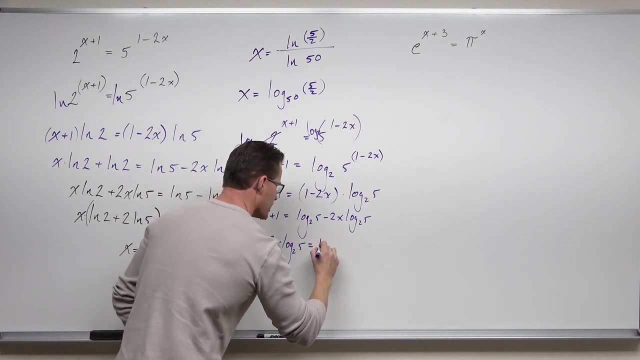 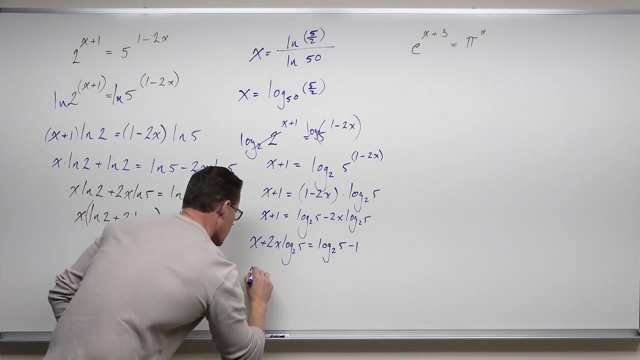 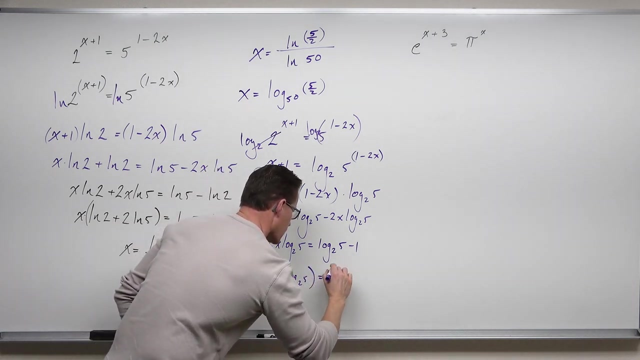 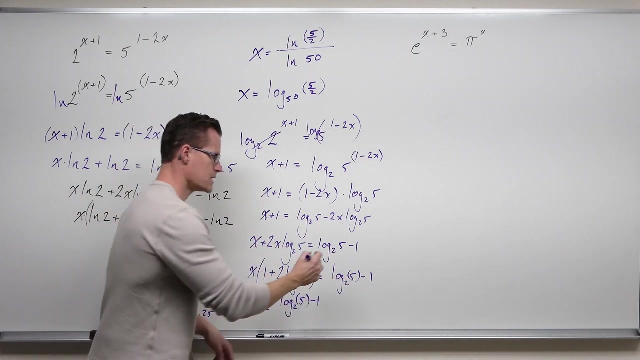 We've got to collect our x-terms and our non-x-terms. So adding and subtracting, respectively factoring and then dividing. I'm keeping this five in parentheses so that I don't accidentally subtract that one. That would not be good. 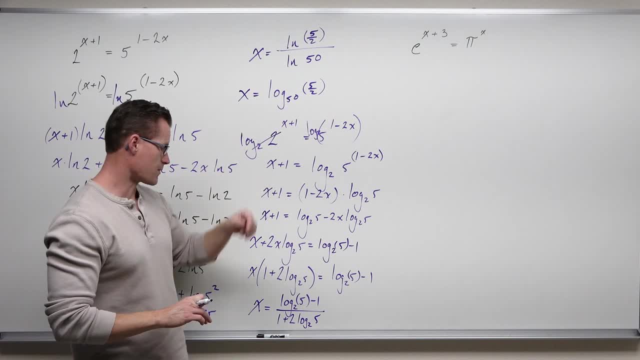 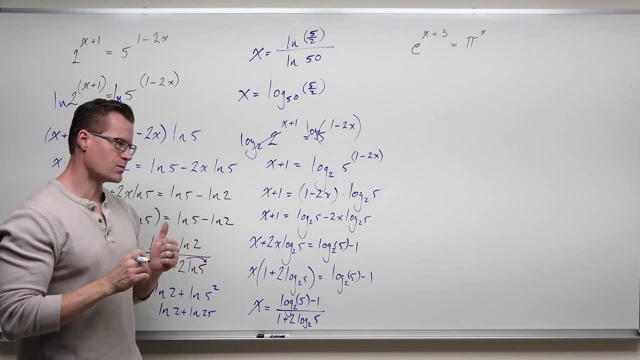 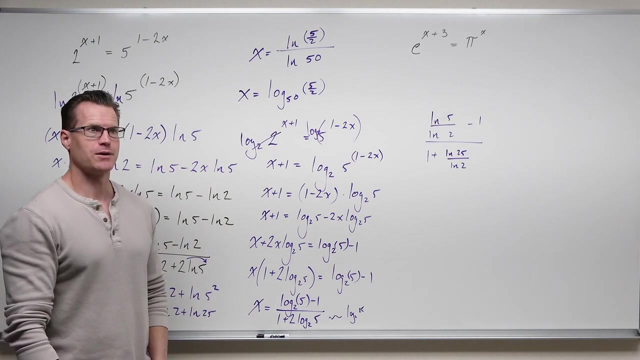 Now that looks decidedly different as what we got right there. Is it the same thing? Yes, but it might take a while. It might take you some work to actually see it. I hesitated for a second because I didn't know if I really wanted to show you. 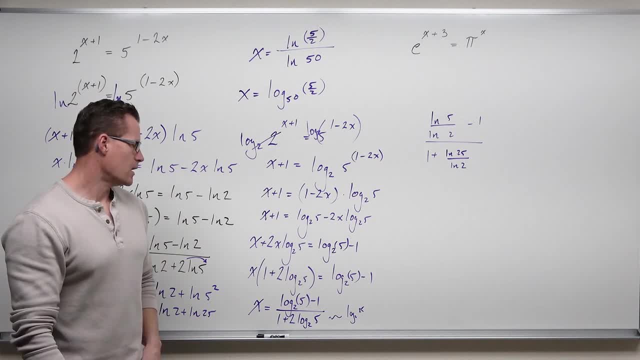 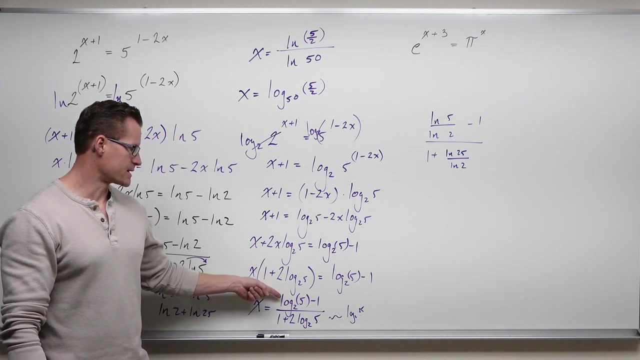 but I do, because I always do Every time, darn it. Look, if you change this to log base 2 of 25,, so move that to x, so we get log base 2 of 25, and then you can write this as ln 5 over ln 2,. 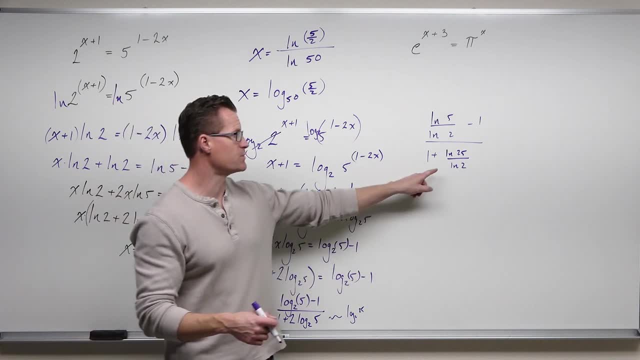 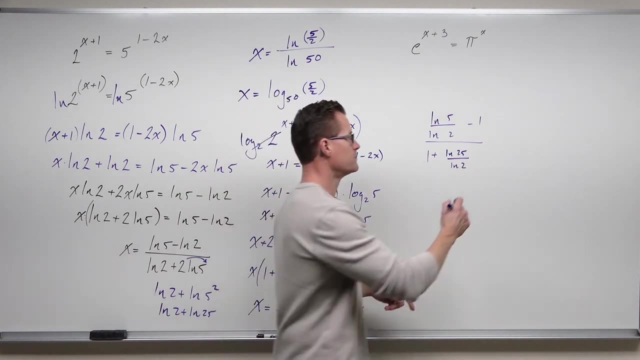 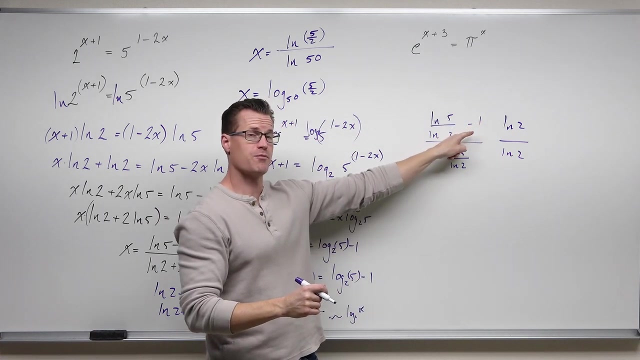 change of base and ln 25 over ln 2, change of base. Do you notice that your LCD of ln 2 on this complex fraction you can multiply ln 2 over ln 2.. It would distribute Cancel here and get ln 5 minus ln 2.. 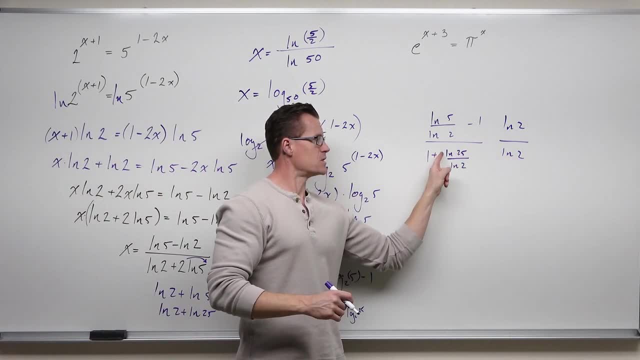 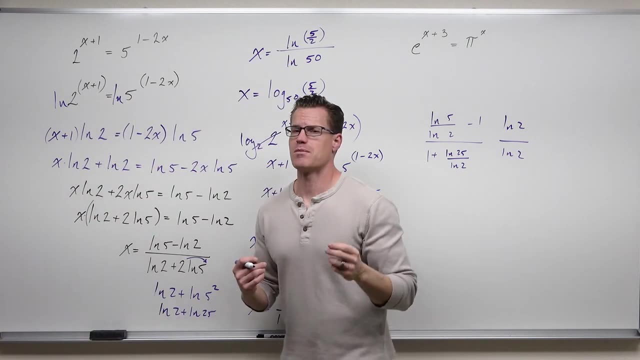 That's that It would distribute here. That'd be ln 2 and cancel ln 25.. Here's ln 2, and this is ln 25.. So it is the same thing, It just looks decidedly different, Way, way different. 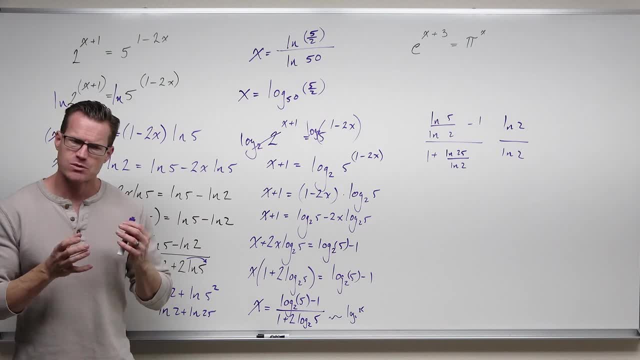 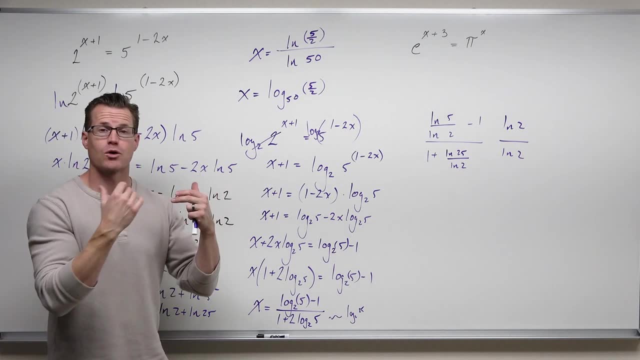 And that's one thing you find out with logarithms- is that sometimes what you get can look fundamentally different from someone else's answer. And they're both right, Because there's lots of different techniques that are equivalent, Lots of different properties that will do the same desired effect on this. 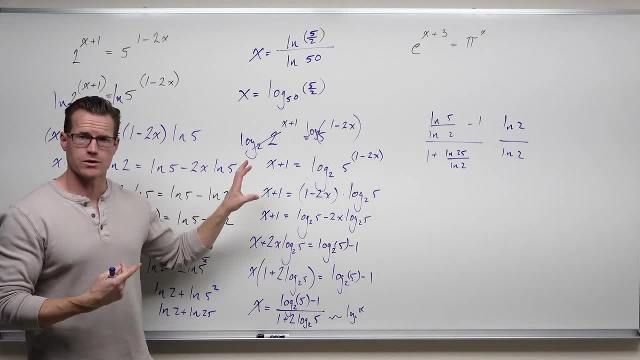 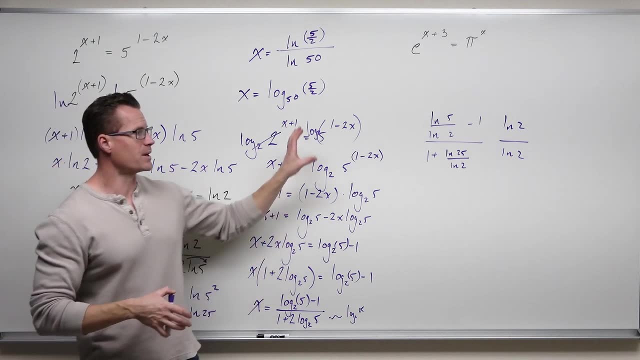 And so don't really worry about it. As long as you follow an appropriate technique- what I'm showing you here, one of these two things- you're gonna be fine. I hope that makes sense to you. I hope that you see that we can get a different look. 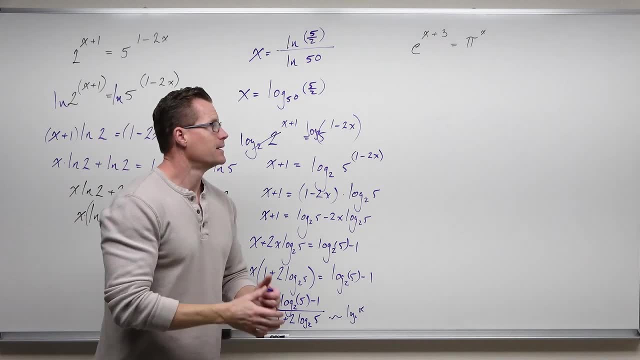 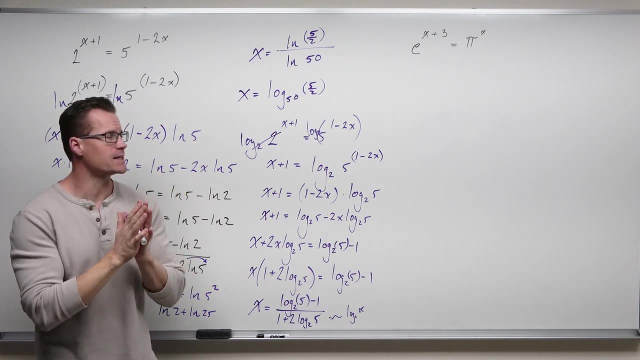 but it's still exactly the same thing. All right, we're gonna move on to the next one before we do our substitution. So we have e to the power of one, e to the x plus three equals pi to the x. That looks kind of crazy. 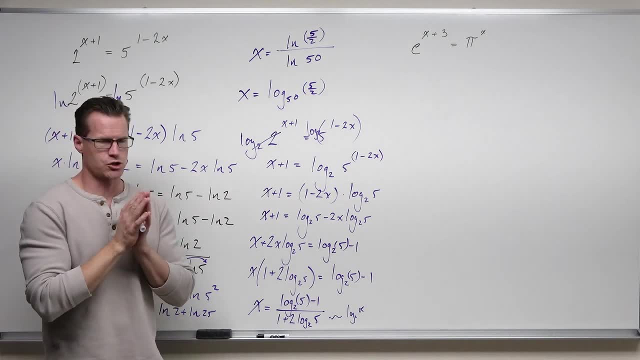 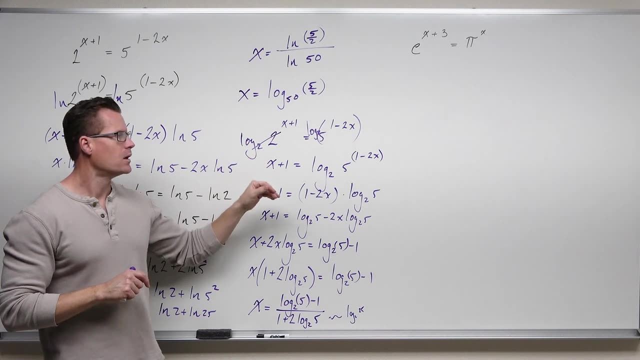 This is one reason why a lot of people use ln- And this one is for sure you're gonna wanna do that. It's kind of the same reason as using ln or log of two here, because you get this cancel thing going on. 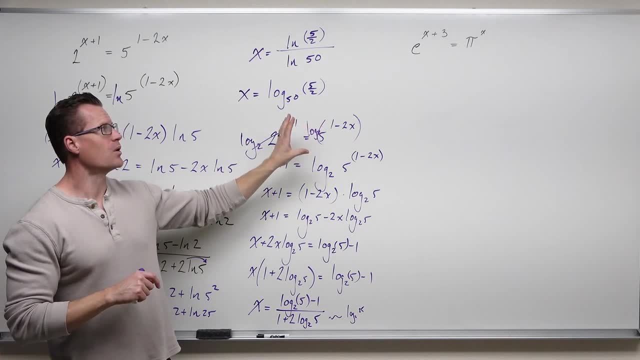 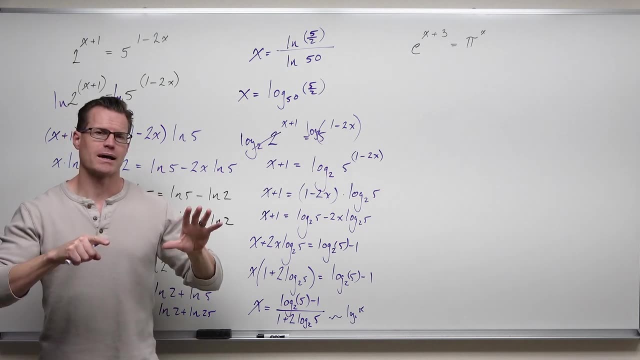 and you deal with something with a different base on the other side, and that's okay. But with a log base e, you don't have to write that base. So it looks a little cleaner and a natural log is something we can automatically evaluate on our calculators. 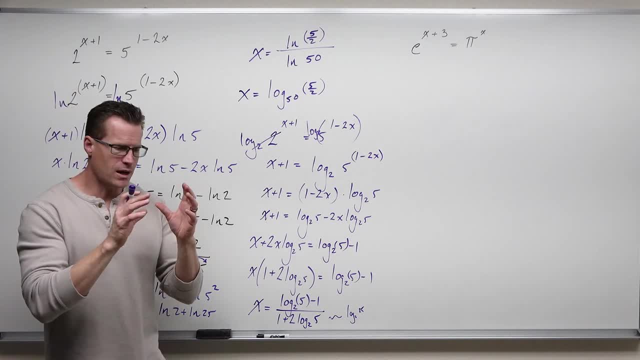 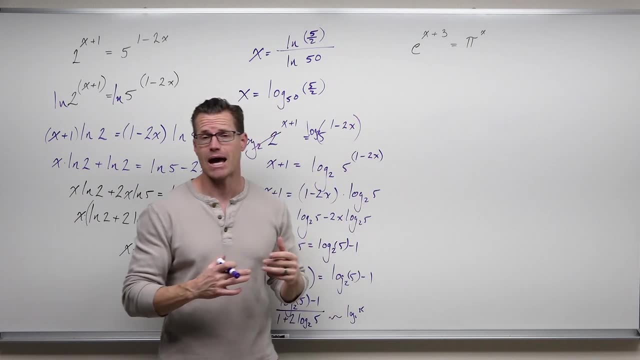 So that's very nice, very convenient. So we qualify this, So we say what it looks like. Is this an exponential where you can have common bases? No, that's not gonna happen. Is this an exponential equation where you have an exponential on one side? 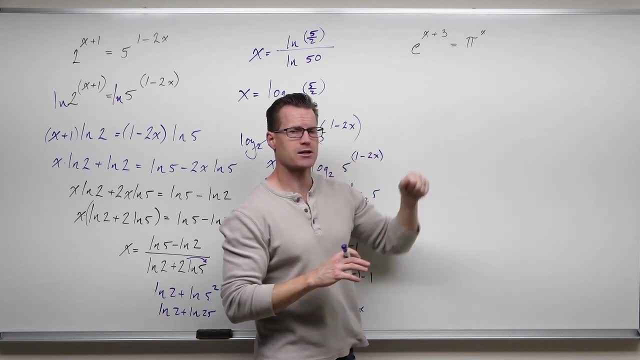 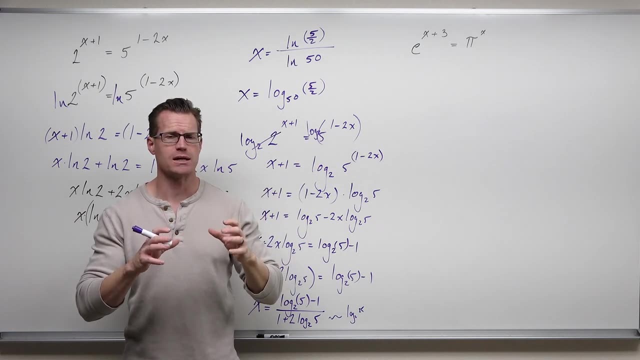 and a constant on the other. No, we have two valid exponentials, both of which have variables in their exponents. So we cannot do those two techniques. We have to. we're forced to do a logarithm on both sides. So you could choose a log base 10,. 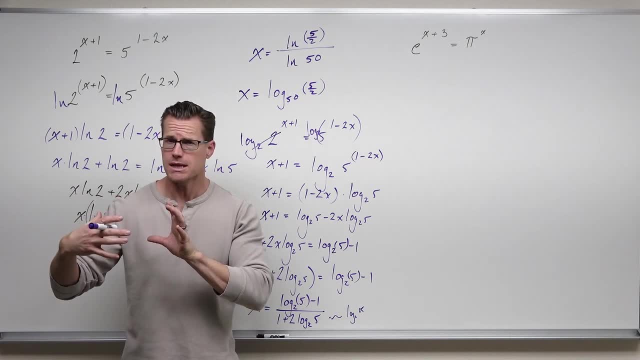 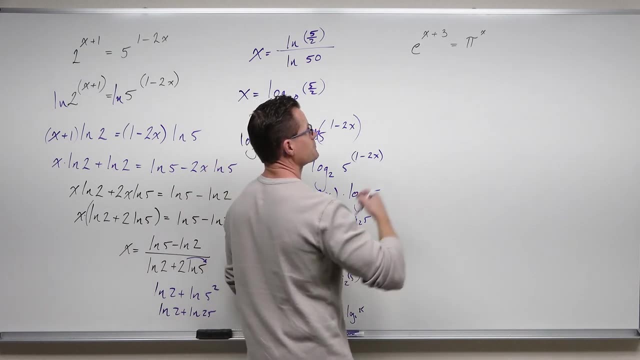 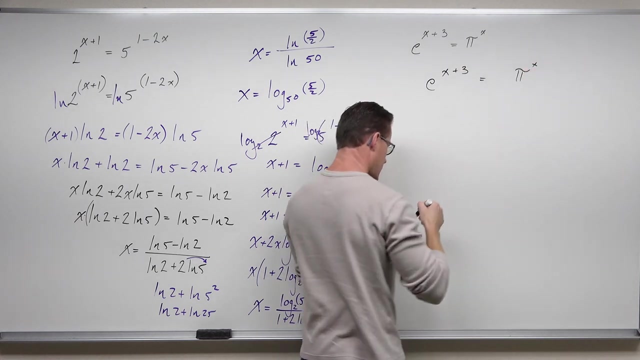 y. or we could choose a log base- e, Yes, y- a natural log That already has a base of e. So when we do a logarithm on both sides and we choose that base of e in our logarithm, it inherently composes a function with its inverse. 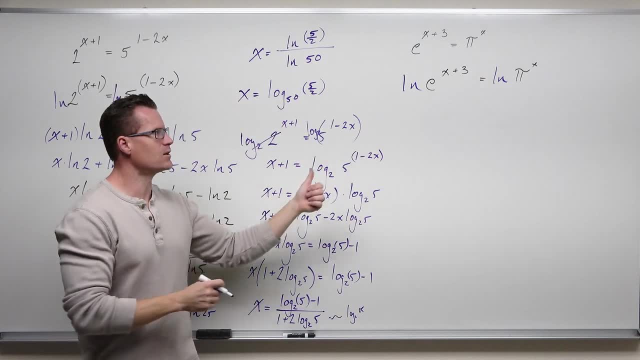 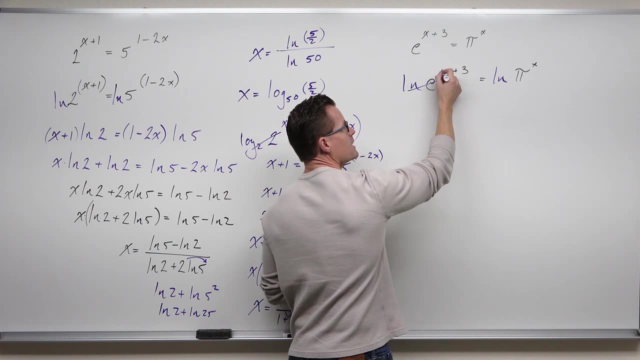 And it doesn't make the other side worse like it kind of did over here. That was a little bit tedious to work through What it does. it says: this is a log base e. This is exponential base e We know from our properties. that's gonna simplify. 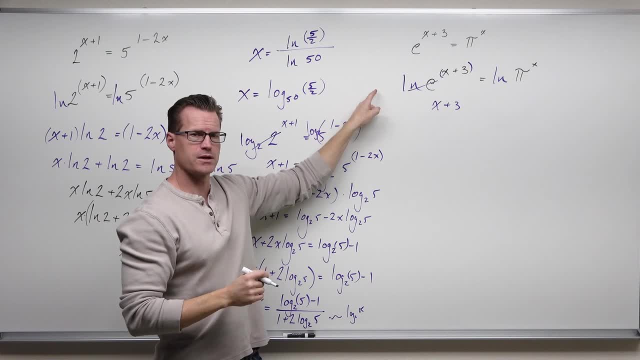 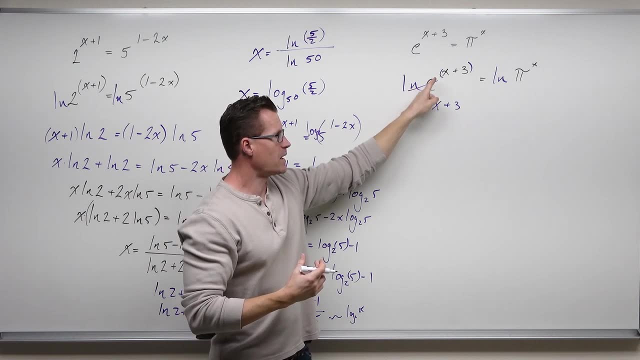 and we just get x plus three. Do you need to move this to the front of your logarithm? You can, but it's not gonna be relevant. You're just gonna get ln of e to the first power. You get a one. 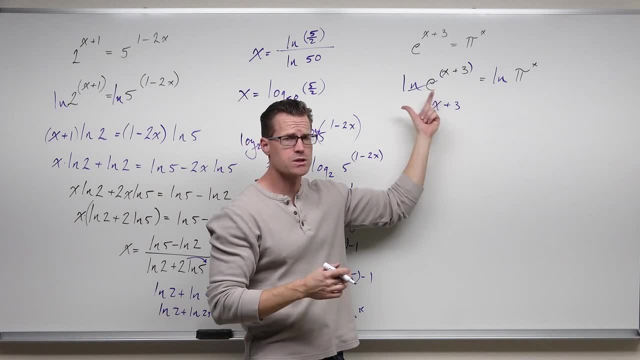 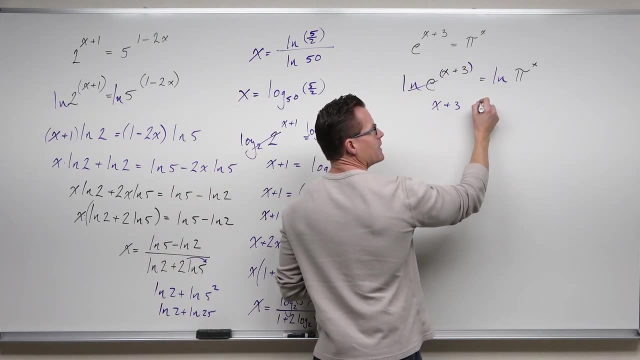 One times x plus three gives you x plus three. This property is fine. You're using a property of exponential. oh sorry, logarithm's right here to say: when you compose a function that's inverse, it does cancel On the right-hand side. nothing really happens. 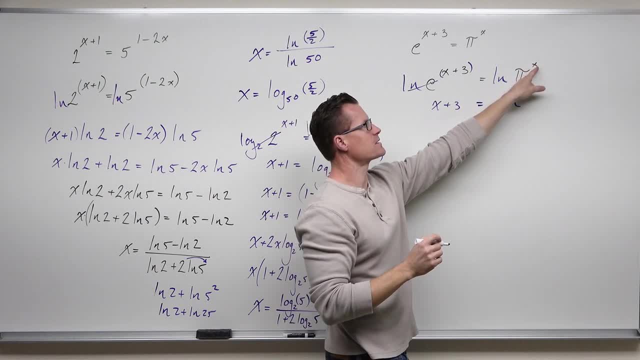 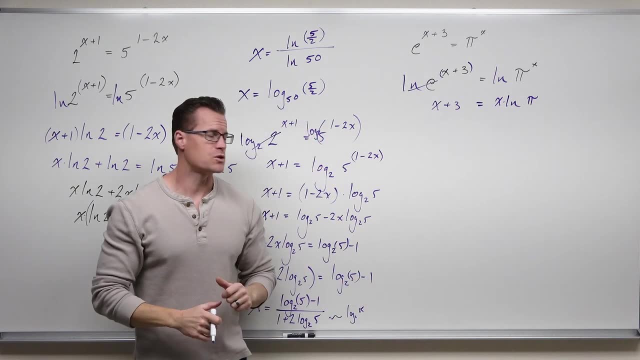 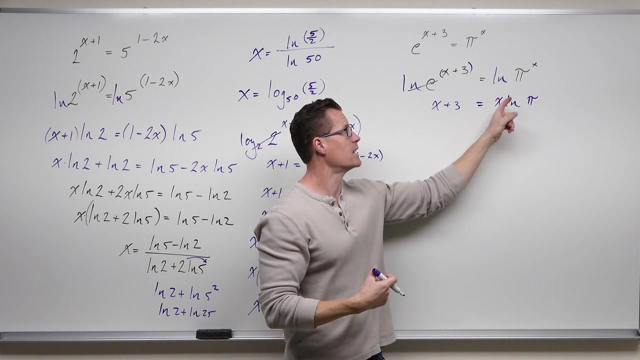 Besides the fact that we have to move this to the front as a coefficient Now there's no distribution to do, like we had to do over here, because we just have that x to the first power, not add or subtract it. If I would've put like a minus two here, 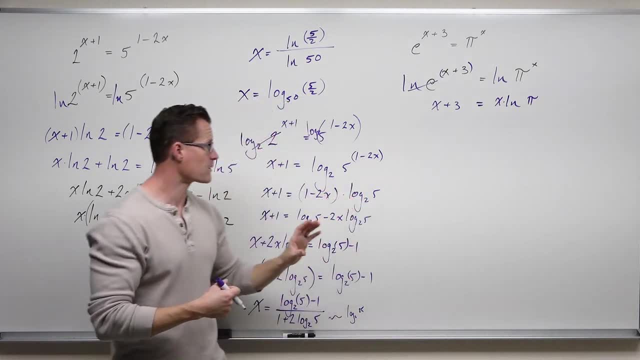 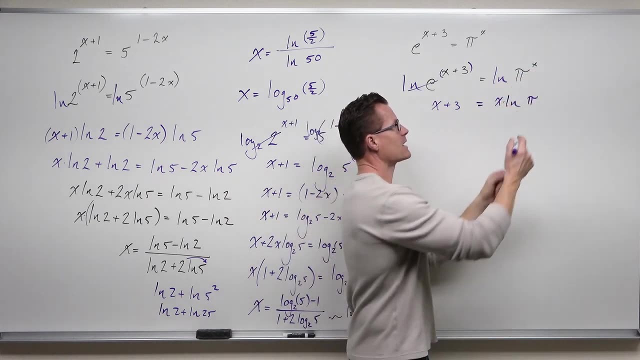 then, yeah, I'd have to distribute and combine my x terms. It would look very much like this example or this example, which is why I'm not showing that to you. I've already done that. So if that had like a minus two, 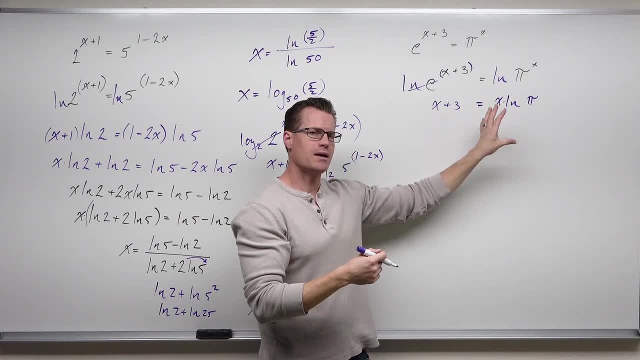 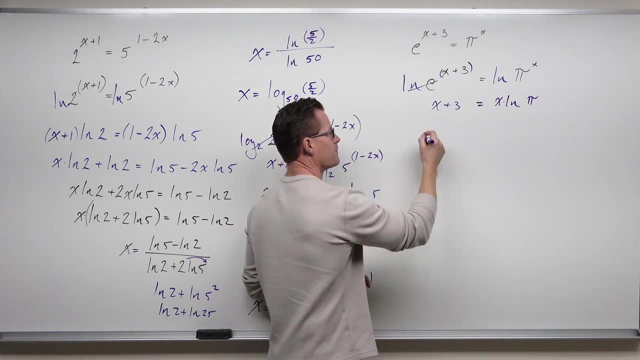 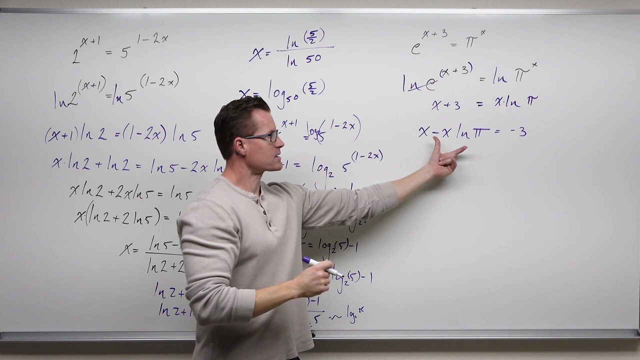 we'd have to have an x minus two and then distribute. In this case we're gonna group our x terms on one side, our non-x terms on the other. This is telling you you're gonna have to factor and divide. So I've subtracted x, ln, pi and subtracted three. 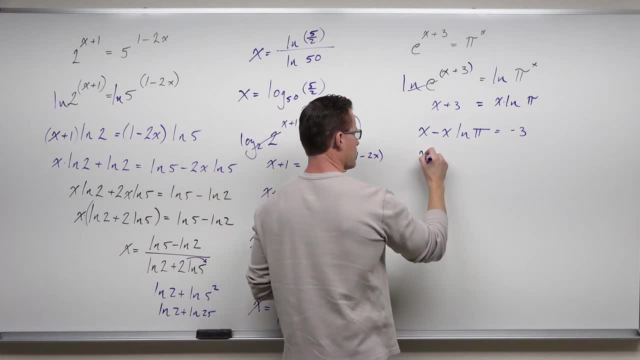 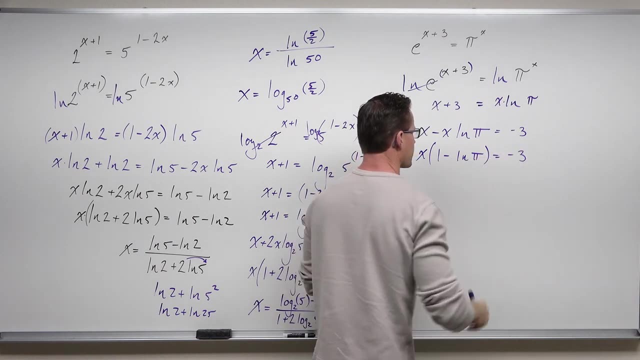 Now that we have all our x terms grouped, we can factor that x And lastly, we're going to divide both sides When we're done. that's about as clean as I can make it. There's no other. there's only one logarithm. 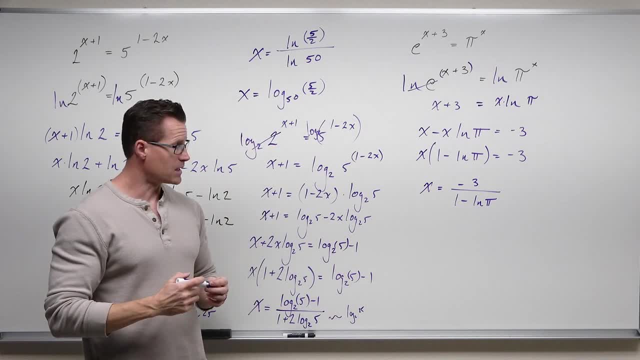 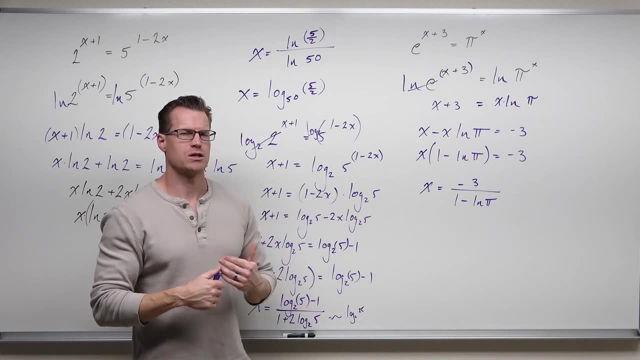 And so there's no logs that I can combine. I hope that you've seen why we like to use ln a lot. It's a little easier to write, It's on your calculator and it cleans up every time we see an e in components. 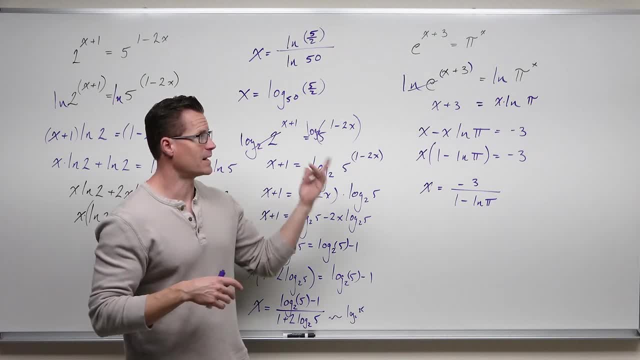 So I hope that you've seen why we like to use ln a lot. It's a little easier to write. It's on your calculator. You can use the e and compose it with a natural log. It's very, very nice. Also, you're noticing one thing. 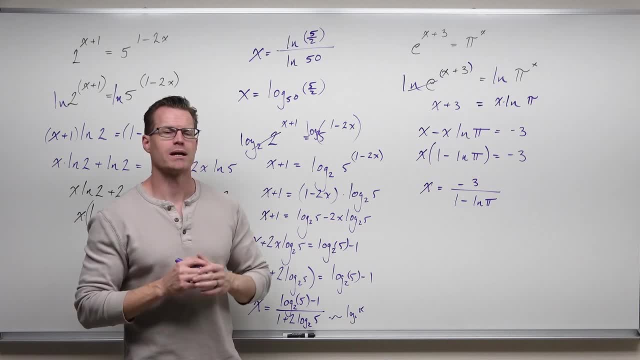 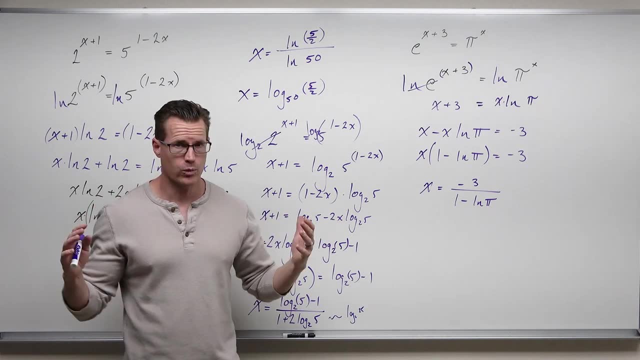 You're noticing me not really plugging in a lot of these to say, hey, what about our domain? Remember something: Our domain for exponentials is all real numbers. So it doesn't matter what we plug in to our exponentials, we're gonna be able to get something out. 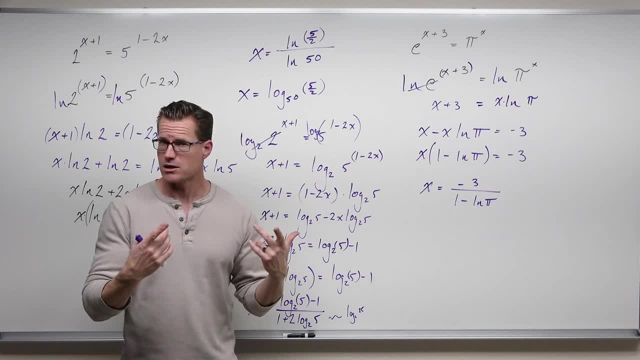 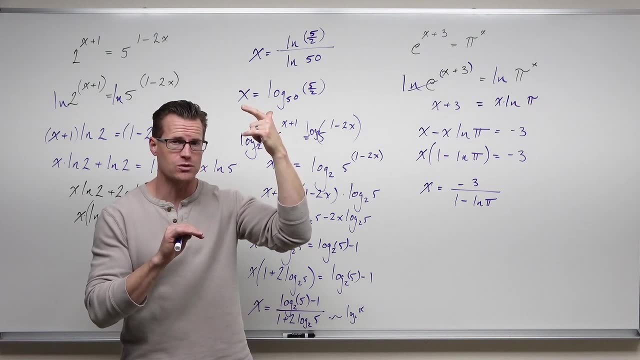 What that means is that we're never having a domain issue. Now, the range of an exponential is from zero to positive infinity, not including the zero. Remember that you can't plug in a number to an exponential and get zero unless it's been shifted. 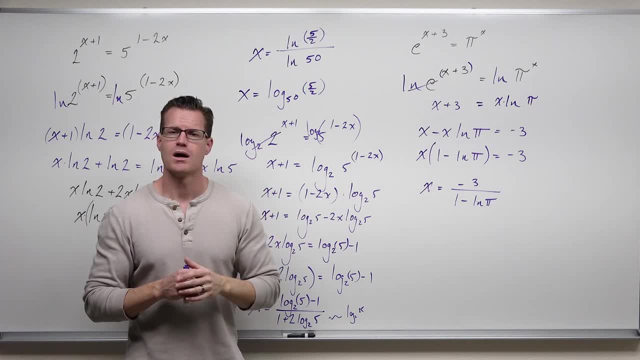 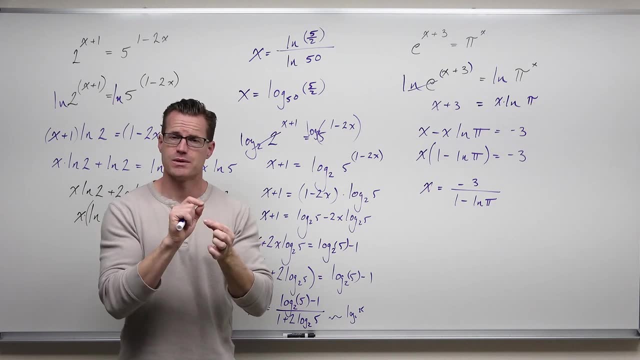 So there will be some horizontal asymptote somewhere on our exponentials. What that also meant for logarithms was that your domain has to be reversed from an exponential and your range is reversed from an exponential. Let me explain it a little bit better. If your domain of an exponential is all real numbers, 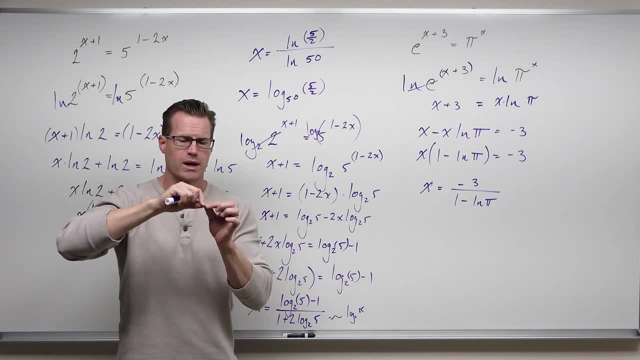 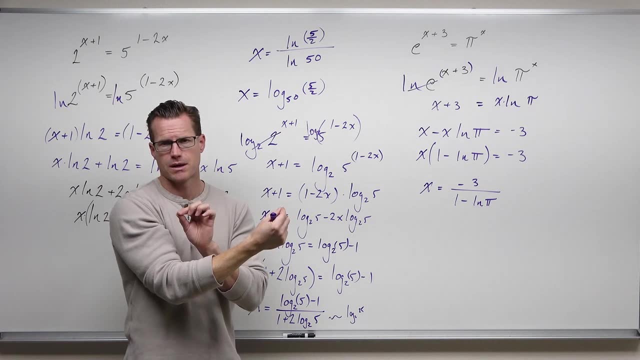 your range for a logarithm is all real numbers. If your range for an exponential is from zero to infinity, your domain for a logarithm is all real numbers. logarithm is from zero to infinity. Is that a problem when we start taking a logarithm on both? 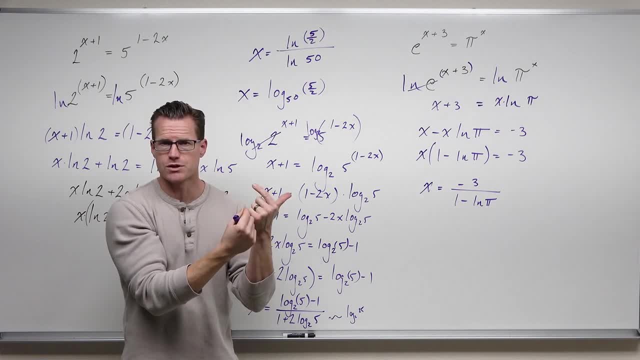 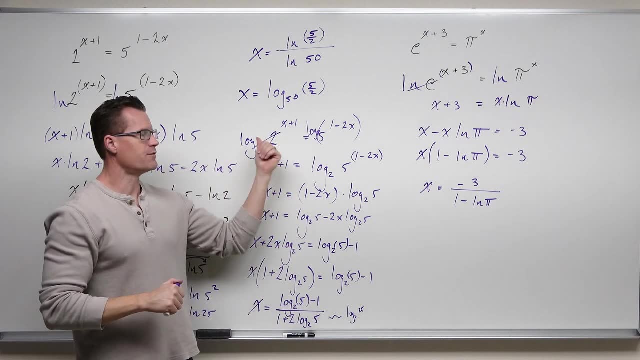 sides, Because we should always be thinking of the domain right. Two functions are inverses on their domains respectively. So think about that. When I take a logarithm of both sides of an exponential, do I have a problem? Am I saying, oh, that could be negative. I'm not, Because an 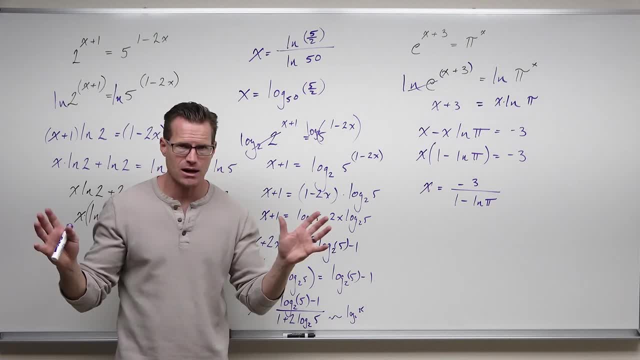 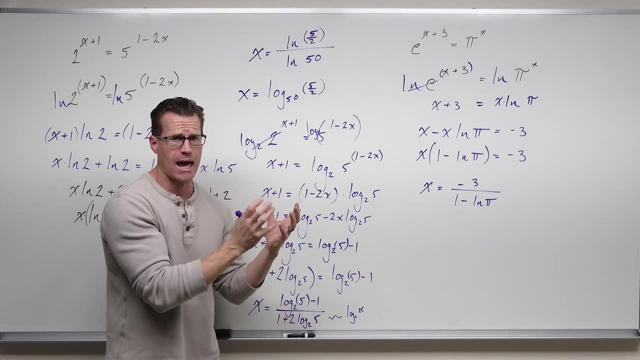 exponential can only give me out positives. It cannot give me out negatives unless it's been shifted around, and that would be a constant added afterwards, added after your exponential. We don't have that. That's always positive, That's always positive. And so when I take a 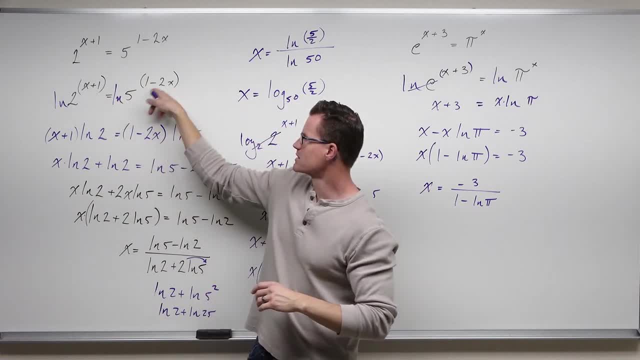 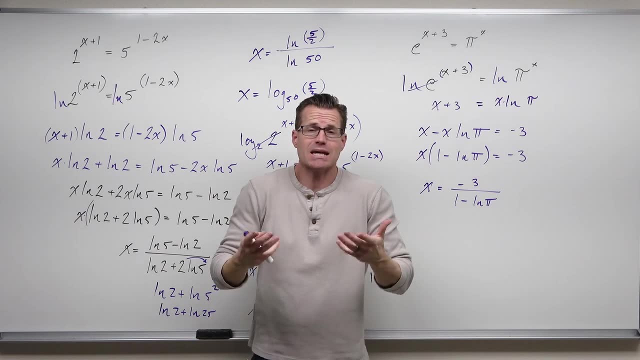 logarithm of both sides, no matter which one I do, this is always positive. this is always positive. That logarithm is saying I need my insides to be positive. The exponential says: no problem, I can't even give you a negative, I can't even give you zero, So we're not breaking a domain issue. 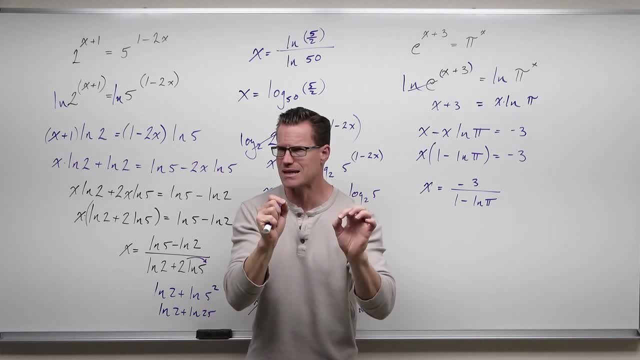 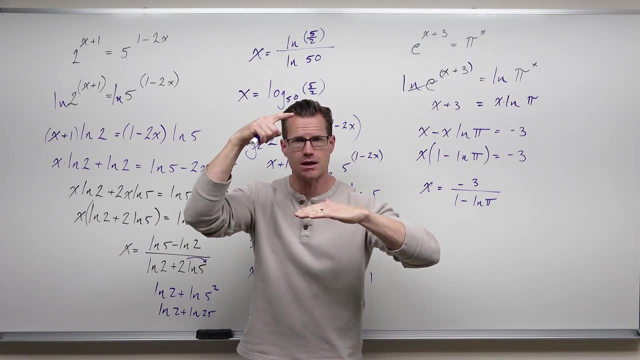 when we take a logarithm on both sides of our exponentials. I hope that you're seeing that, seeing that, yeah, I'm doing a logarithm and the insides have to be positive, but exponential's range is from zero to infinity. That matches perfectly with the domain of a. 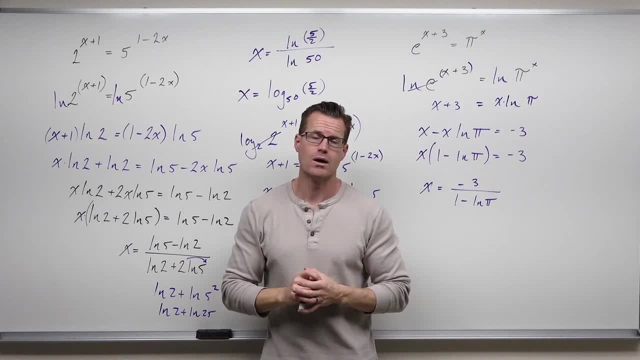 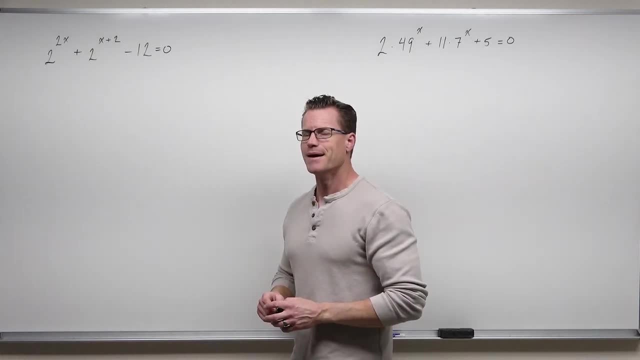 logarithm in zero to infinity, that we need to use a logarithm anyhow. That's why this technique works. They are inverses on their respective domains. Okay, I hope you're ready. We got a couple ones that look a little weird. When you see this, you see several terms, mainly like three. 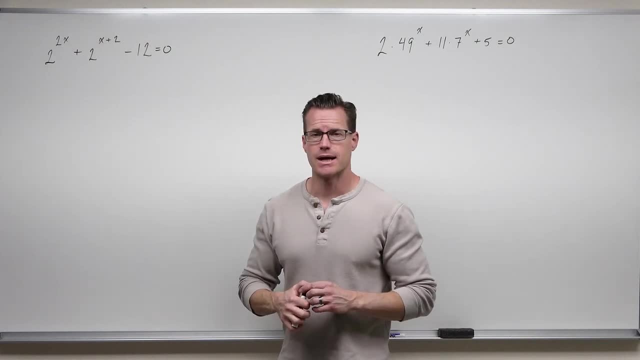 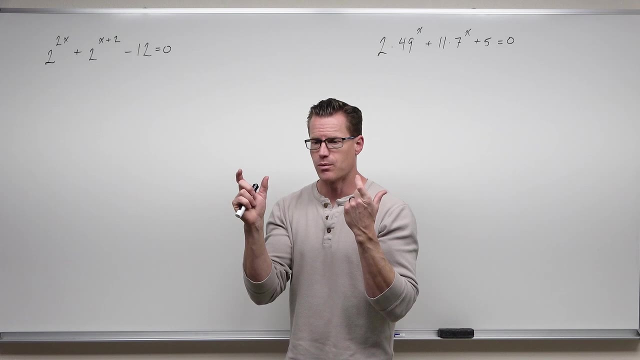 terms and you have some things that say: I cannot possibly isolate an exponential here. I can't get two exponentials on each side, and so I will not be able to use the common basis that your exponential is equal. I won't be able to use a direct. take a log of both sides. I don't just 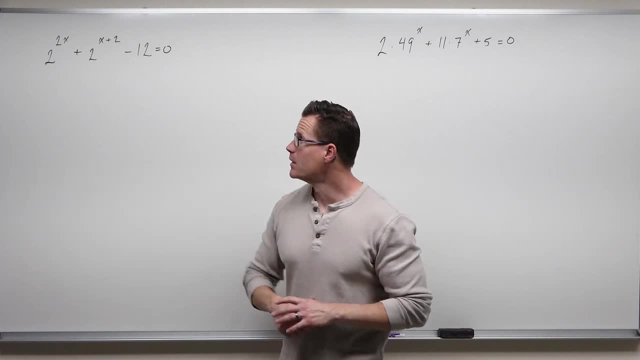 have one of these, one exponential, and I can't combine them, and so I won't be able to go straight to a logarithm. Typically, what you'll do here is a substitution technique, and so here's the thought process: If I've got not all exponentials, I can't isolate one and I can't make them equal. 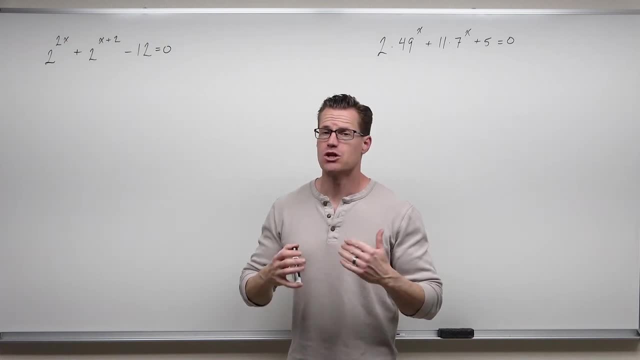 so I can't use logarithms as a common basis. I'm going to have to change it to something that's not an exponential to solve it and then put the exponential back. So when we take a look at it we go all right. can I write this as something where 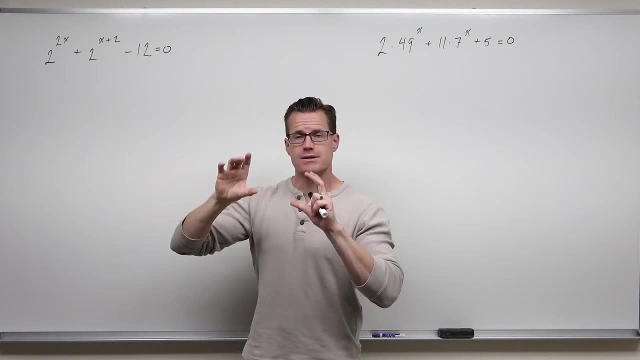 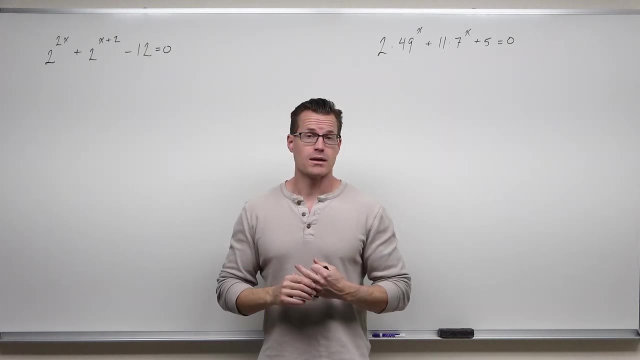 the first term and the second term have the same exponential? Right now they don't. Right now we have two to the two x and two to the x plus two. Those are very different. They have the same base, though. That's very important. And then a constant. Well, you don't necessarily need a. 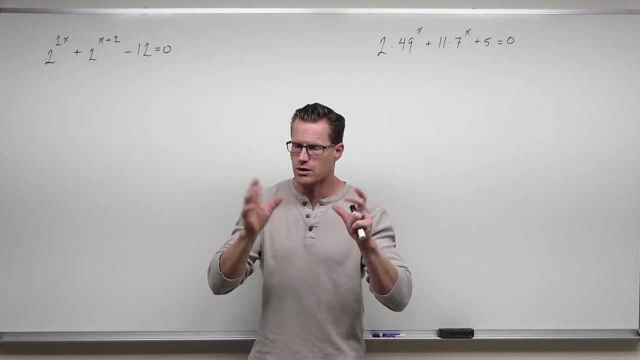 constant, but can I write at least the first two terms, or all the terms, if you want, if there are, as having the same exponential that we can substitute. So we're going to do things like use some exponent rules to rewrite these a little bit and I'm going to walk you through that. 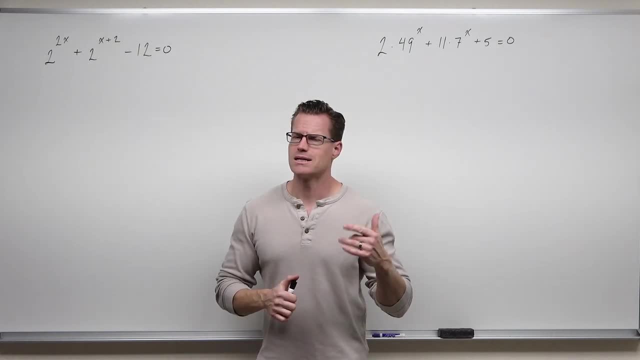 So something like two to the two x and two to the x plus two. Firstly, identify what your exponential wants to be. We're probably going to work this down to two to the x. Well, that means I need to rewrite the first term as two to the x and the second term as two to the x times something. 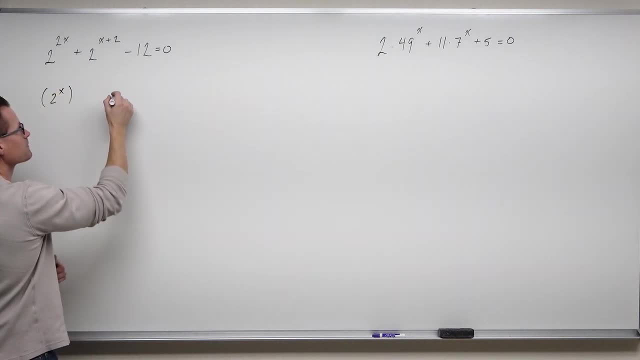 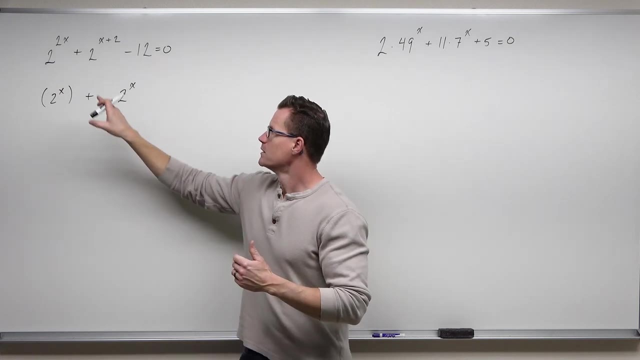 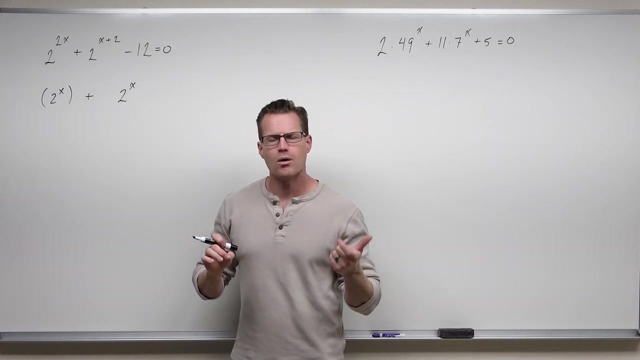 the first term as two to the x and the second term as two to the x. Think about what two to the two x means. Two x is two times x. Now, how do we get two times x for exponentials? Well, that had. 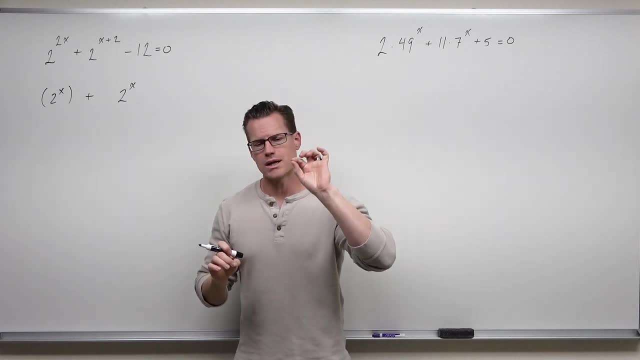 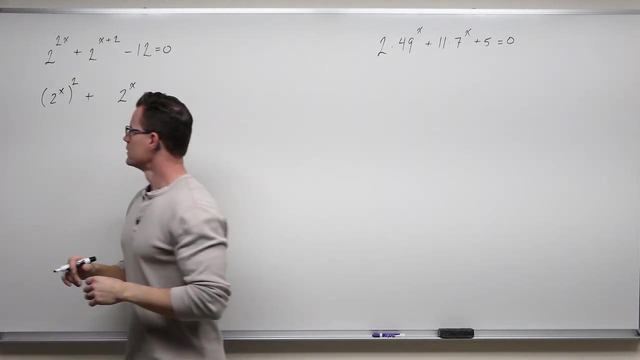 to come from an exponent raised to another exponent, because when an exponent is raised to another one we multiply those. So this came from two to the x squared. Notice how this still makes two to the two x. So we're just thinking through kind of the. 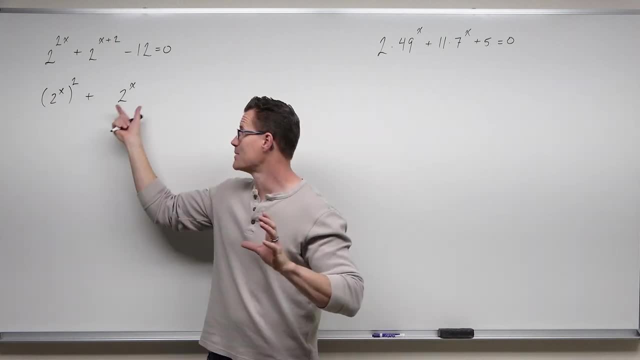 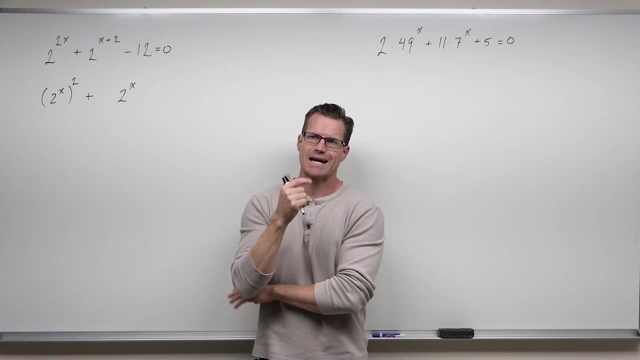 opposite of some exponent rules, and writing this as something that's going to be the same, as another part of my function, another part of that term. Now, how about two to the x plus two? Well, I need two to the x, but x plus two. How do I add exponents, Exponents that are added. 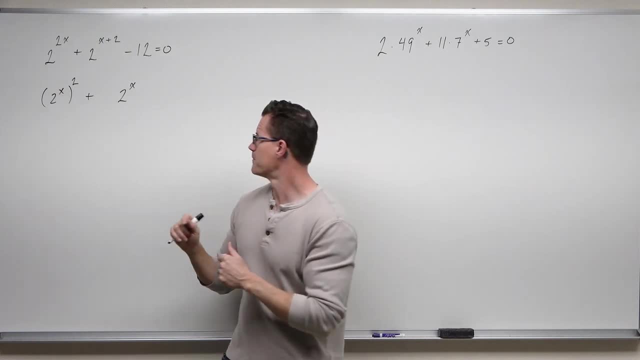 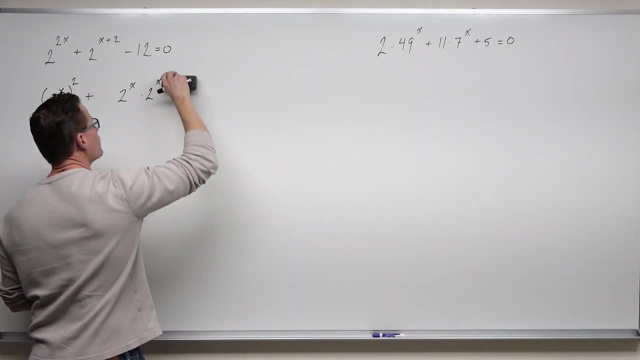 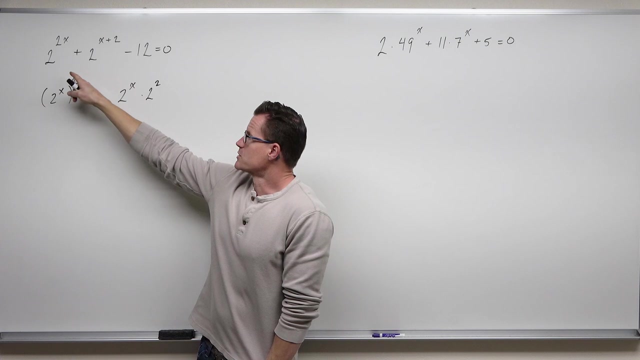 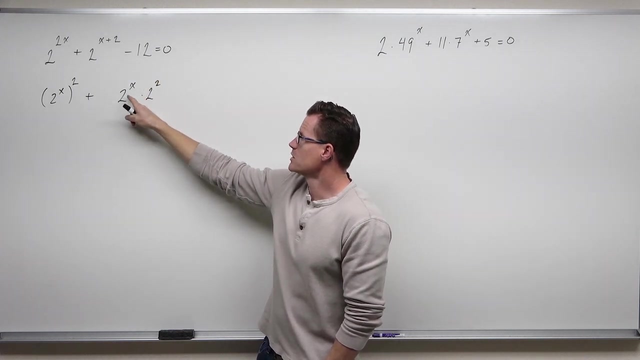 came from common bases that were multiplied. That's not right. That is what I want. second, So two to the two. x came from x times two. x times two is two x, Two to the x plus two came from two to the x times two to the second. Notice how, if I were. 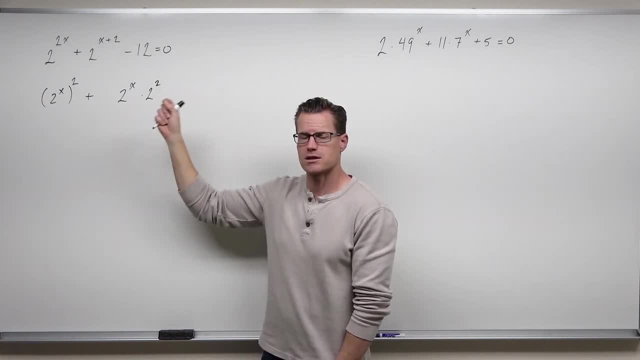 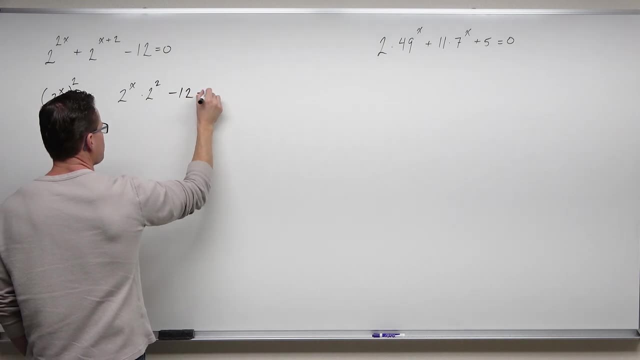 to combine those, I would get common base. I would get two to the x plus two. I would add those exponents- That's where that came from- And then minus 12.. So we've pretty much accomplished what we set out to do. If we simplify that just a. 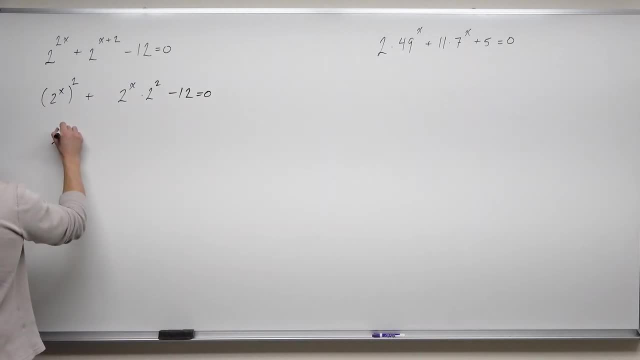 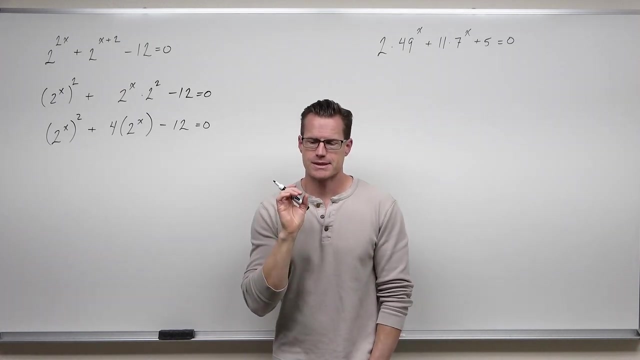 little bit, that's just four. So when you're trying to do a substitution, we're trying to make the first term and the second term have the same exact inside, In this case the same exact exponential two to the x- And then we're trying to make the first term and the second term have the same exact inside, And then 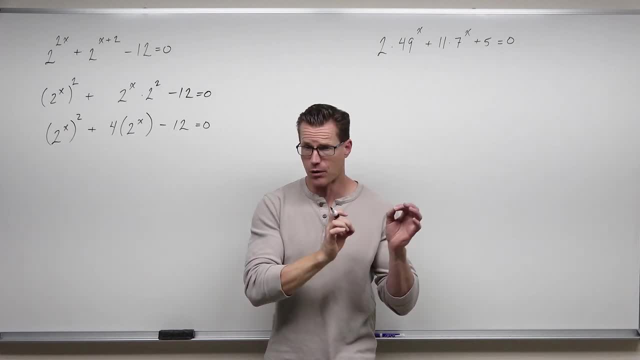 we have these powers. whatever we have, it doesn't really matter. We're trying to get that out of there. So when we accomplish that, when we look at it and say, hey, I can rewrite these and I can rewrite them so that I have the same exponential in two spots and nowhere else, Well then I'm. 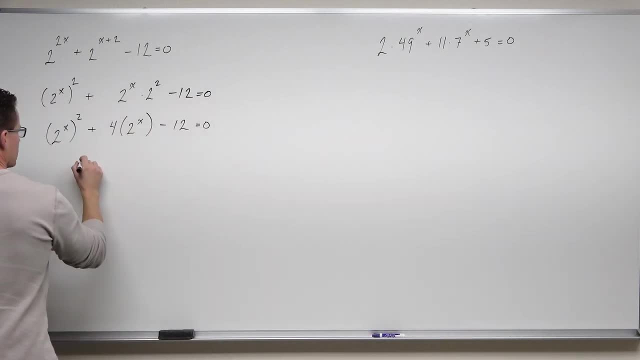 going to do a substitution. I'm going to call that u Now we're going to use that twice. We've seen this several times. We know that we're going to get away from 2 to the x and then later on we'll. 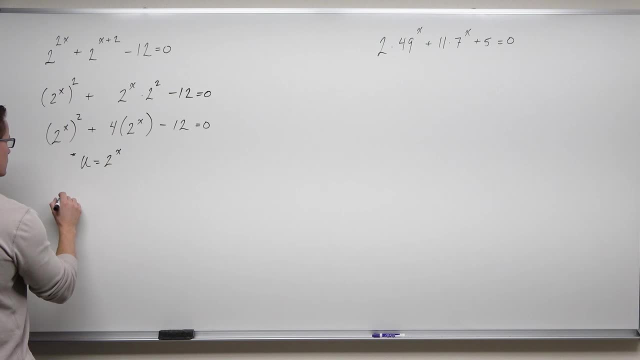 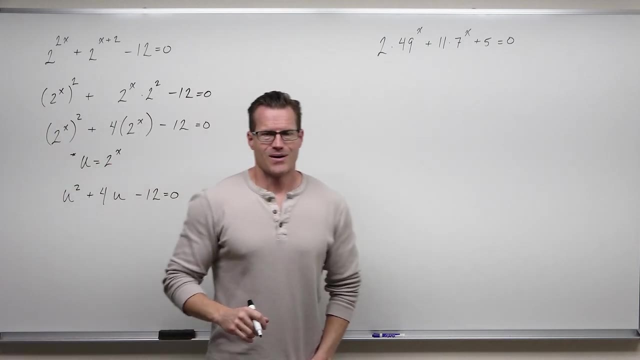 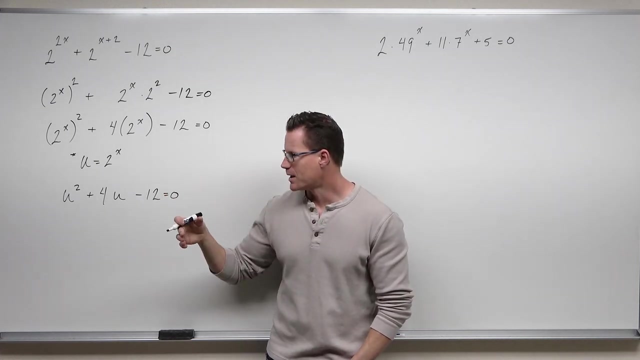 go back to it. Almost always, what you get is going to be factorable. So you get everything on one side. get it in order- it's first term positive- and factor it. If it's not factorable, I'm not going to do one for you. This is how I'm really not. If it's not factorable, you need quadratic. 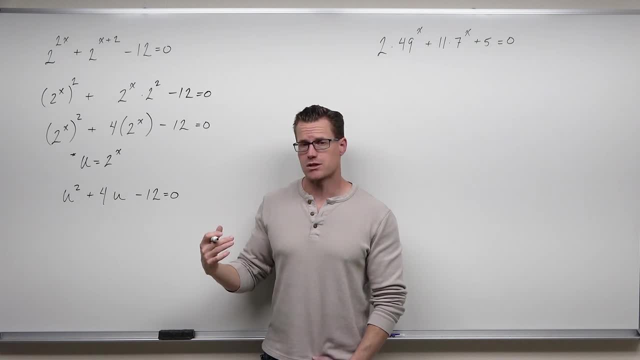 formula. If it's higher than a power 2, you need another technique to solve it. But ultimately, once you solve it, you go back to the hey. the u you solved for is 2 to the x. Put that back and then continue with the logarithm, And you can do that. I gave you four techniques. 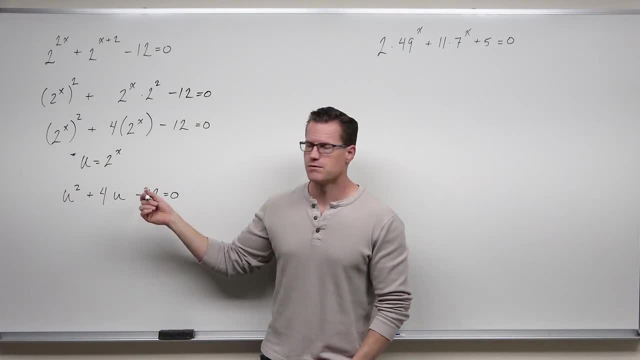 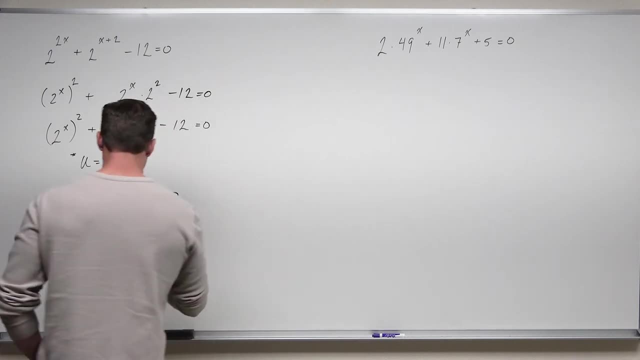 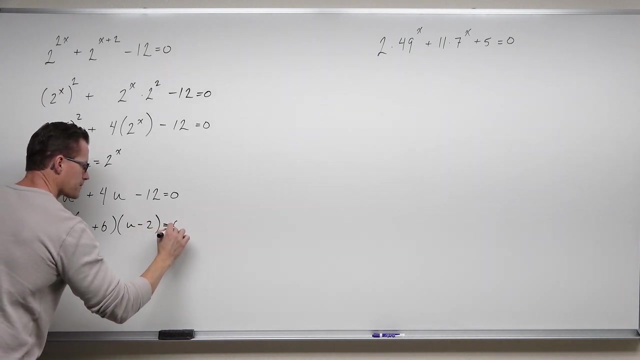 on how to do that, But most of these are factorable. If not quadratic formula, it's kind of nasty, But they are factorable most times. So this would be: u plus 6, u minus 2 equals 0.. 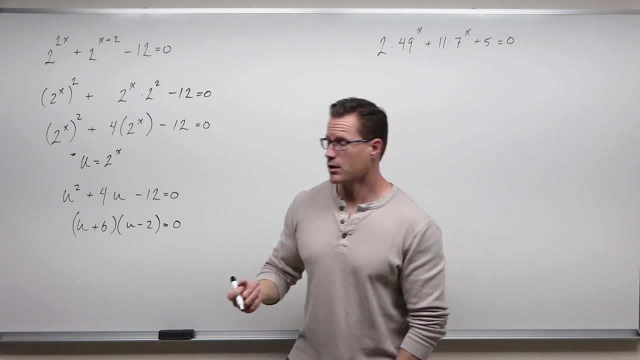 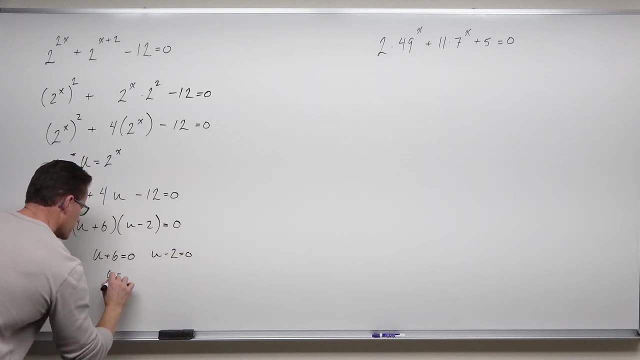 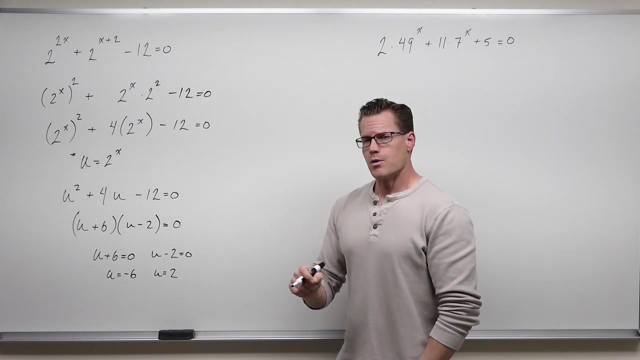 You can check it, but that's going to be correct. Zero product property says: keep on going. Now you're not done. You're so close but you're not done. Remember that we're not trying to solve for u, We're trying to solve for x, and our x is wrapped up in the exponential We said. u is 2 to. 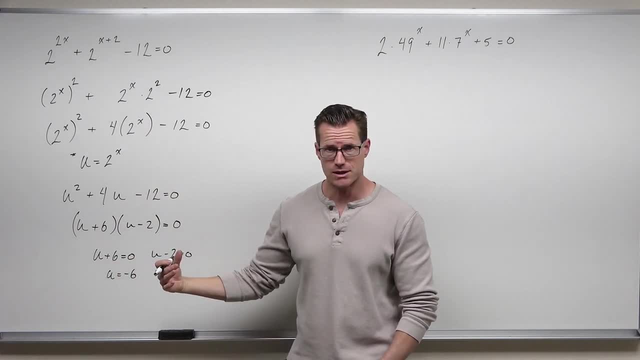 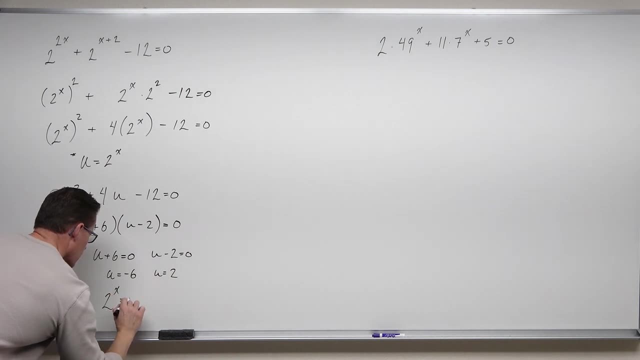 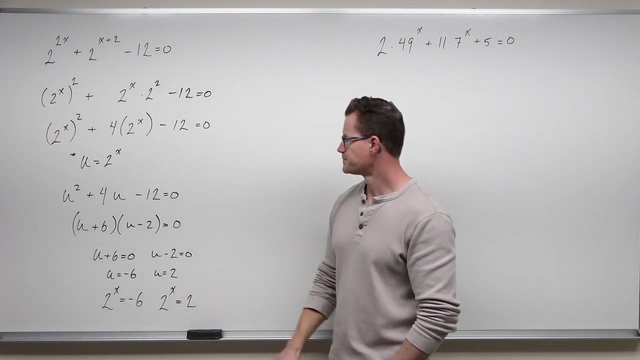 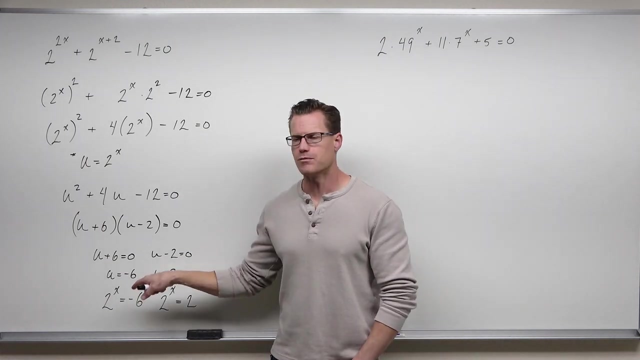 the x. So if u equals negative 6, then 2 to the x equals negative 6.. And if u equals 2, then 2 to the x equals 2.. Now, what do we do? Well, we think. Firstly, let's think about this one: 2 to the x equals. 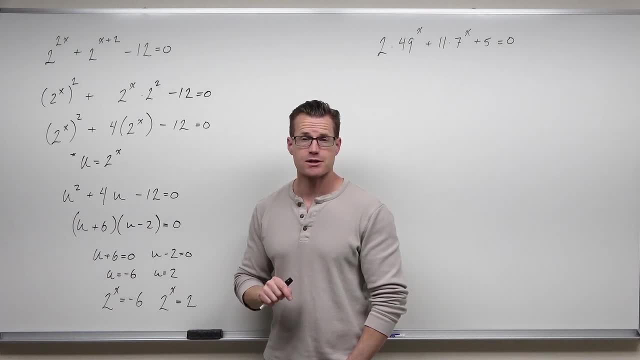 negative 6. And you go. wait a minute, I thought exponentials had to be positive. That's true, And sometimes in these techniques they can be positive. And sometimes in these techniques they can be. we get a false solution. This is not valid. Your exponential can't equal. 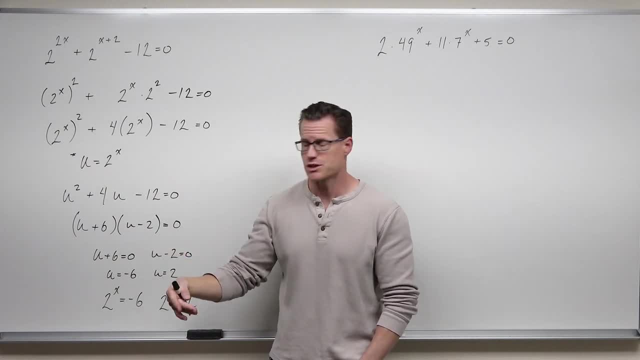 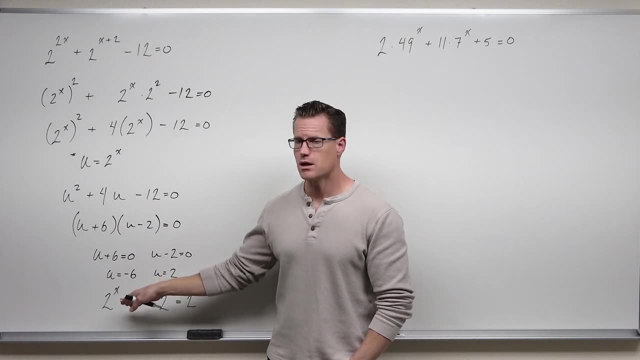 negative. Do you remember? they have a horizontal asymptote at zero. They can't even get below zero unless you start shifting them, and that's not shifted. So this right here is not okay. This right here is not a valid solution. There's no X you can plug in to. 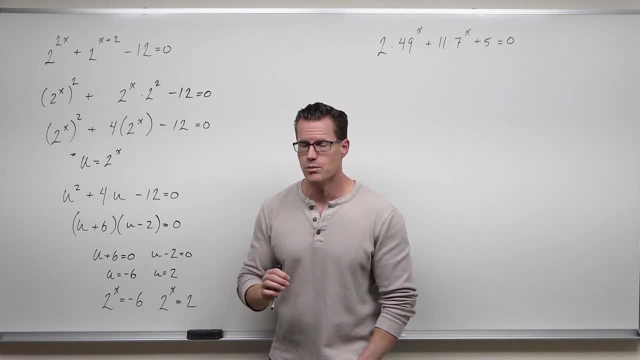 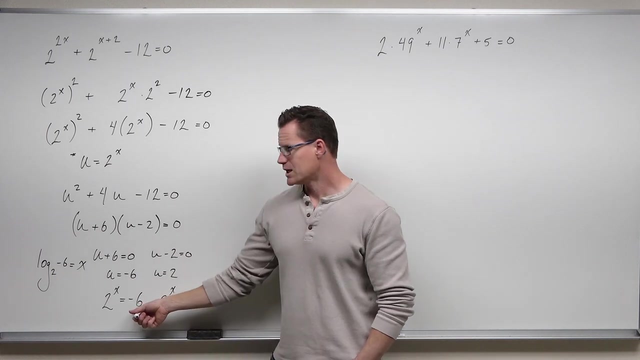 make this actually happen. Now, if you tried to, if you went to a logarithm and said: hey, my base is 2, my exponent is X, you end up with a domain issue, A range issue. listen, a range issue for an exponential. what you get out is a range. 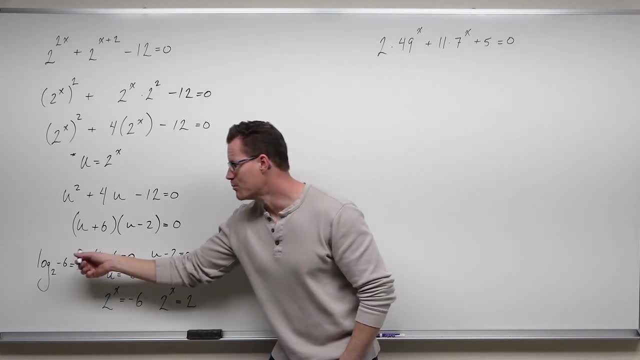 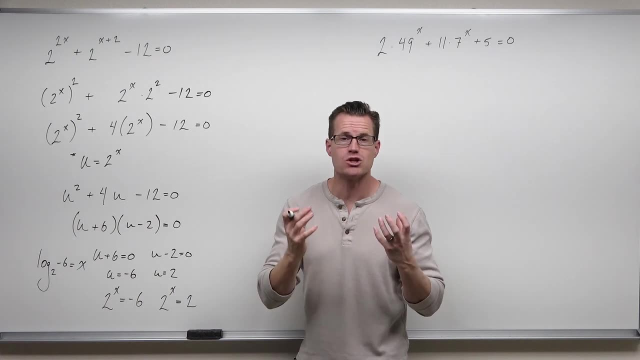 issue. A range problem for an exponential becomes a domain problem for your logarithm. Why? Because range and domain switch for every inverse relationship that you have As far as functions go. functions are concerned, including exponential logarithms. This is not a 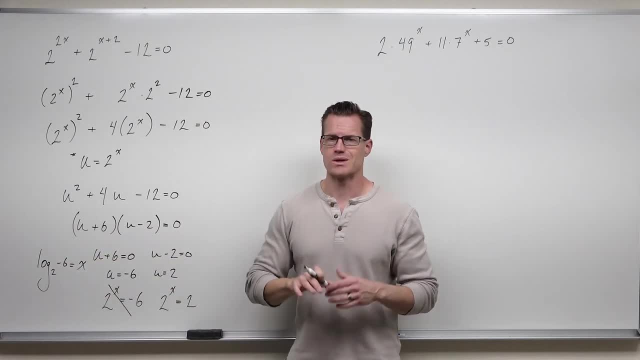 valid solution. It creates a domain issue for the logarithm, a range issue for the exponential. Either way, you just can't have it. Now, what about this one? You can write this as a logarithm or you can just think about it. These have common. 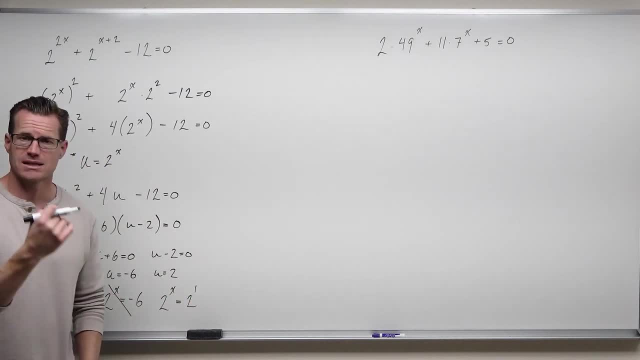 bases. Hey, that's kind of nice: 2 and 2 equal, which means X has to equal the exponent of 1.. Now, in general, this is not what you're going to have to do, right? You're going to have to write this as a logarithm. So you certainly can, because 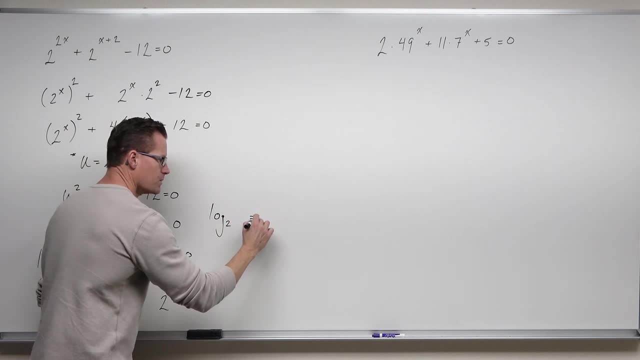 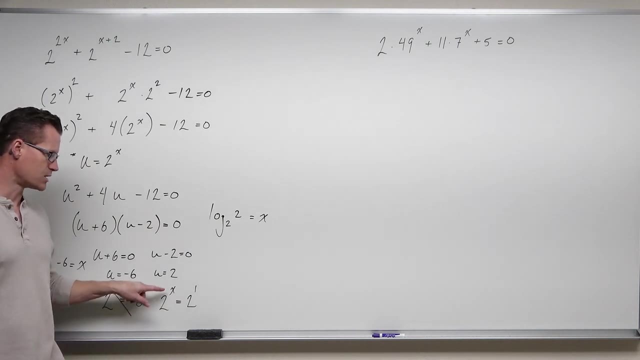 your base is 2, log base 2 solves for that. So log base 2 of 2 equals X. Here's your base, Here's your exponent. We separate those with logarithm and let's use a very nice property. Say: you compose a function with this inverse. That's exactly what we. 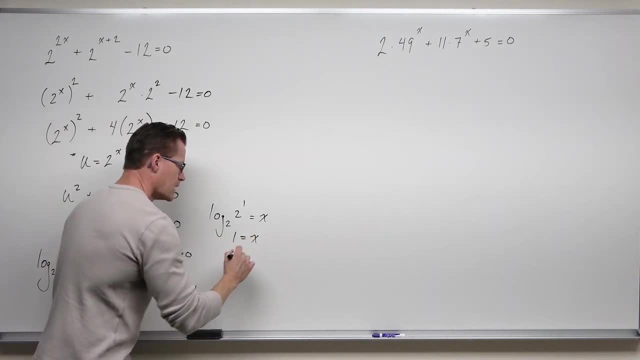 said, You're with the same base anyway and you would get X equals 1.. I'm going to walk you through a couple others. What would happen if this wasn't a 2?? What if this was a 1?? If that was a 1, you can think about it. Just think 2. 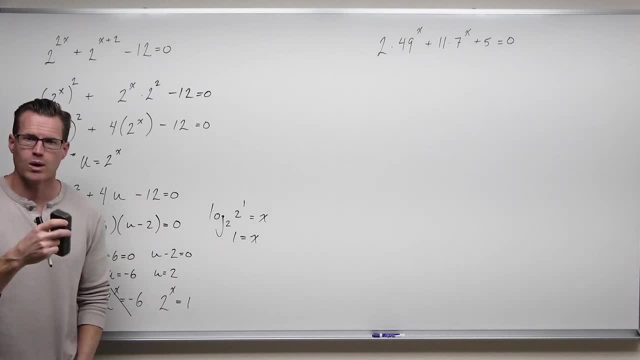 to what power gives you 1? any base to what power gives you 1?? Well, you'd have to have 0. That would bear out right here. So if I had base of 2, exponent of x, a logarithm separates the base from the exponent. 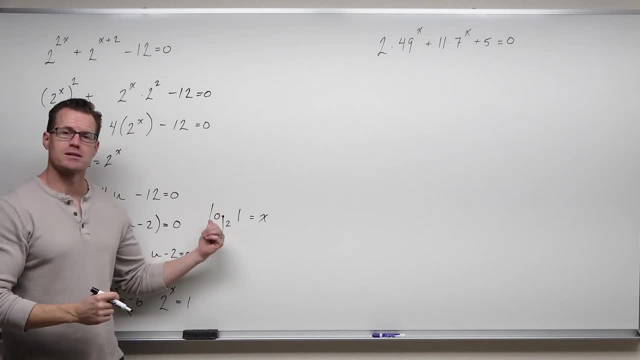 puts what the exponent equals to as your argument and says: hey, that's another property. we have Log base I don't care of. 1 is always 0. Then 0 would equal x. Okay, what if it wasn't one of those special cases? 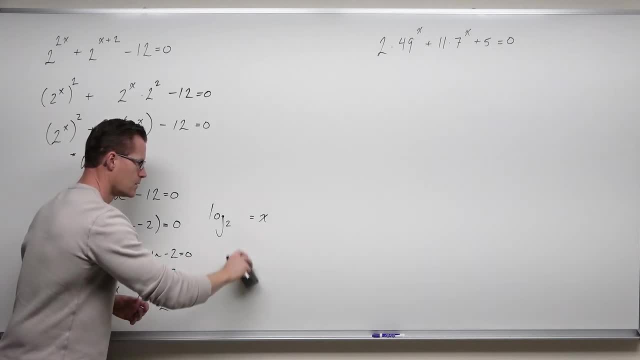 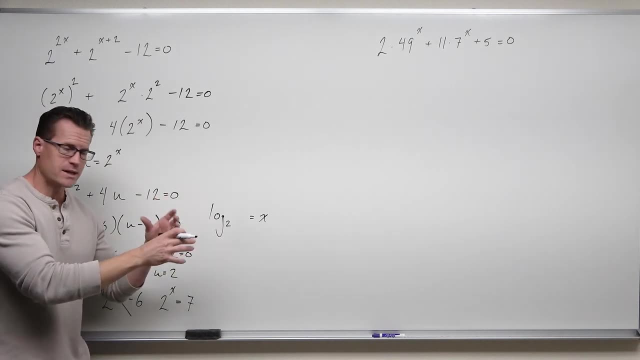 that you showed me, Leonard. What if it was like 7? 7.. What if log base- sorry, 2 to the x equals 7?? Well, logarithm still writes it as log base 2 equals x And you'd have 7 right there. 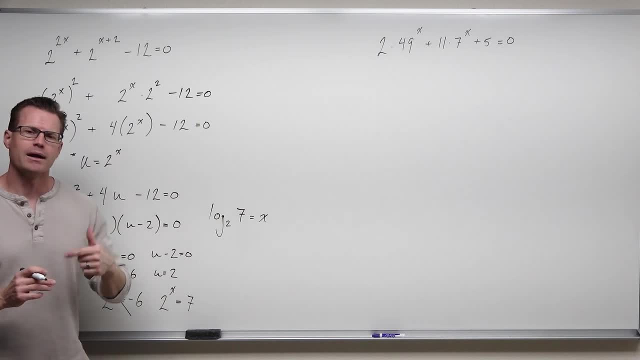 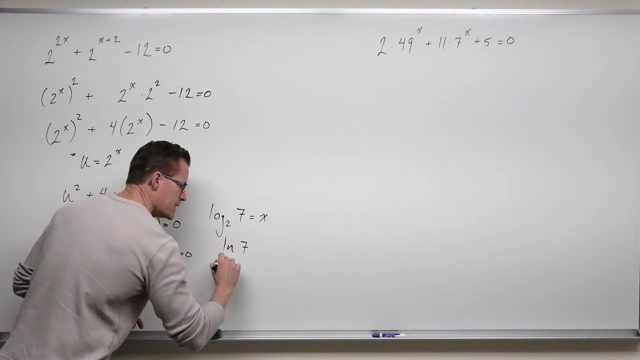 This is a solution. This is fine, You're done. You don't have to do anything more. Now, if you're asked to approximate, which you almost always are, then you could do a change of base Pick ln. Pick log, base 10.. 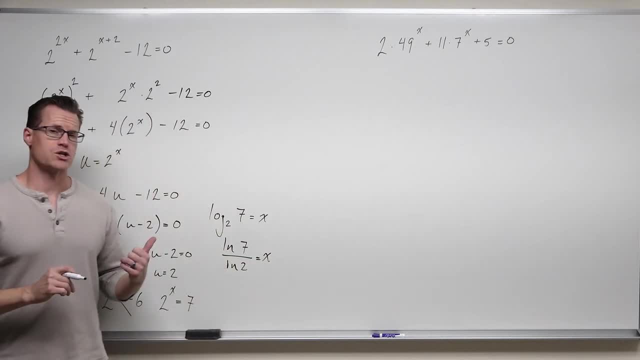 Does it really matter? And you could do a change of base And you can evaluate that ratio. So those are the three cases that we typically get when we're doing a substitution. We never get this whole exponential equals exponential without the common base. 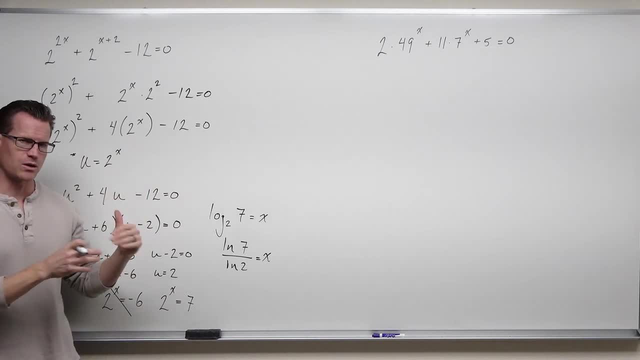 But we never get variables on both sides, So those previous examples aren't really relevant for a substitution, because we don't really get that. What we end up getting is something that looks like this, or the two previous ones that I gave you, And then we can go directly to a logarithm. 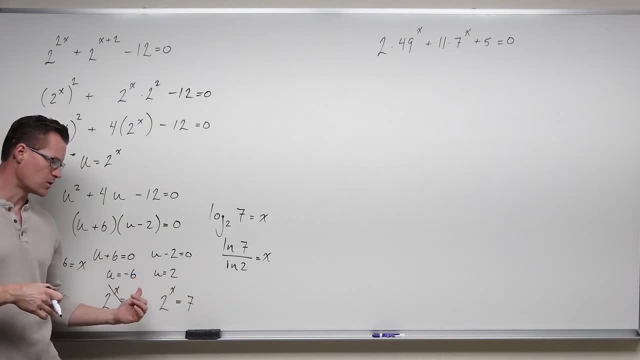 Now, could you? Could you do ln on both sides, move your exponent and evaluate? You could. but it is easiest to go directly to a logarithm And that's why I showed you that first technique in the first example that we did. 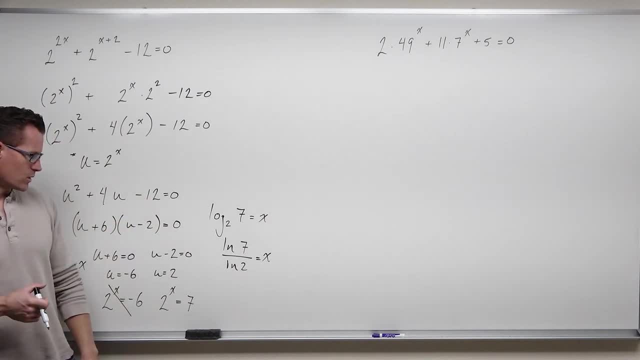 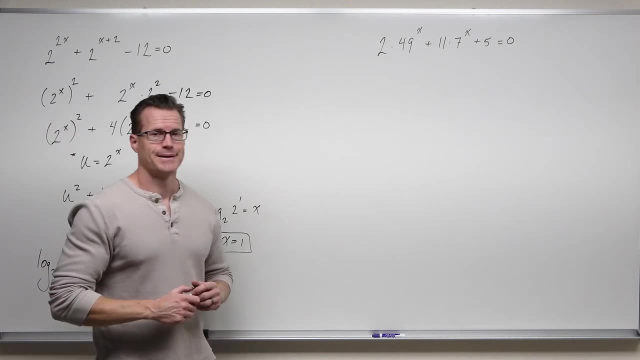 So this would become easier. So I hope that makes sense. Our real answer was one. I just wanted to show that to you just so that we're kind of complete here. All right, Last one. I'll discuss one more with you, but I'm not going to solve it all the way. 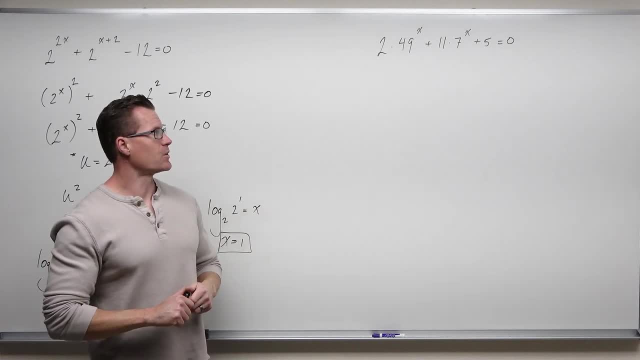 I'll discuss it, This last one that we're actually going all the way through. we're going to look at this and we're going to firstly recognize what it's talking about. This is an exponential equation, Yes, but categorize it. 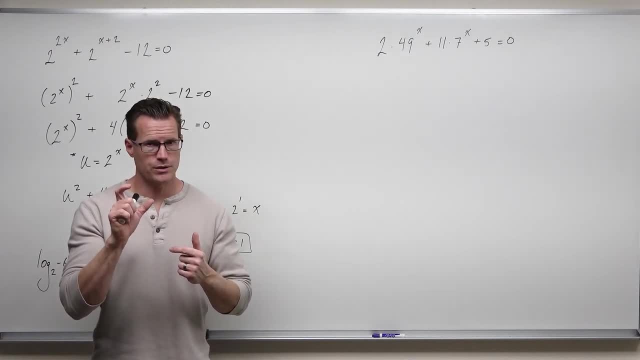 Is this something where I have one exponential? Well, no, That means that I can't isolate it and get a constant on the other side and then use a direct logarithm. Is this something where I have two exponentials, where I can get one on one side and one on the other side? 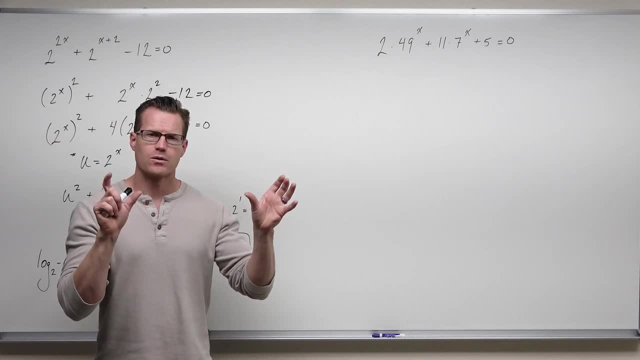 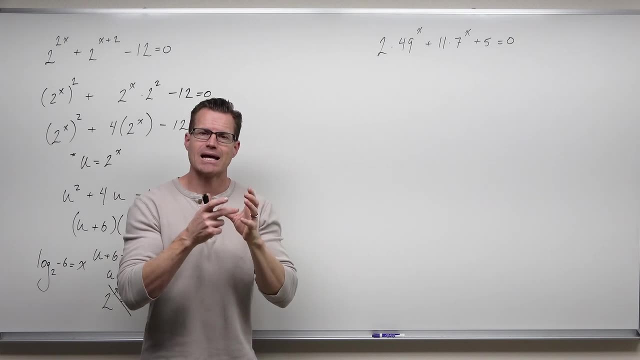 either for common basis or for logarithms. direct use of logarithms: No, because that five messes it up. Actually, that two kind of messes it up too. I can't just get one exponential on one side, One of the other and do a log of both sides is not going to work. 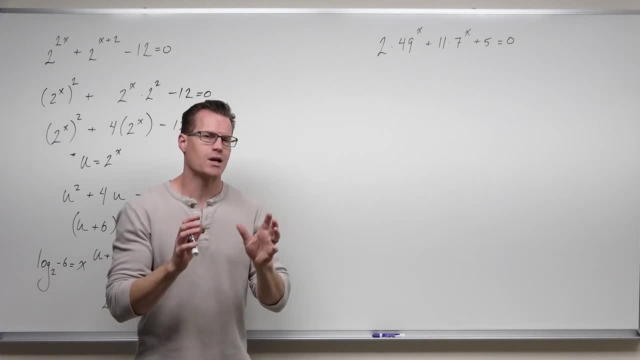 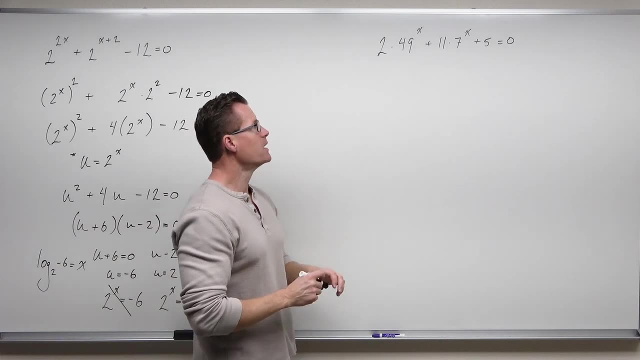 I'm going to have to do a substitution. So if I'm going to do a substitution, I'm going to make this so that I have the same exponential in two terms of my expression here, my equation. So I'm looking at this thing and well, what's the best choice for our base? 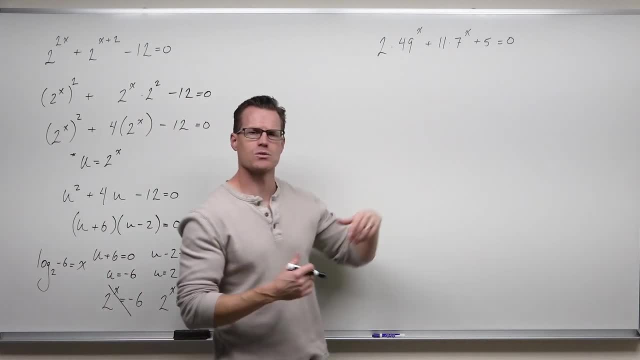 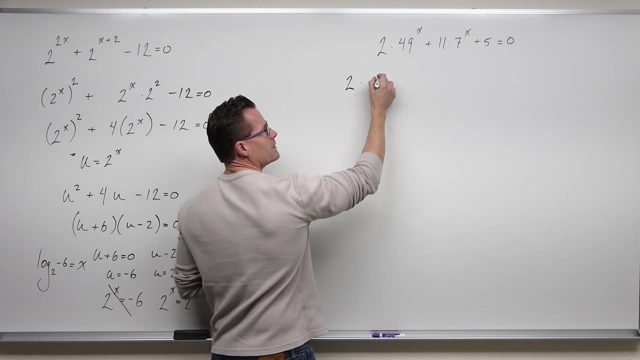 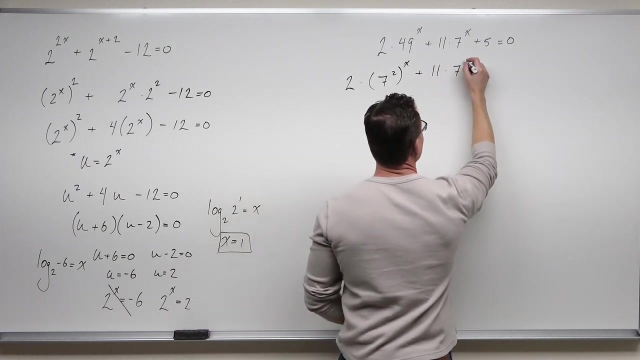 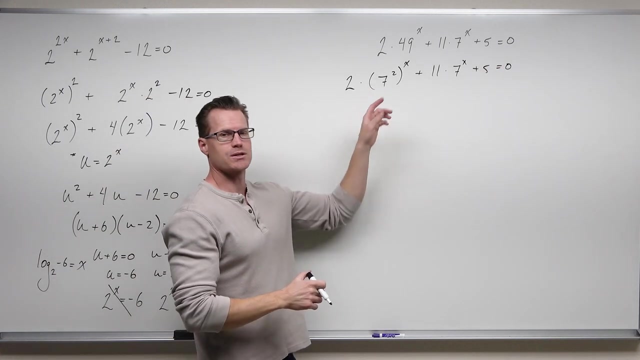 Forty nine looks like you simplify into a base of seven. So we're going to do that first. So I'm thinking I want to write this as a base of seven. This is seven squared. Now. that's all well and good, but that doesn't help us. 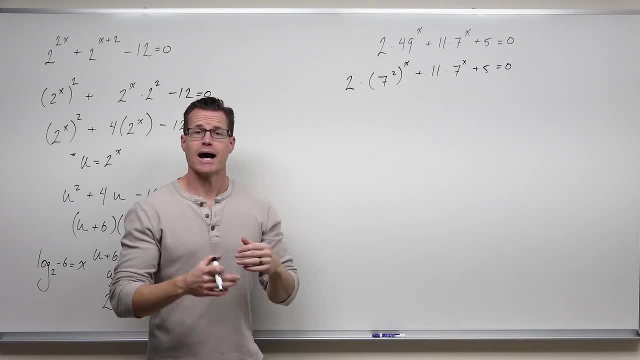 Why? Well, because that's seven to the X and that's seven to the second. I need them to be the same. But take a look at what happens if I have seven to the second power, to the X power, I can multiply that two times X. 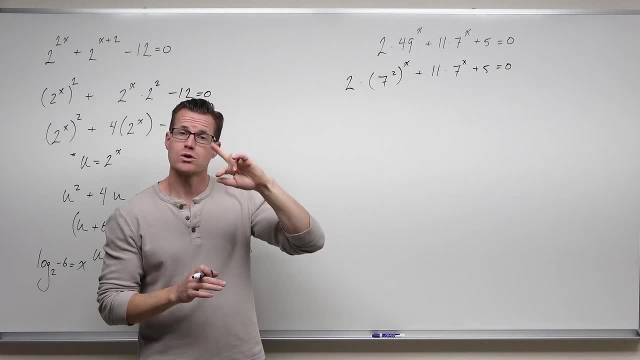 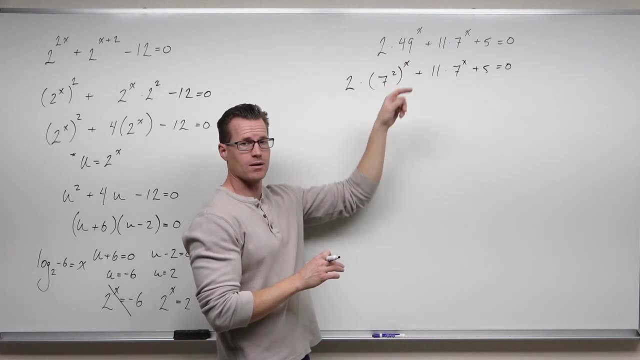 But wait a minute. two times X means the same thing as X times two, So could I just reverse those? Keep this in mind: If two times X is two X, then if I put an X here and a two there, that would still be two X. 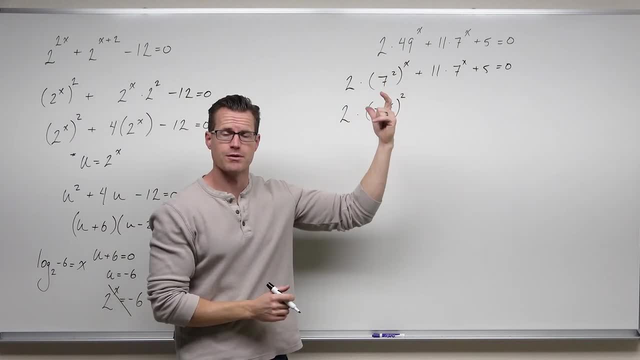 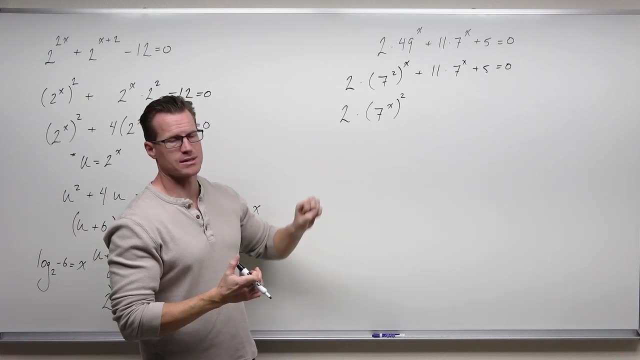 I'm really hoping that you see that. because multiplication is commutative, you can have those two exponents in whatever order you want, and they still make forty nine to the X. Honestly, they still make the same thing. So whether I have seven to the X squared or seven squared to the X, it doesn't matter. 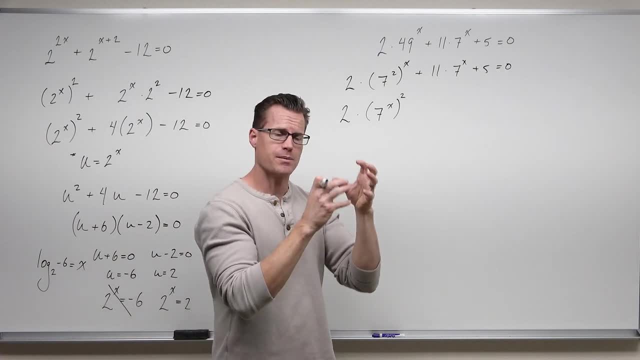 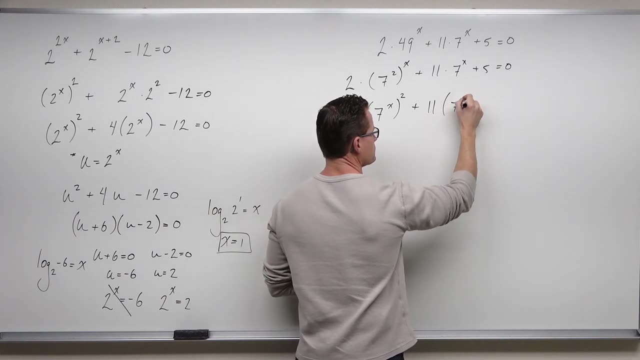 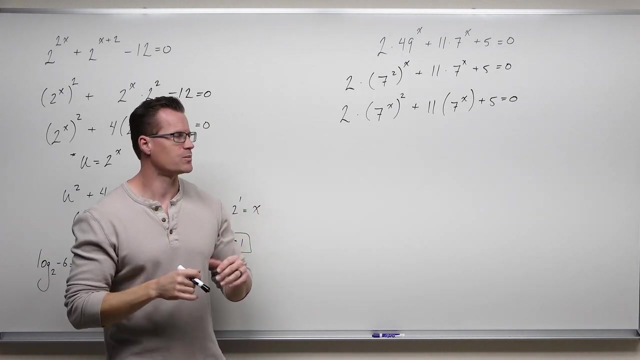 I'm going to choose this one because it fits what we're talking about. What I'm trying to do here is fits with the. I'm trying to match the exact same exponential in two terms of my equation. I also show those in parentheses to make my substitution a little bit more noticeable. 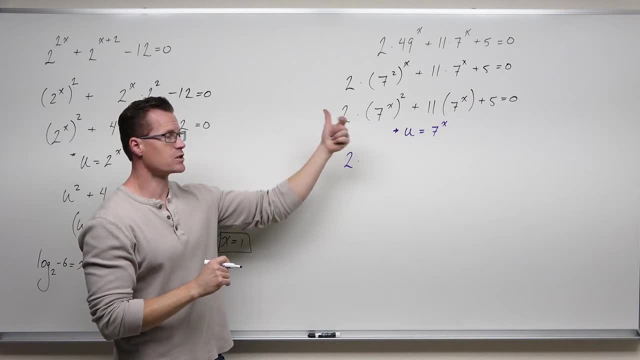 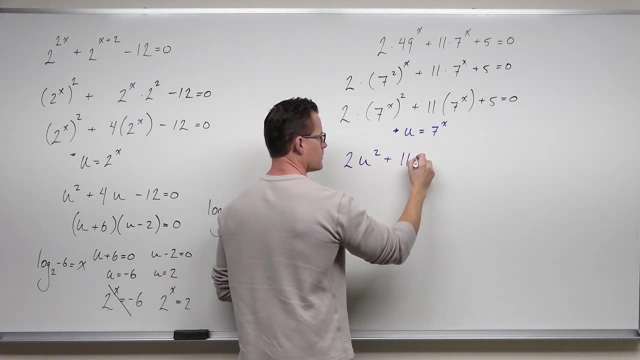 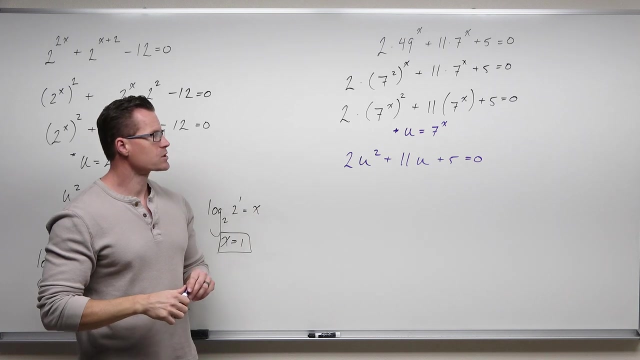 So if my, my seven to the X exponential is going to change into U, I've got two, and then this becomes U squared Eleven, U and then plus five. OK, so let's go ahead and factor that. It's going to be factorable almost all the time. 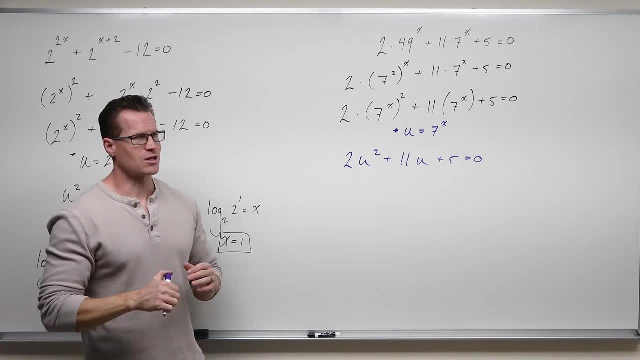 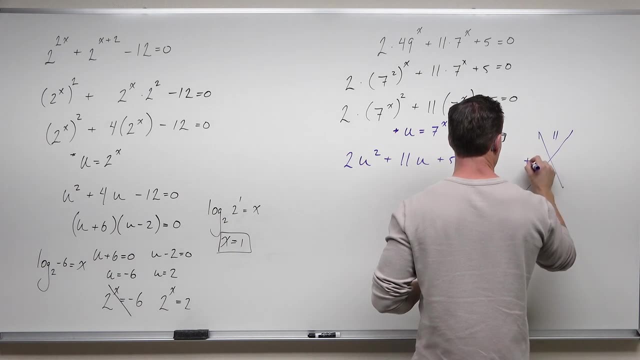 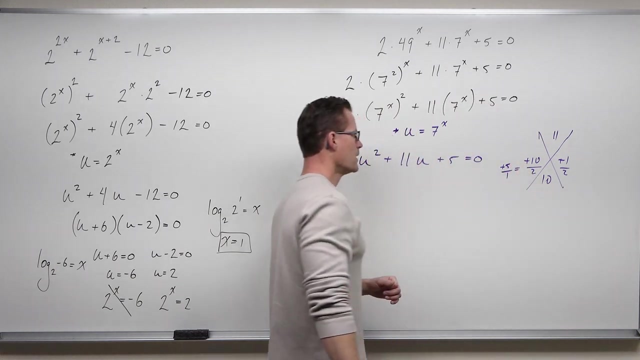 Just be careful. when they're not, You have to use a different technique. Check your factor media. It's probably factorable. So this is going to factor as common mistake. You're not in excess right now, You're in use. So when you factor you've got to use you. 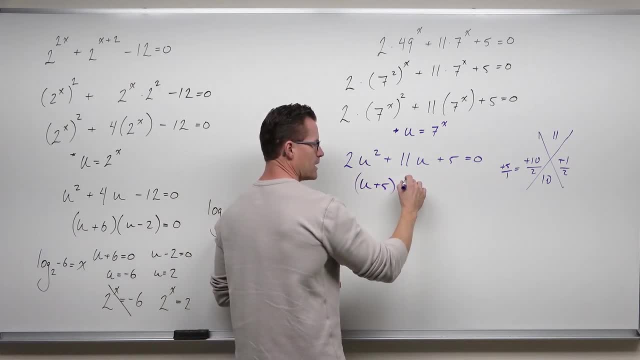 So we've got one U plus five. We've got two U plus one. We can double check this: That's two U squared plus U plus ten U, That's eleven U and then plus five. The zero product property is going to set each of these equal to zero. 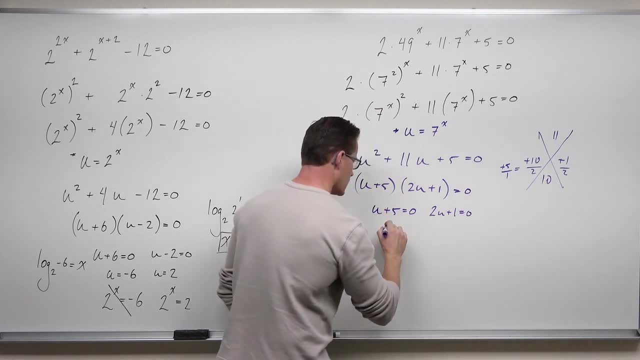 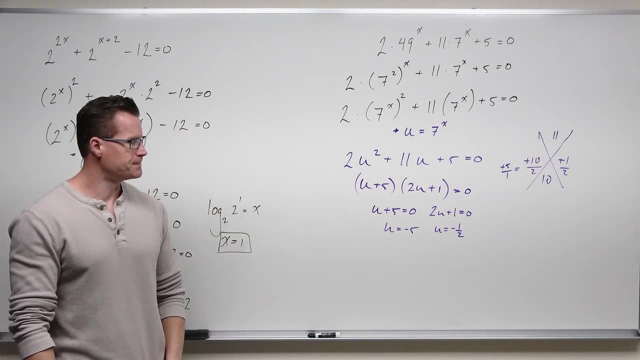 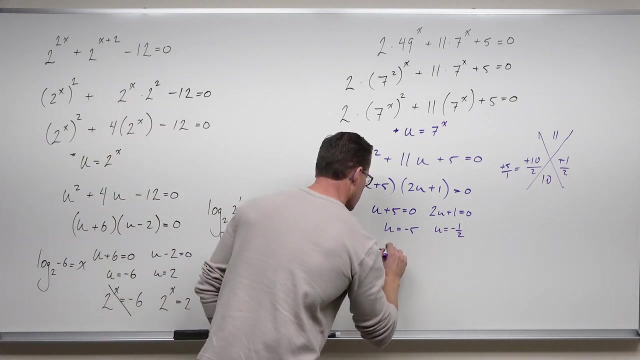 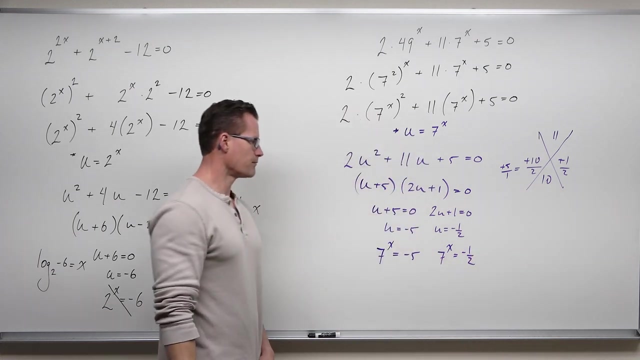 Right now looks just fine. On the next thing we're going to do. Hopefully you understand this is not so fun When we do this. right now we're going to look at this and go wait. hang on, I'm sorry. 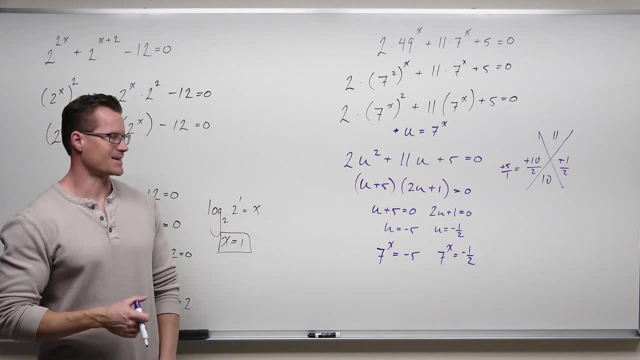 Right now We're going to look at this and go: wait, hang on, This is bad. Why? Why isn't it working? Why, Why, Why, Why? second, I've got two negative numbers here. Those cannot be solutions because exponentials cannot. 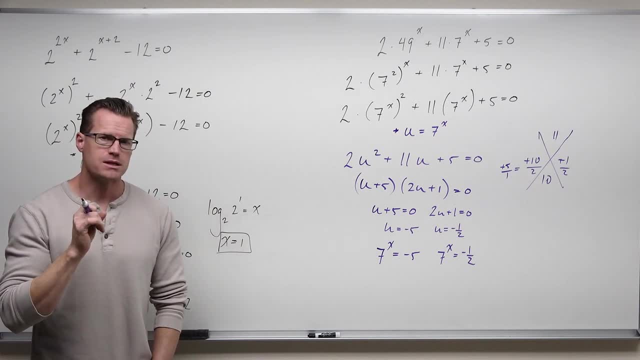 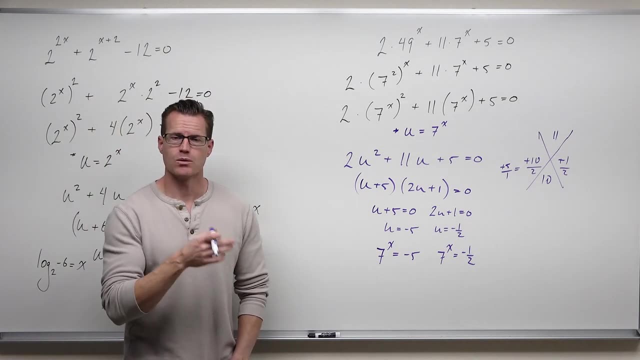 equal negatives. Now I'm going to make it real clear. This is not a domain issue for your exponential. You can plug in anything that you want. This is a range issue. This is saying: what can you plug in to get this output? You can't. There is a range issue. There's no way to. 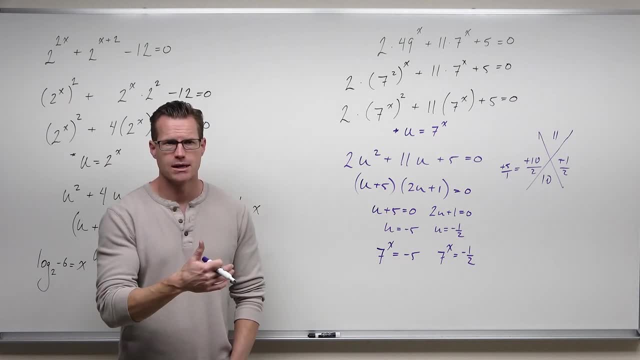 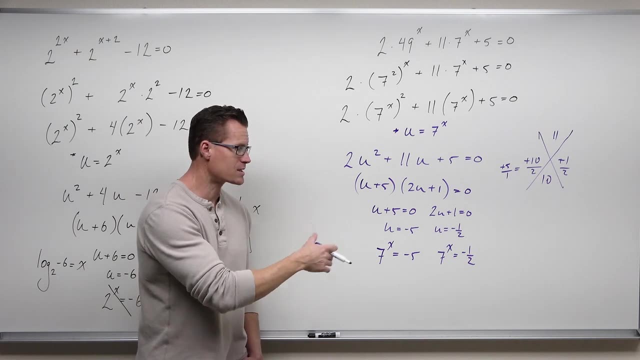 get out negative 5 and negative 1 half from 7 to the x. It becomes a domain issue for our logarithm. if we were to try to do it, We'd get log base 7 of negative 5 and log base 7 of negative 1 half. 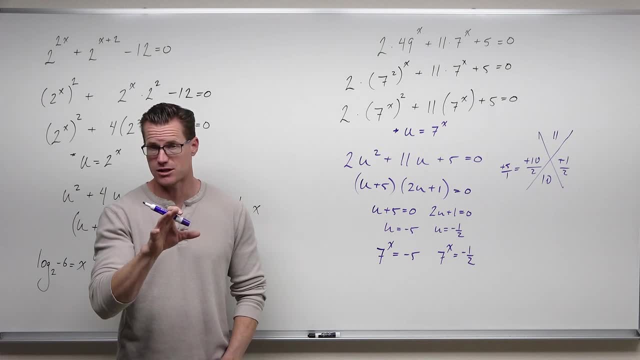 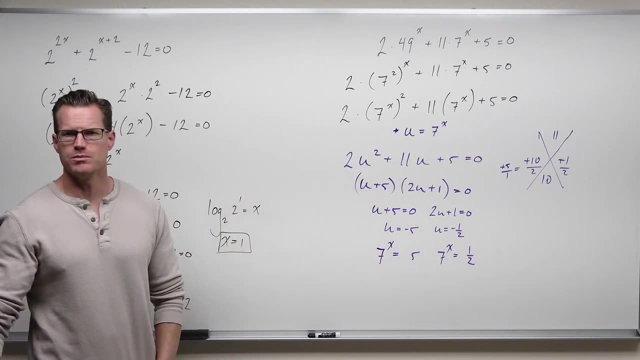 That's a domain issue because it came from a range issue of an exponential. I hope that makes sense. If we would have had positive- now we don't, I know we don't, But if we would have had positive, then you'd be just fine. You can say: all right, this would be. 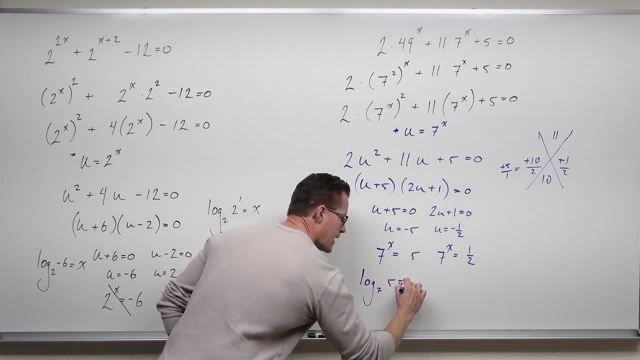 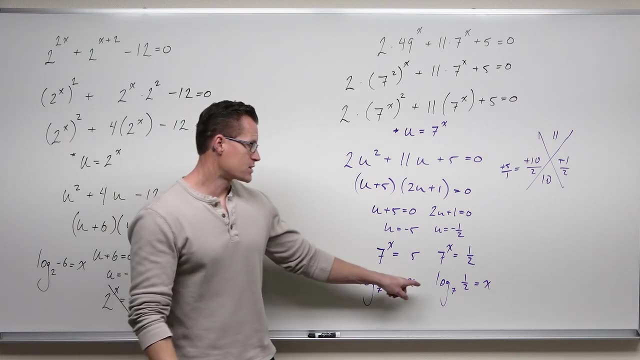 log base 7 of 5, log base 7 of 1: half equals x. Please listen, This will give you a negative. That would be fine to get a negative out, but you can't have a negative inside your logarithm. That would be plugging in a negative for your exponential. That's okay. 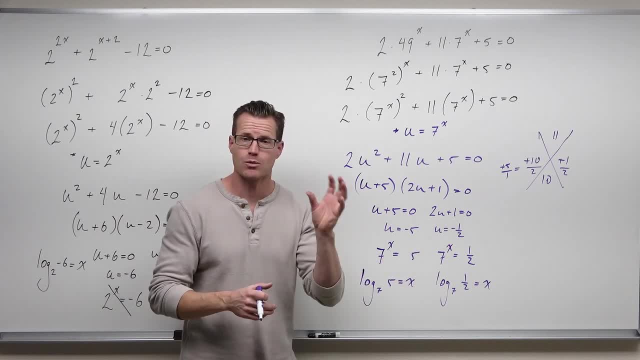 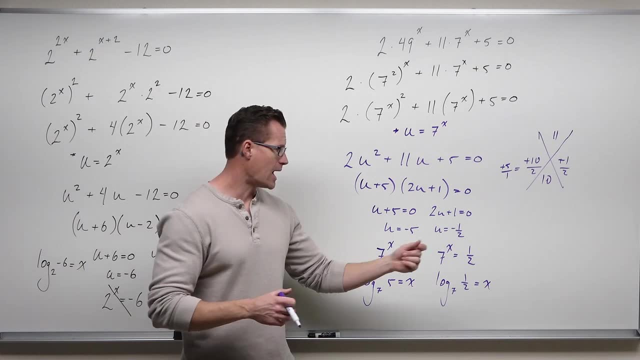 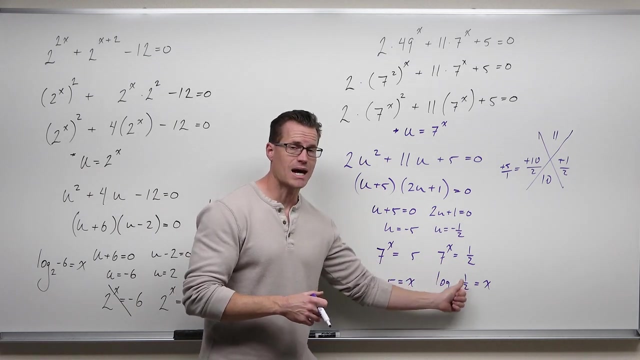 You can plug in a negative here. That'd be fine to plug in a negative, but it can't get anyone out. So what you can't get out of an exponential is what you can't plug in to a logarithm. I can plug in negatives, I can't get out negatives. I can't plug in negatives, I can get out negatives. 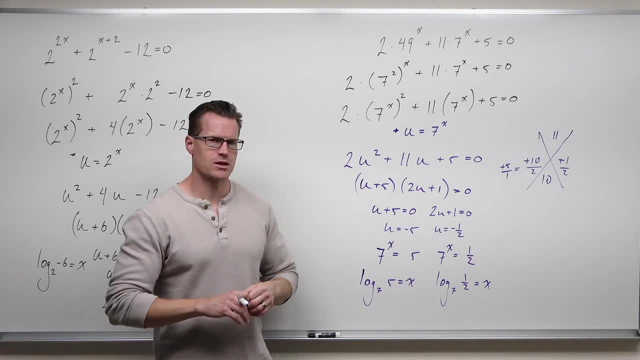 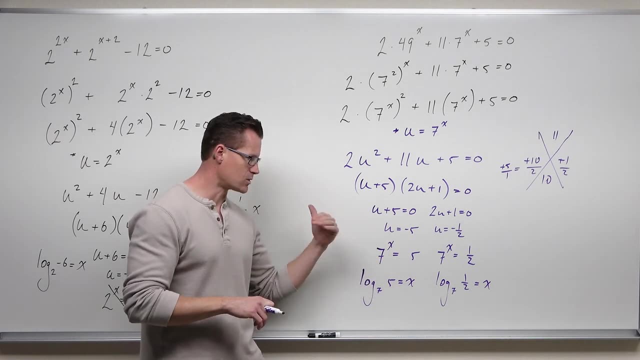 would be our two solutions if these had been positive. I just want to show that to you to make sure that we saw that one more time. You could show it differently, of course. You could do a log of base 7 of both sides and ln of both sides, move your exponent divide A log base 10. 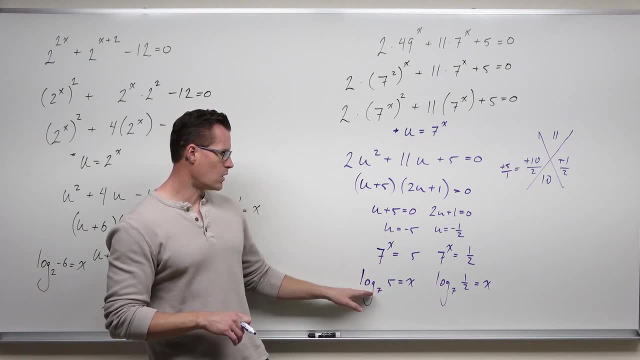 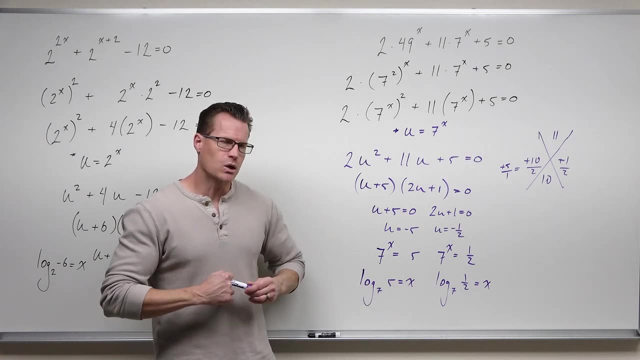 of both sides, move your exponent divide. You could also change your base and get log of 5 for log of 7, or ln 5 over ln 7, same thing over there- and get a different look so that you can approximate it a little bit easier. But that's where I'm going to end on these. problems is 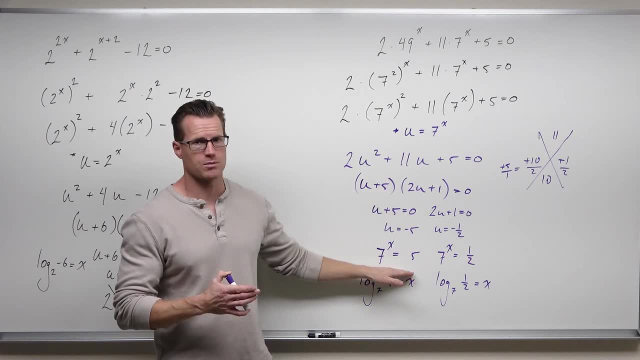 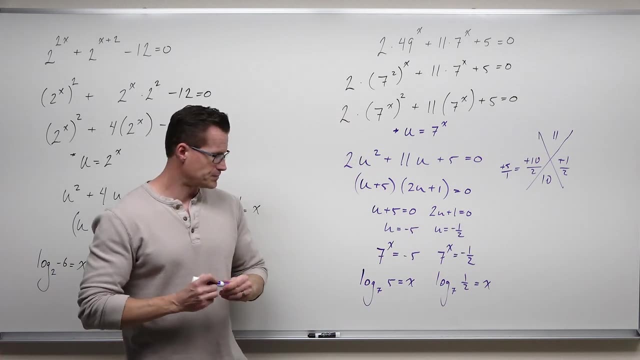 this idea. Once you get down to here- this is something we've talked about already- You cannot let them equal negatives. In this case, you have no solution. It's not possible to do Okay. I felt bad that I gave you one with no solution. Feels like you didn't get what you. 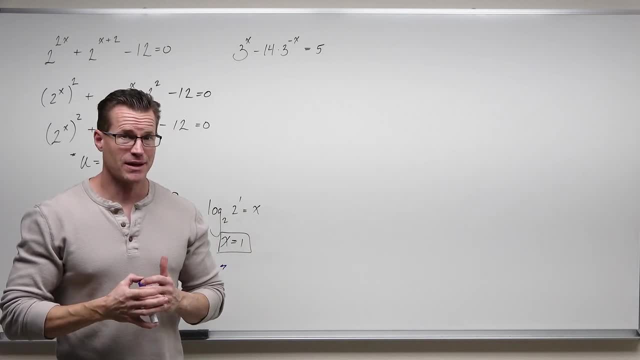 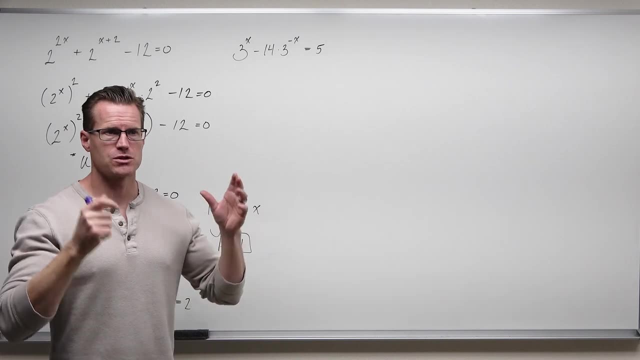 paid for, even though for most of you this is absolutely free. So I'm going to give you one more because I feel like it and I can. So sometimes these negative exponents just go what? And I'm stuck and I don't know what to do. 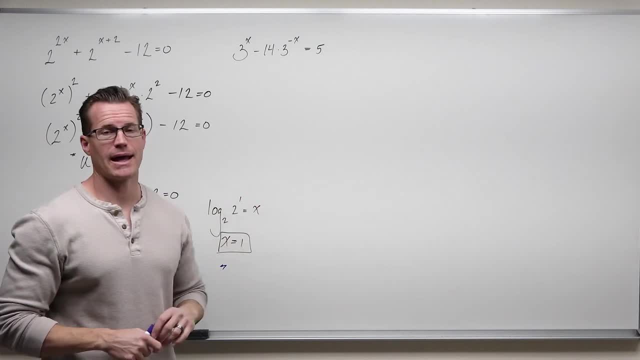 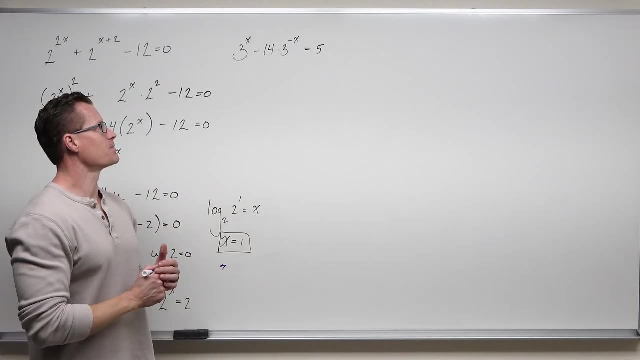 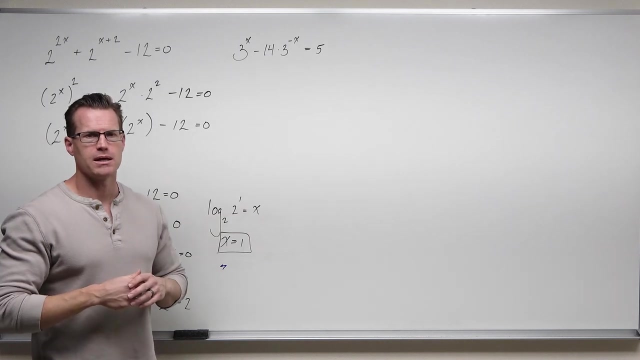 And I wanted to show how to do that and that you can get one solution out of these. At least this one does. So let's take a look at that. 3 to the x minus 14 times 3 to the negative x equals 5.. Firstly, classify or qualify it. Where does it fit? Is this one exponential? 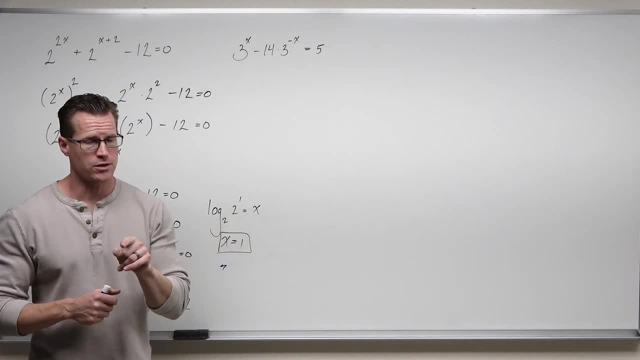 No, Can I combine those? No, not with subtraction. Do not try, You can't do it. Okay, can I get one exponential on one side and one on the other side without a constant Common basis? No, because the 5 messes it up and so does the minus 14.. Can I get one exponential? 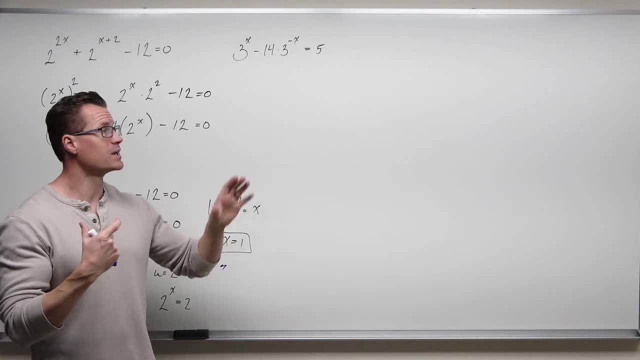 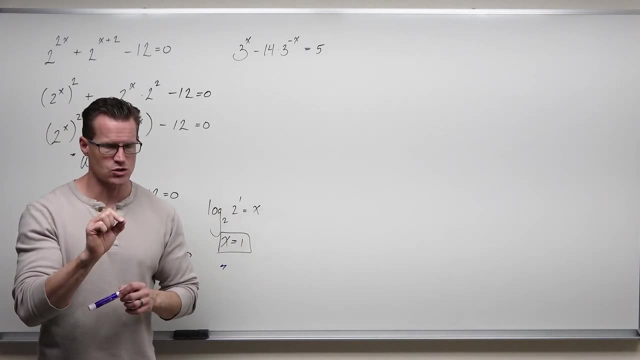 on one side and one on the other side, with different bases, and use a logarithm. No, because for the same reason, This is another substitution, but you have to set it up correctly. We must get the same exponential in order to substitute it and we have to have it in two. 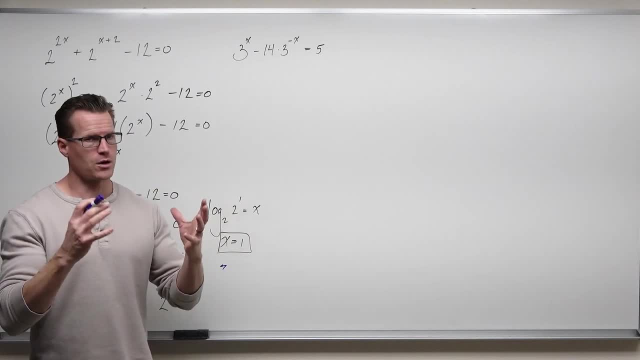 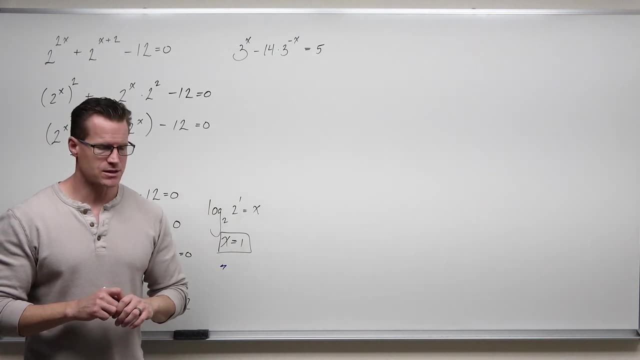 terms. So what are we going to do For our techniques to work? by the way, what are we going to do If you see a negative exponent? there's two choices, and this is what your textbook should say. If you see a negative exponent, there's two choices, and this is what your textbook should say. 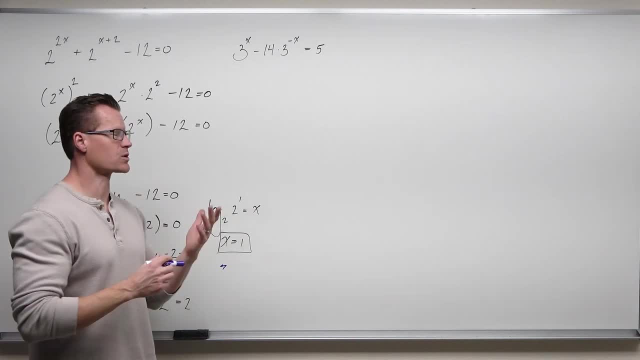 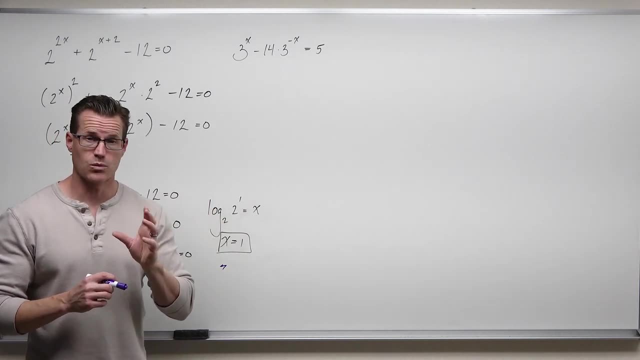 Multiply by x to the positive 1.. Oh, sorry, I said that wrong. Multiply by 3 to the positive x. You can do that on both sides, but it might be a little easier to see why you're doing that. And it's the same thing, but maybe write it a little differently so you see why you're. 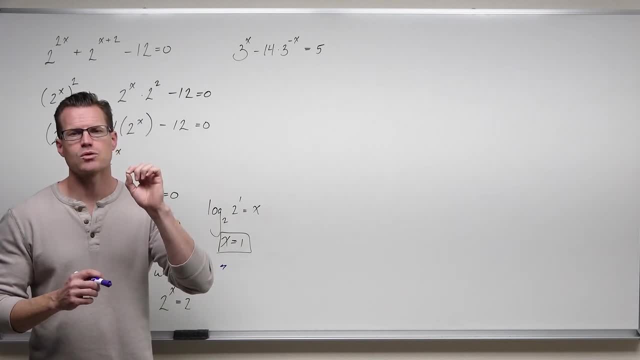 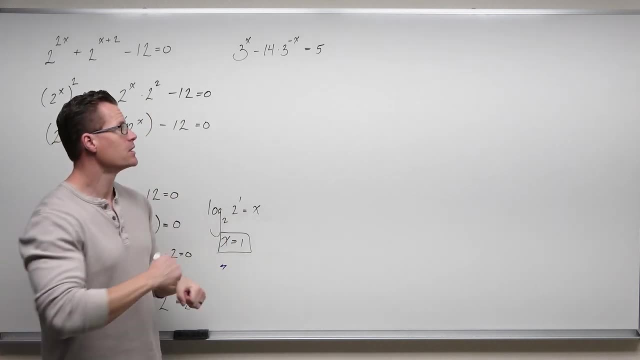 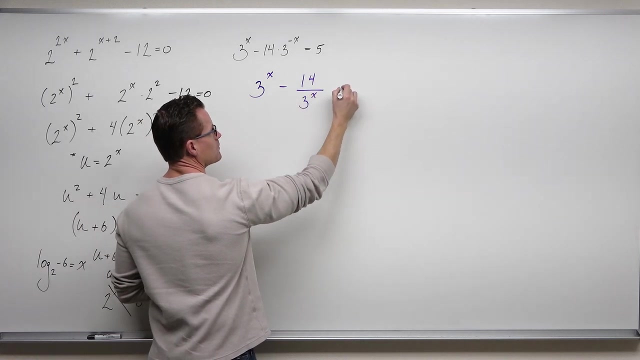 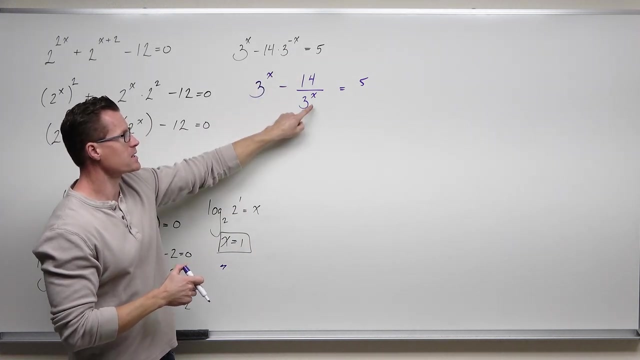 doing that, Remember that a negative exponent creates a fraction with whatever's being raised to that negative exponent on the denominator right where it's at. So this means This: This means 1 over 3 to the positive x. So 14 times 1 over 3 to the positive x. 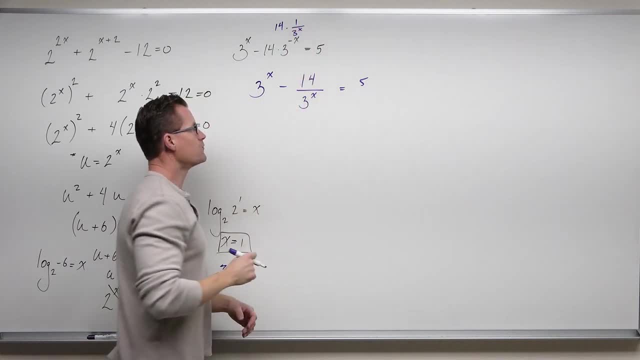 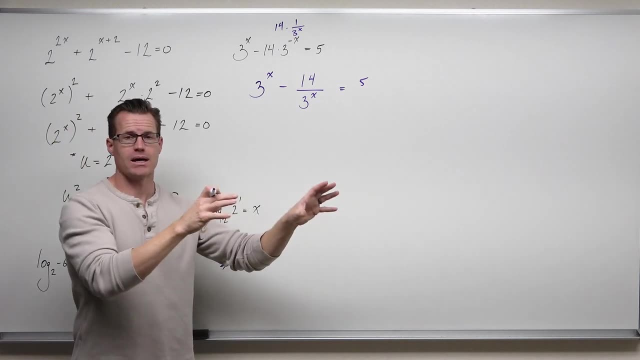 gives you 14 over 3 to the x. This is why they're telling you: multiply by 3 to the x. Why? Because this is now an equation that has fractions in it. How do you get refractions? You multiply by the LCD. 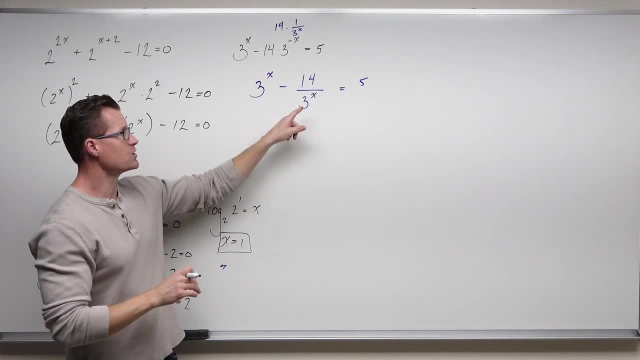 In this case that's just 3 to the x. Now do we have a domain issue by having that on the denominator? No, because 3 to the x can't even equal 0.. Oh, as far as I'll ask you. 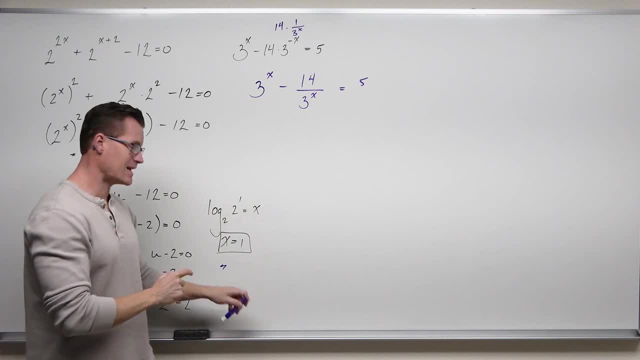 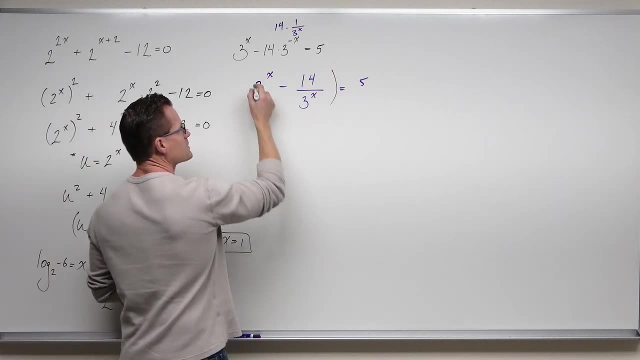 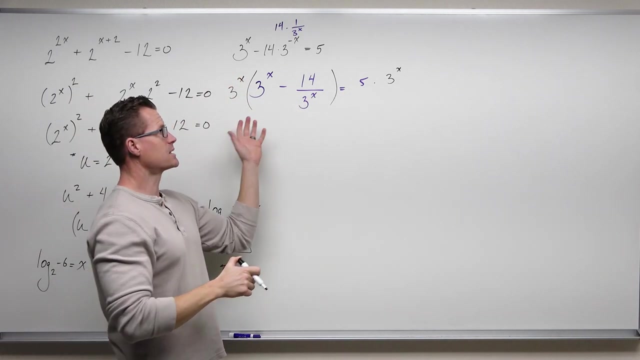 can't even equal that. So there is no problem. All we've got to do is understand that. in either case, what we want to multiply by is something that makes that negative go away. Well, that's going to be 3 to the x. Now, keep this in mind. It's got to be on both. 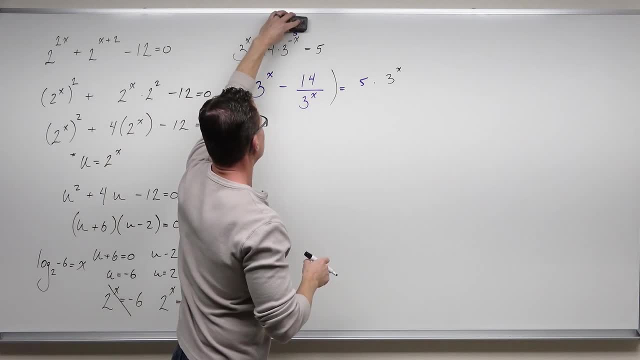 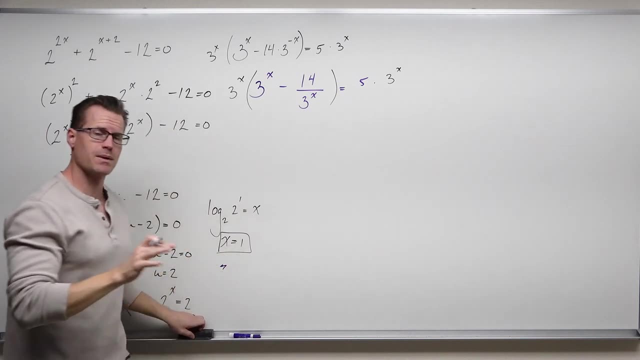 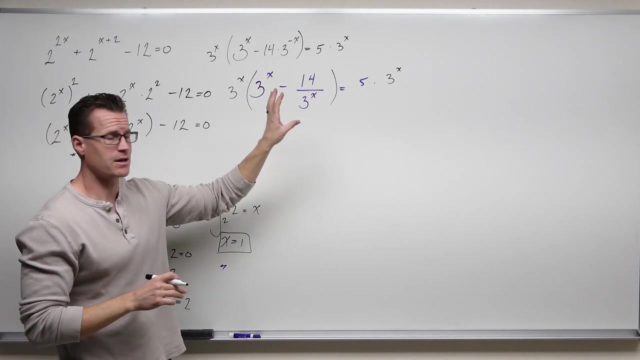 sides. Whether you do it here Or here, it doesn't matter. It has to be on both sides, because you're multiplying an equation. So multiply both sides by whatever takes you to that negative exponent. That negative exponent means something on the denominator that needs to go away. In our case it's 3. 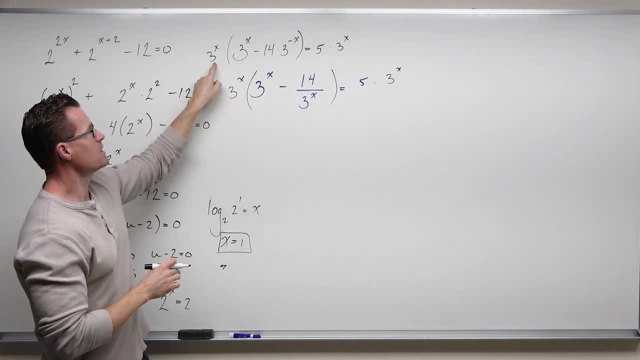 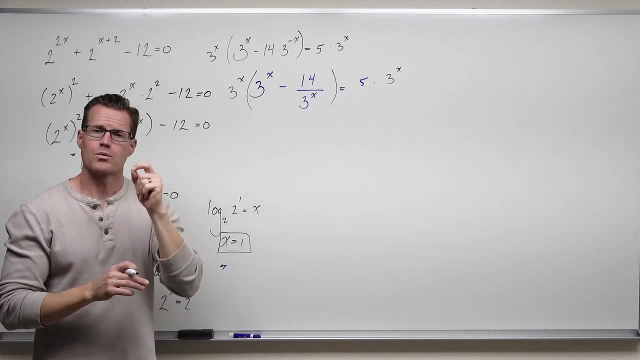 to the x. We're going to multiply and then distribute. If I distribute here, I'm going to get 3 to the x squared. Don't write 3 to the 2x. Don't add them. Write the 2x to the. 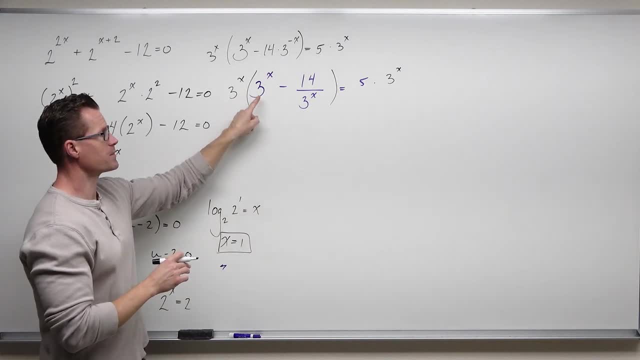 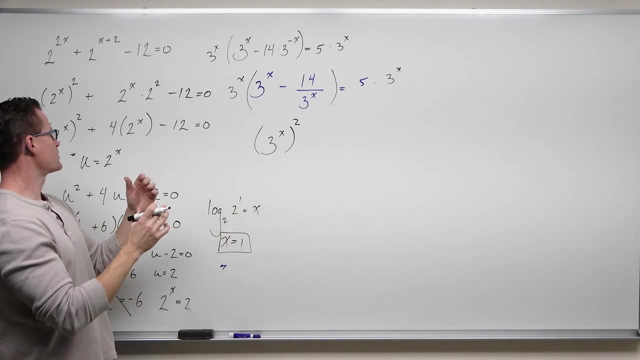 negative exponent. Write them as what you're going to need for the substitution. So 3 to the x times 3 to the x is 3 to the x squared. Could you write it as 3 to the 2x? Yes, but 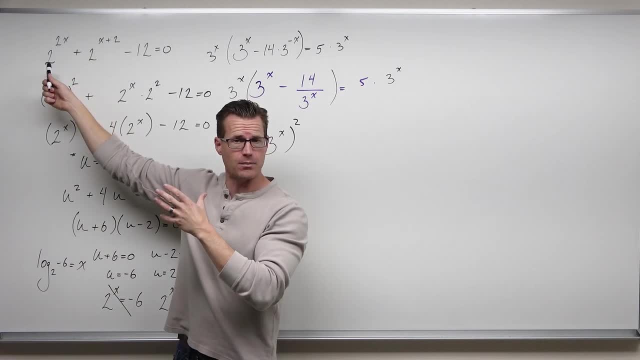 you're going to get exactly what we got here. That's where that came from. It came from 2 to the x times 2 to the x. That gave you 2 to the 2x, which we had to write as 2 to. 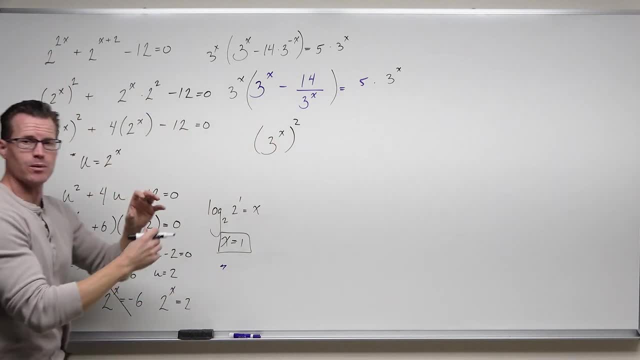 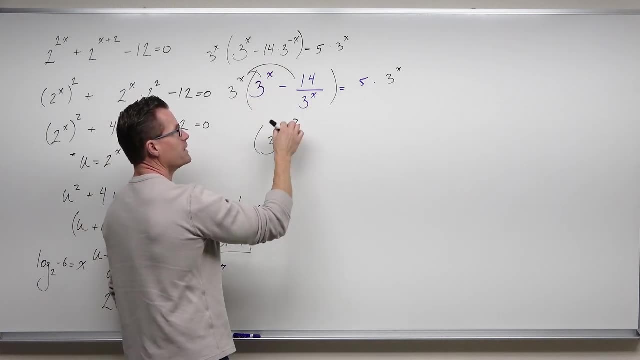 the x squared. So this is the same thing as that, but we've written it more appropriately for our substitution work. That gives you 3 to the x quantity squared. This, Your denominator, is going to cancel with that. So 3 to the x times 14 over 3 to. 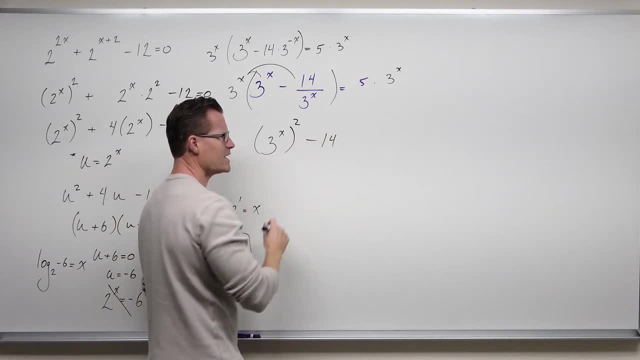 the x. You cancel that, You get minus 14.. You go, wait a minute, My substitutions work. Ah, it's tricky. That's why, on the other side of the equation, we had to multiply by 5 times 3 to the x. There's your other term, with your 3 to the x in it. So we're going to get everything. 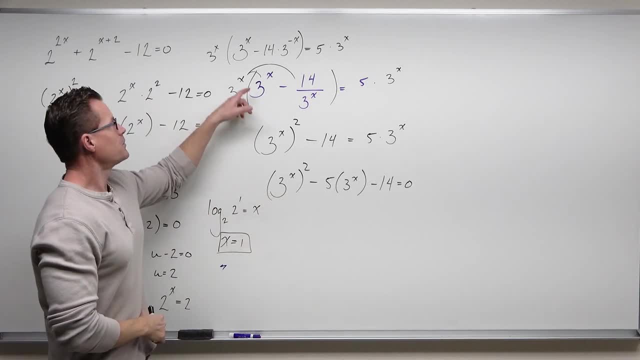 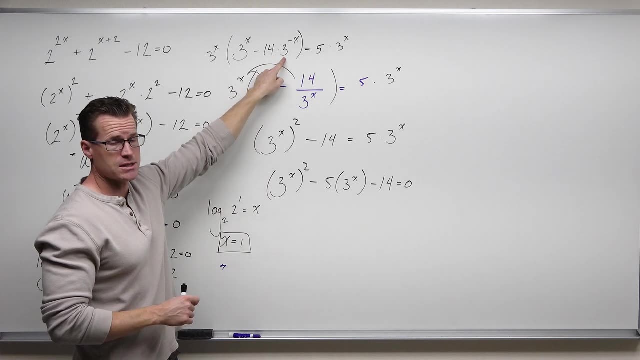 on one side, because we're going to substitute and then factor. Please notice that doing it right here is the same thing. You get 3 to the x squared. You get minus 14 times 3 to the negative, x times 3 to the positive x, Negative x. I'll. 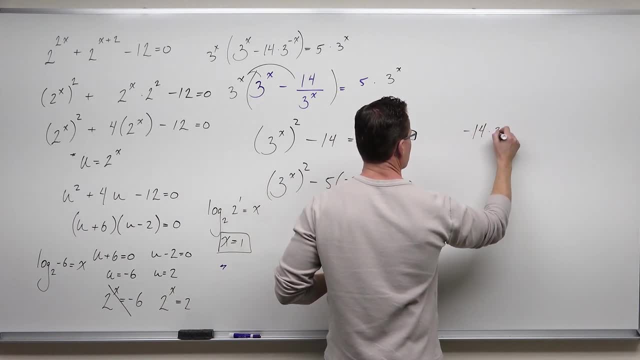 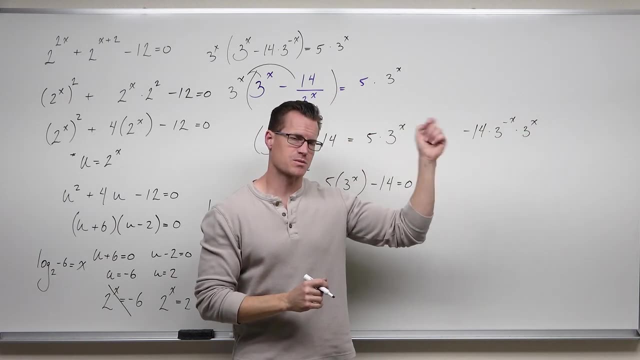 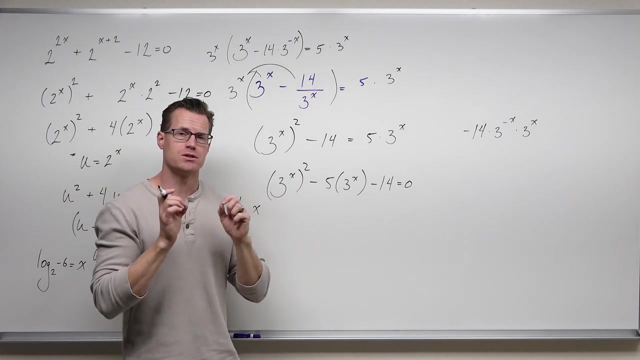 show it: Multiplying common bases, you add your exponents Negative x times or plus. positive. x is 0.. 3 to the 0 is 1.. You just get negative 14 either way. Personally I think that's a little easier to see, but they do work the same. Whichever one you feel confident. 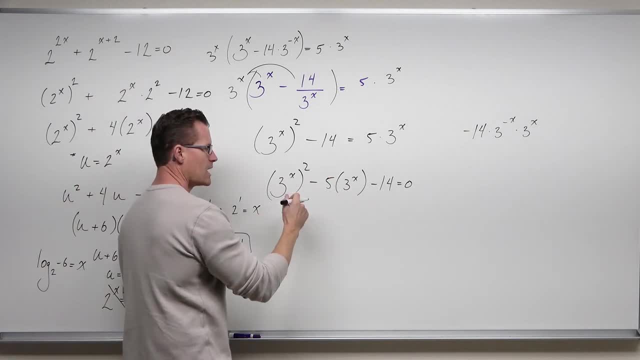 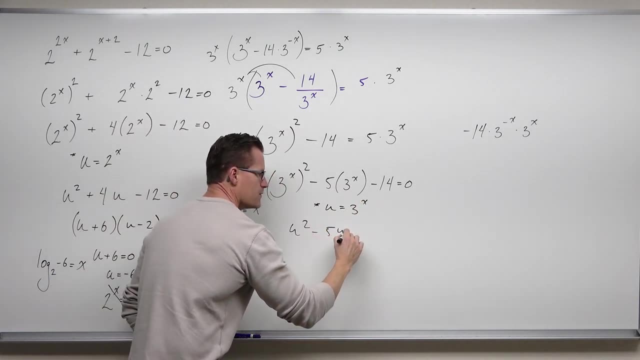 with. it's going to work perfectly for you. We're going to have a substitution available to us, That's 3 to the x, So we're going to substitute that and get u squared. minus 5u minus 14 equals 0. This factors pretty nicely. 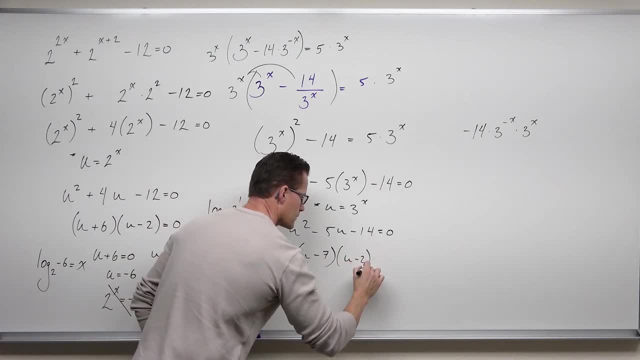 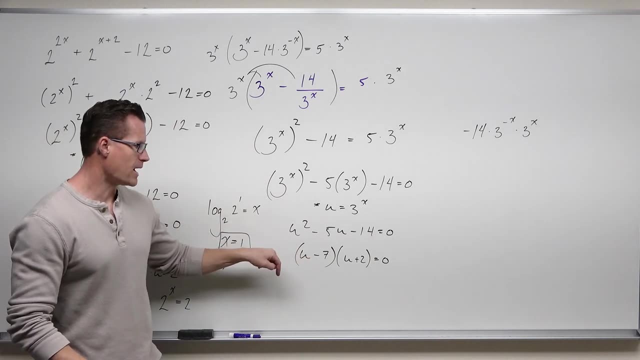 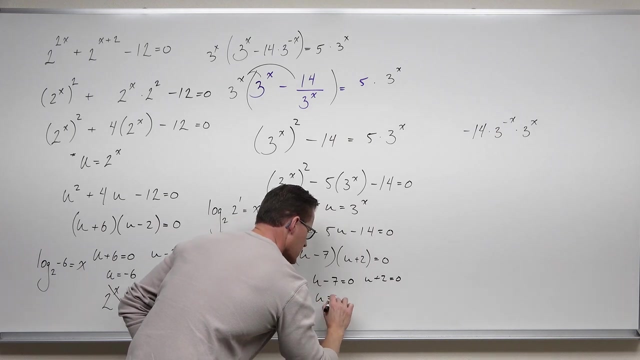 for us, If you do it right, u squared that would be minus 5u and minus 14.. Can you see which of these is going to give us a non-value? Is that a valid solution for real numbers? Hopefully, you say. I cannot allow an exponential. 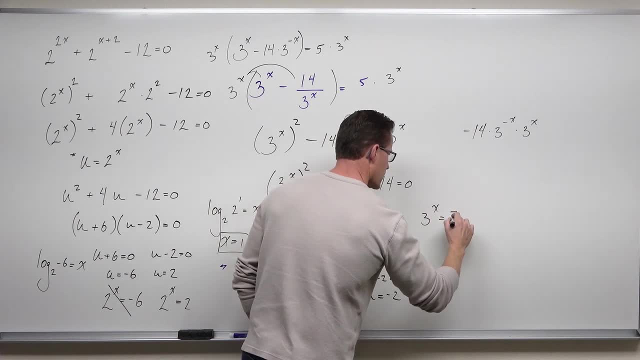 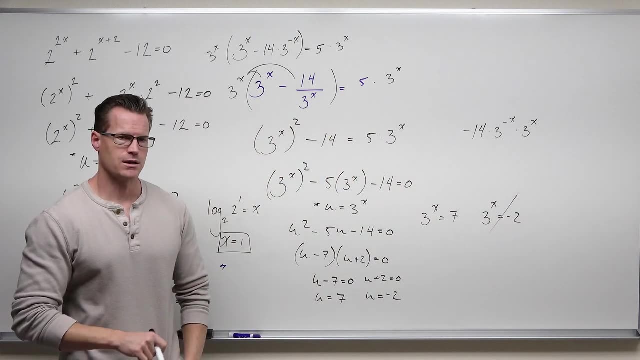 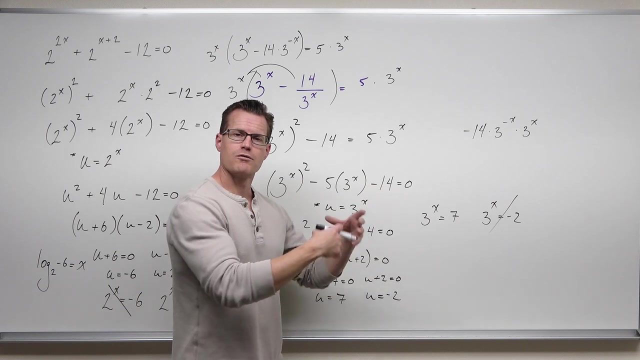 to equal a negative. That's off the table. Your exponentials can't give you a negative. It's a range issue. It becomes a domain issue for a logarithm that we would need to solve that. This, however, looks really good, So I do a log of both sides: Move my x and divide. 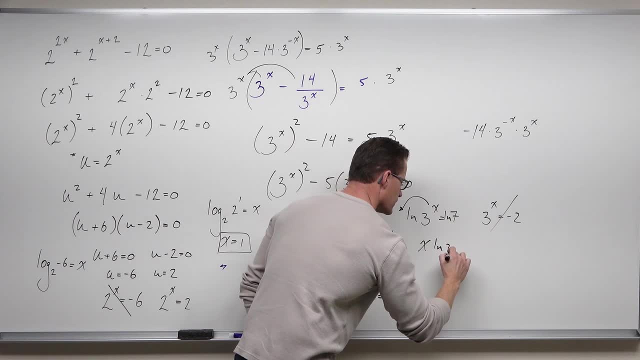 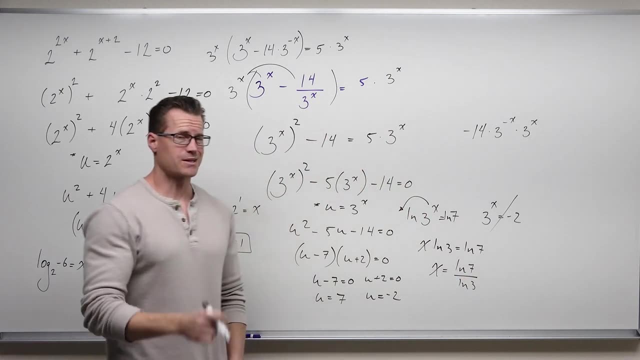 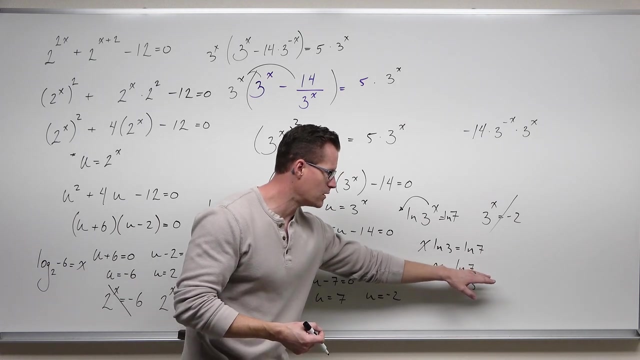 the front. That's one option that's very easy to approximate. Another option: use log base 10.. You get log of 7 over log of 3.. Very easy to approximate Or make it more concise From here. you can do a change of base and pick the base of 3 and an argument of 7 in. 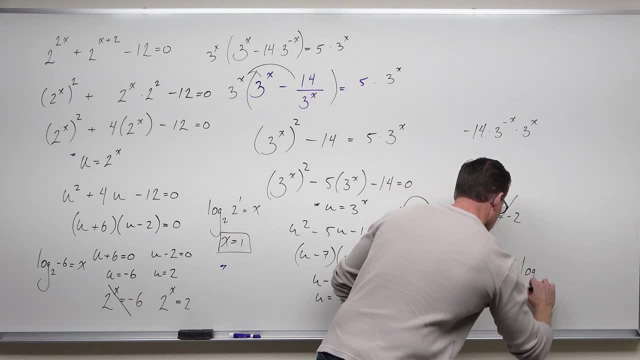 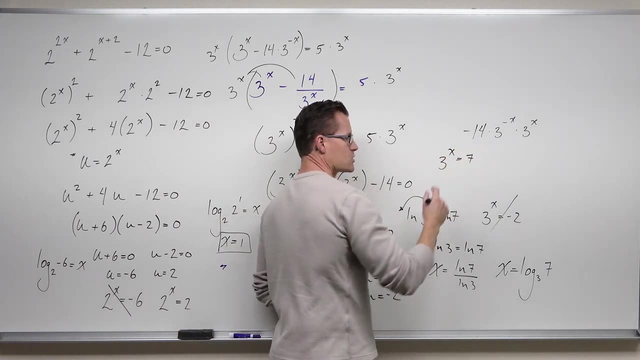 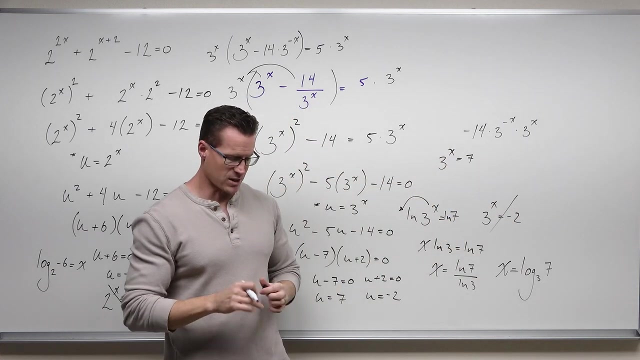 a new logarithm And that's exactly what we get. if we went directly from our exponential to a logarithm, You say: hey, here's my base, here's my exponent. Log base 3 of 7 would equal x, because a logarithm separates base from exponent. Either one. 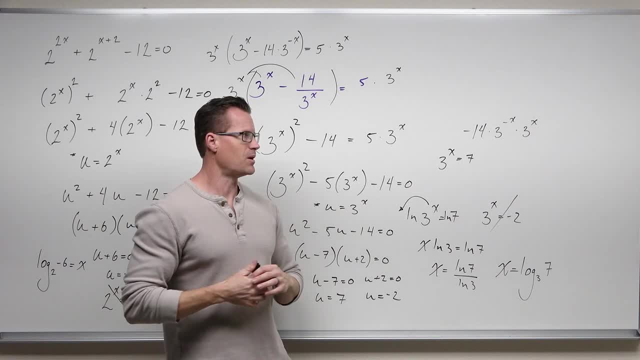 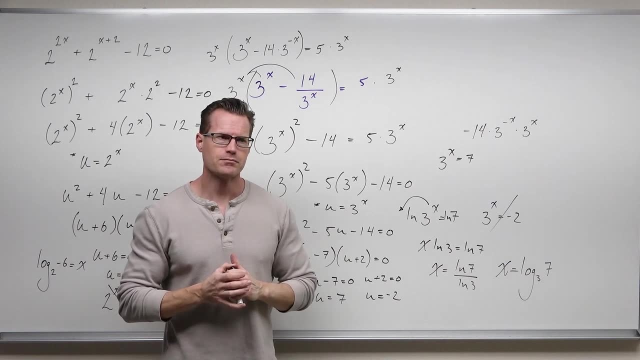 of those is going to work just fine. I hope that this has made sense. I've gone above and beyond, I think, as far as our our examples here. I've shown you every case I could think of to solve an exponential. So I hope that you're with. 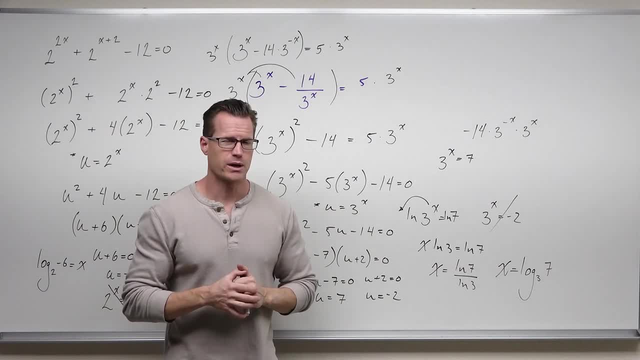 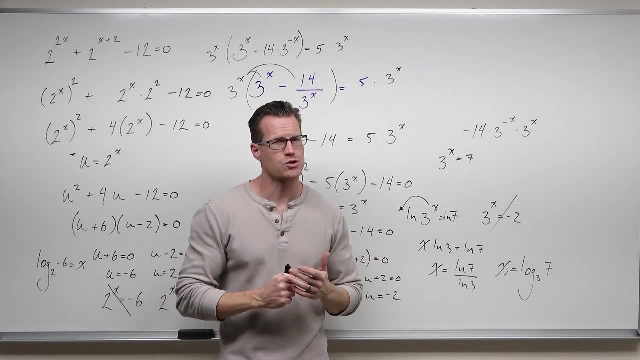 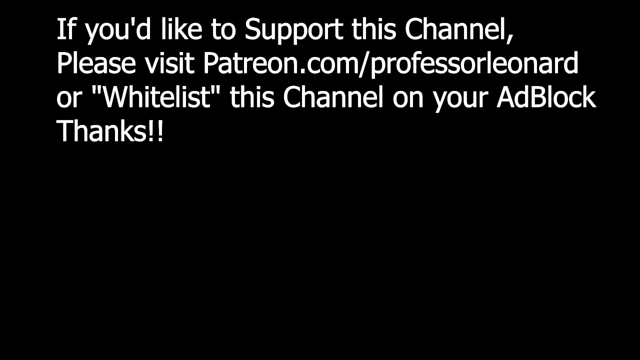 me Moving forward. we're basically done with what I need you to know with exponentials. We're going to go on to how to use them in some real life scenarios, like finance and like differential equations, but only as an introduction to exponential growth and decay. So I'll see you for those videos and I hope you do well. you. 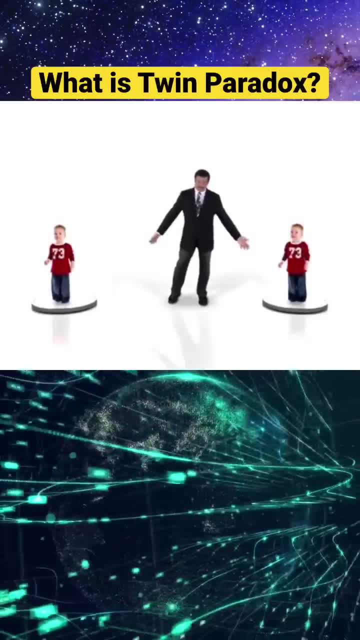 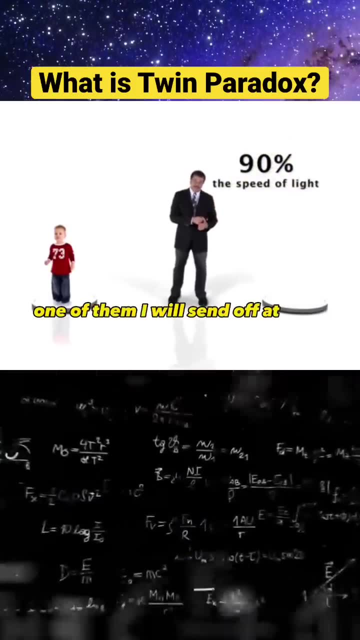 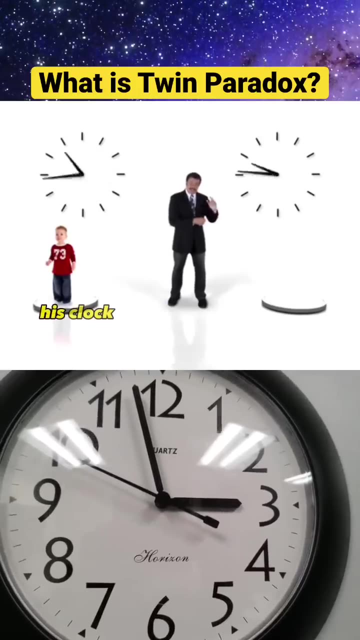 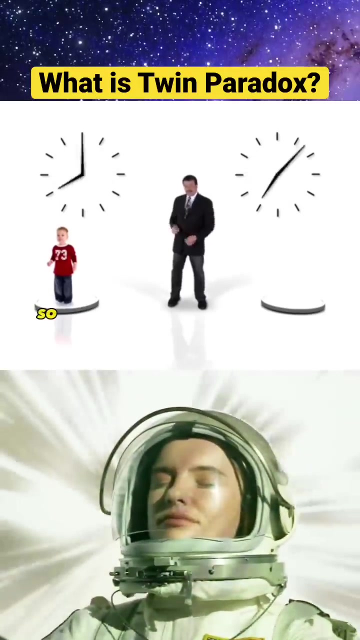 So here's how it works. Let me get a pair of twins, All right, And now one of them I will send off at 90% the speed of light, And the other I'll keep down here on Earth. Turns out this twin that I've already sent. his clock ticks 44% as fast as this twin's clock, So this twin is aging more slowly than this one. How about 99%? 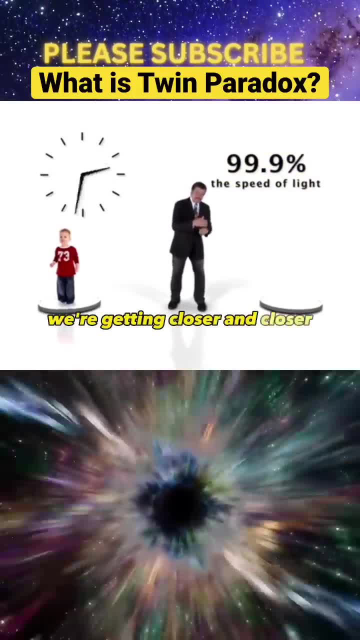 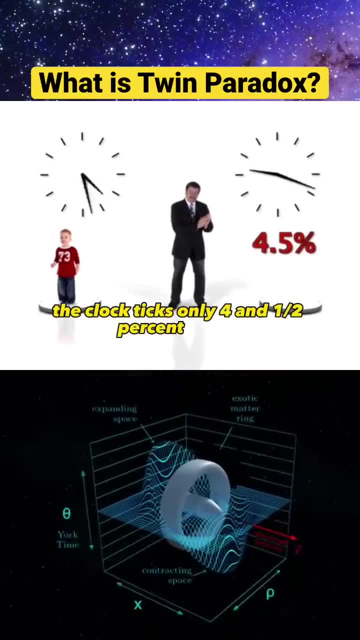 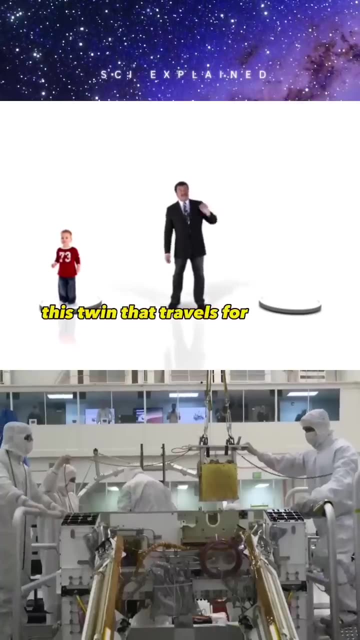 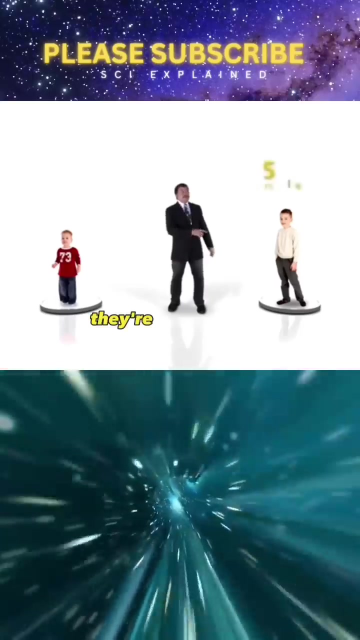 99.9%. We're getting closer and closer to the speed of light itself, And at that speed the clock ticks only four and a half percent as fast. So what does this mean? Tell you what it means: This twin that travels for five years and comes back. if they went at 99.9% the speed of light after five years, they're five years older, We have aged 110 years.